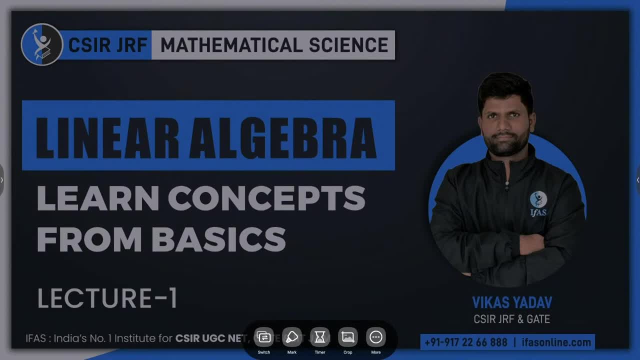 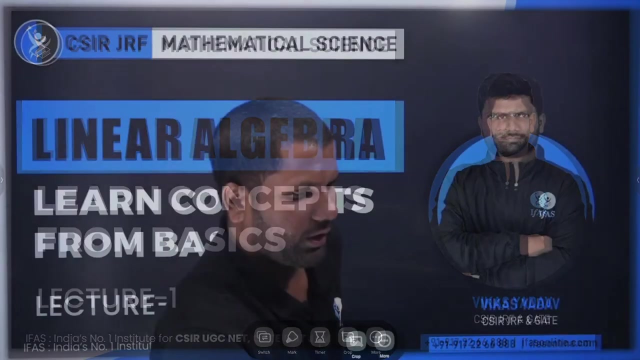 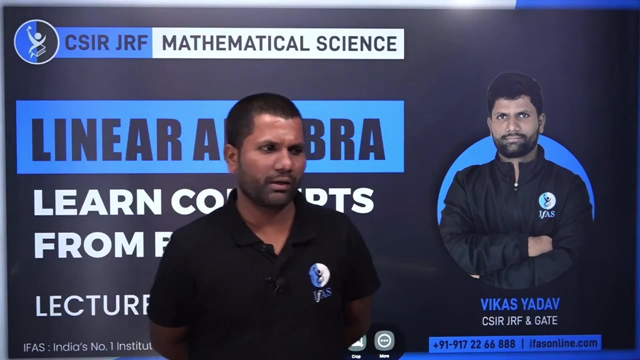 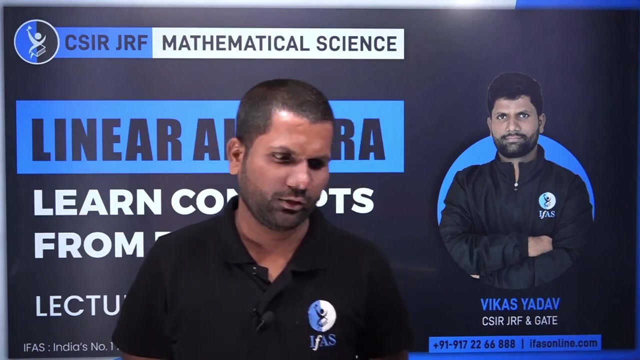 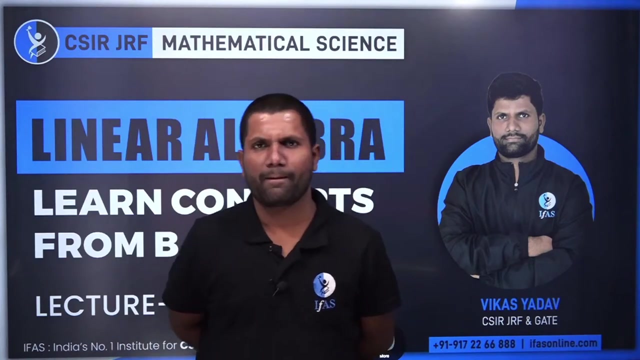 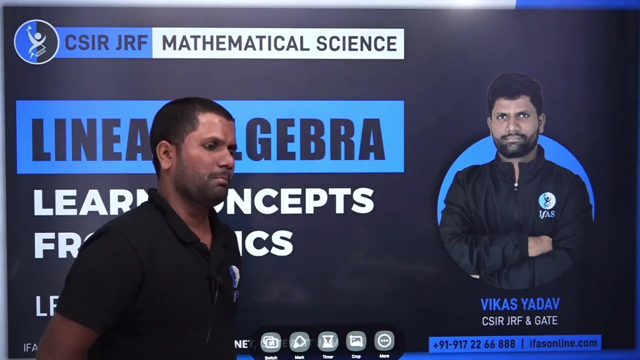 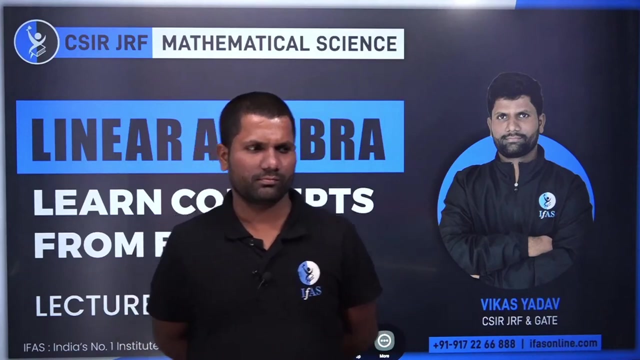 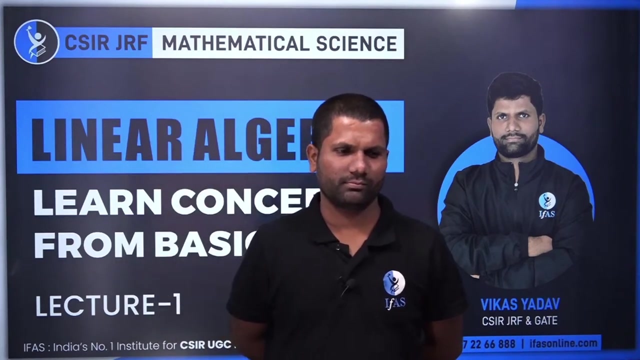 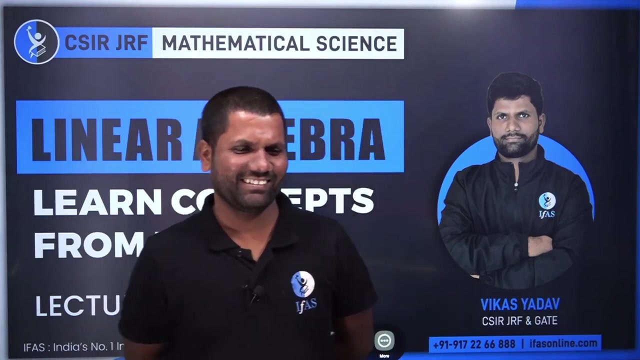 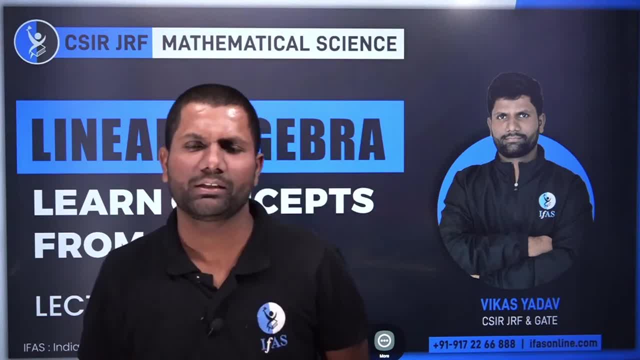 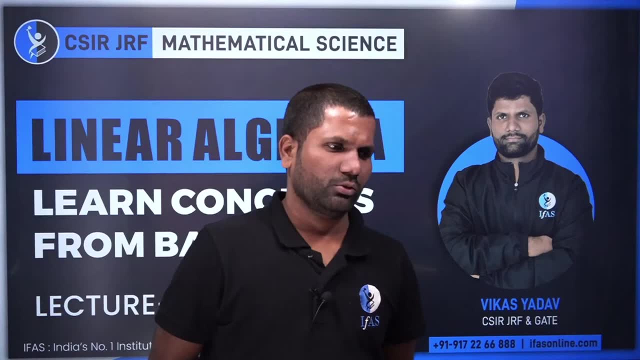 hona to chahiye kaize se dekhe December mein to. agar December mein nahi hoga to phir January aur February mein to hoga, hi hoga. good morning aunty, ma, good morning Irshad. so I hope NET WALA EXAM ap loge pehle thik thak gaya hoga. 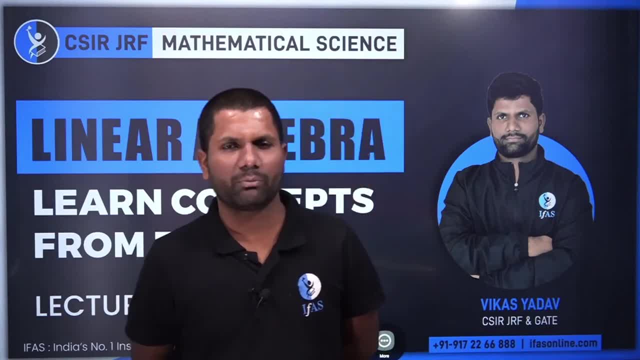 agar thik thak nahi gaya, koi baat nahi. ek baar phir se, 2-4 mahine baad apko phir se chance milega, 4-5 mahine ke baad, to waha par ap loge apna 100% dee jayega. 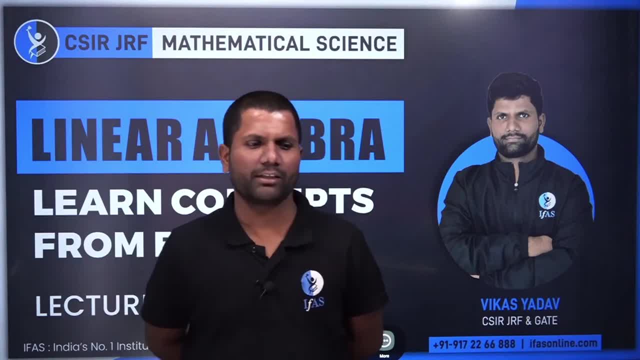 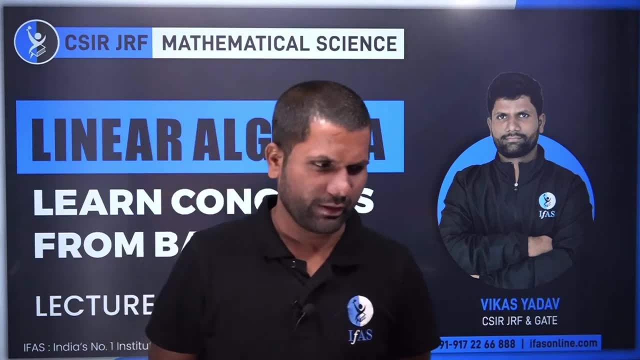 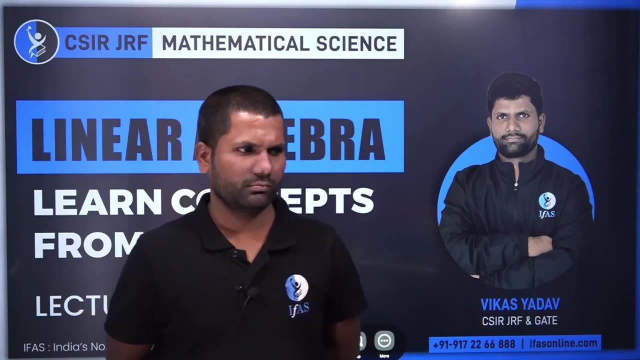 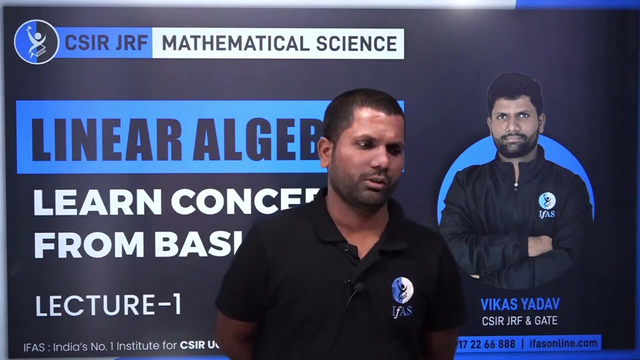 theek hai, bas aap apne tarah se koshis karo, baaki jo hoga, so hoga. good morning, sitar. theek hai to chala jaye aage, continue kiya jaye. theek hai to chali start karte aaj ke session to. 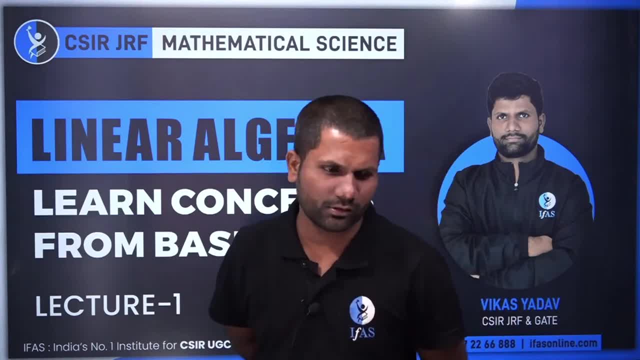 linear algebra. ek baar phir hum basic se start kar rahe hain. haan abhi to dekho Veerpal subah ke time to aapka linear chalega saam ke time 6 bajay saam ke sir. 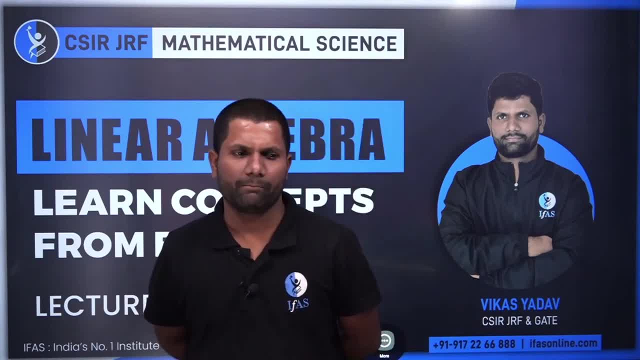 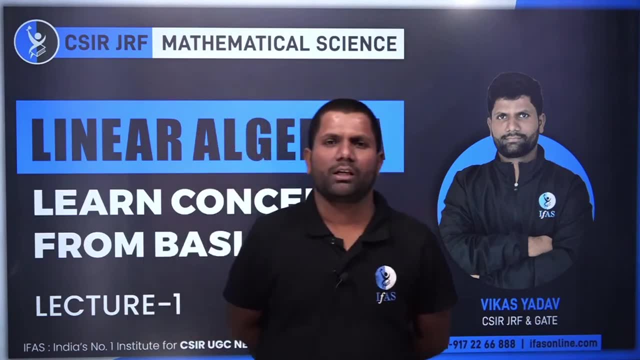 graph aapko bata rahe hain. graph bhi kaafi important hai. theek hai, haan param chalega. graph theory bhi kaafi important hai, ki jase ki aapko pata kuch chijey graph ya limits se. 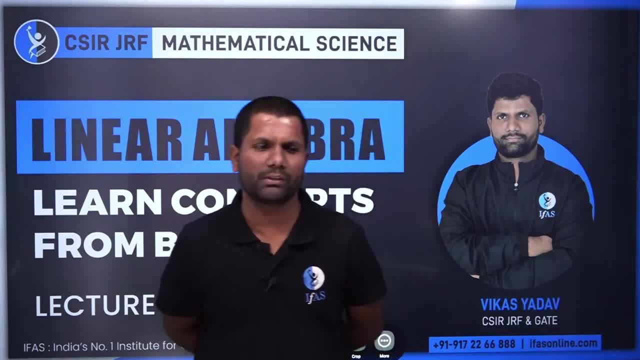 continuity limits, differentiability- kuch chijey aap graph se bhi bata sakte ho to graph agar baad hai aapko baad kare real padhne ke liye to kaafi important hai to uska ek session chal raha hai, saam 6 bajay se. 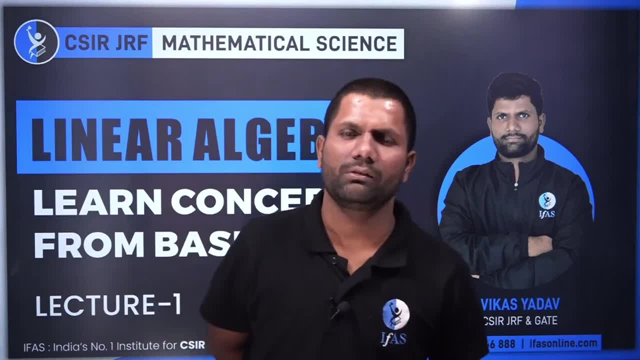 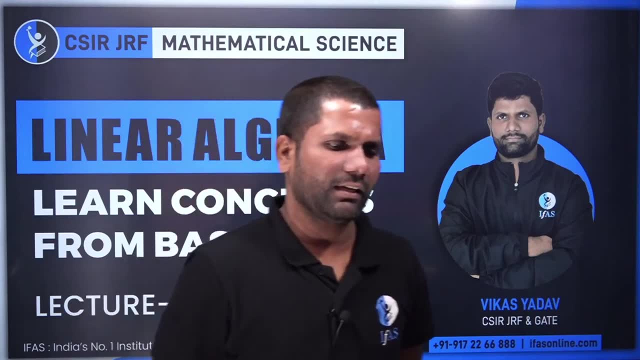 aur abhi aap log jo hamare sath jode subah. 11 bajay wala session. linear algebra ka rahega theek hai net ki answer ki to aa jana chahiye. answer ki jab aaya tabaar. response ki to. 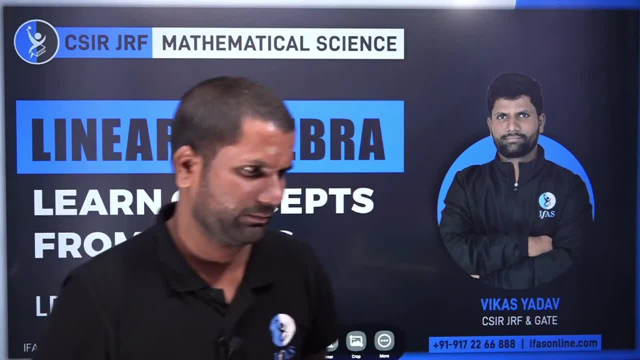 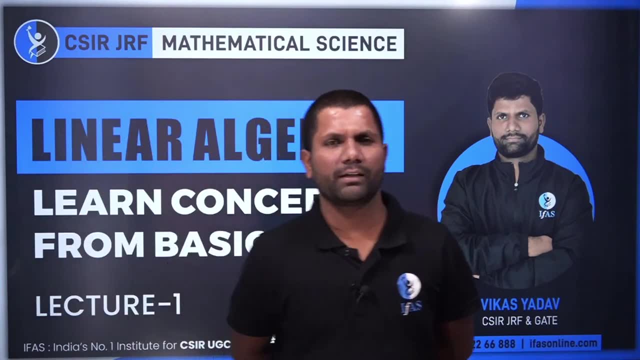 atleast mehne ke andar aa jana chahiye. theek hai. theek hai, agar dekho, vishnu, agar aap na basic se start kar rahe ho, aap kya kar sakte ho? saam series follow kar sakte ho. 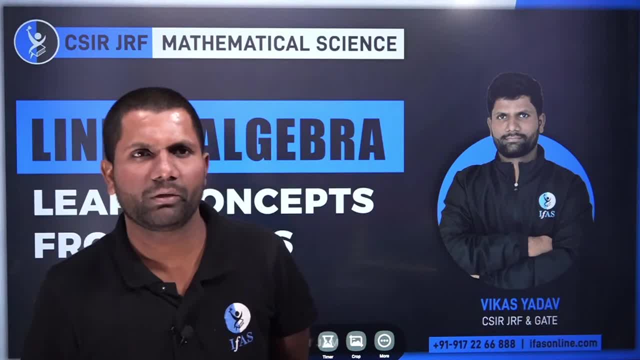 ya vikas vishta, vivek sahay ki book follow kar sakte ho of man and kunj hai isse aap follow kar sakte ho net exam point of view se dekhe to vikas vishta aur sahay wali. 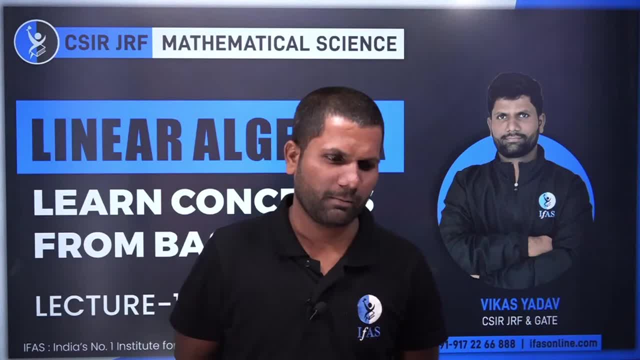 jo book hai o kaafi achi hai. net exam ke liye dekhe to theek hai linear, linear, complete karne ke liye astos pura linear. agar padhna hai to us case, me maan ki chali 80 ghante jate ha. 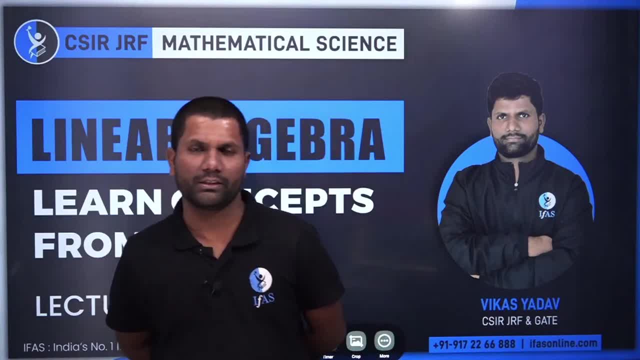 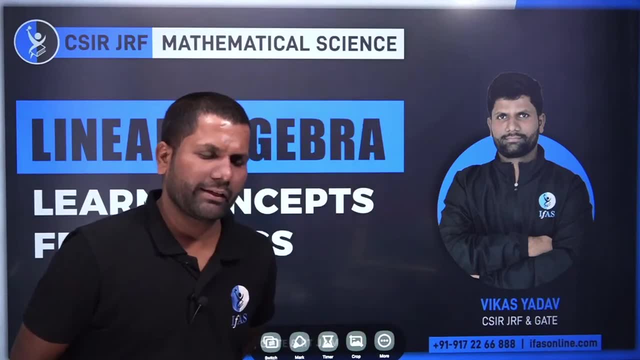 pura linear net ka syllabus padhne ke liye 80-90 ghante lagte hai. theek hai. good morning, priya pal. to chale start karte hamaar ek session aa jaye barte hai agli slide ki taraf. 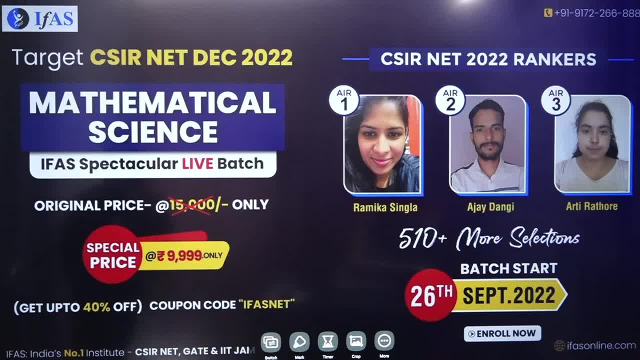 to yaha par ek baat aapko bata do ki yaha par 26 september se CSIR net ke liye naye batches launch ho rahe hai. to agar aap sabhi log hamare sath judna chahte hain, to is batch me. 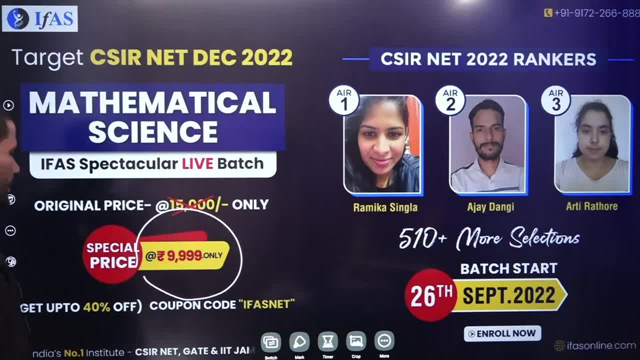 is price ke sath. aap log jud sakte ho. theek hai, yaha par aapko ek coupon code. yaha par diya gaya IFAS net to is coupon code ko dalne ke baat, the offer aapko mil jayega. 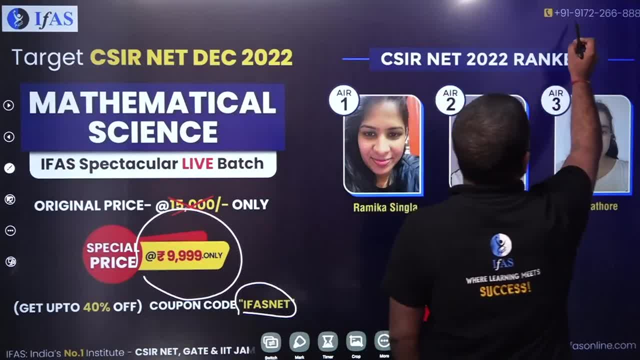 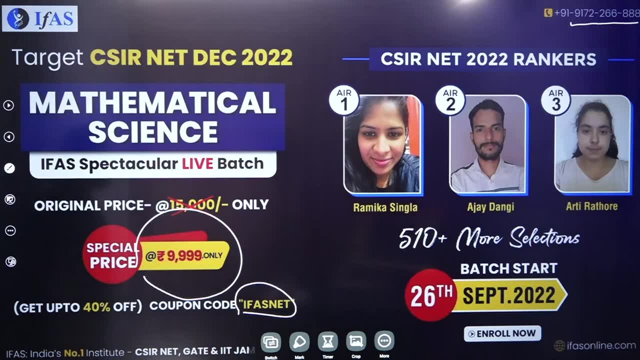 to. agar aap hamare sath judna chahte hain, to is number par aap call kar sakte hain. jo ki hai: 917226688 yaha. to aap hamare official website par visit kar sakte hain. theek hai, good morning. 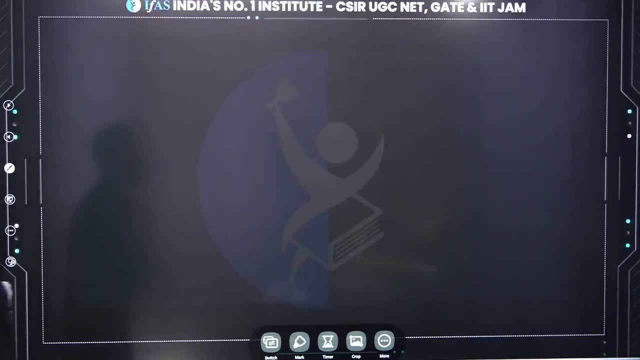 aap barte hain, aa jate hain agli slide par to aaj ham start karne wale hain. vector space. se theek hai to vector space padhne ke liye kuch cheeje jori hoti hain. 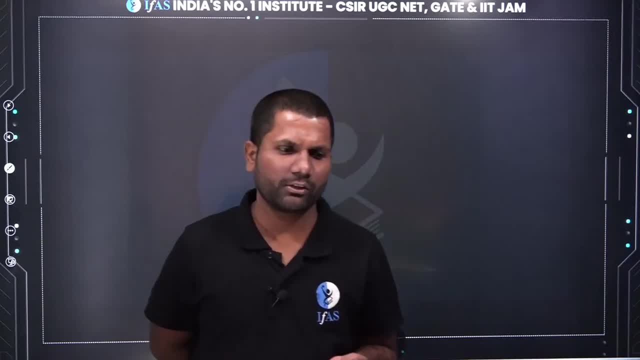 jase aapko koi kahe na: vector space. kya hota? agar aap vector space padhna chahte, ho na to sabse pehle aapke paas ek non empty set ho na. chahe bhi, aa subah ke time ek ghante hoga. 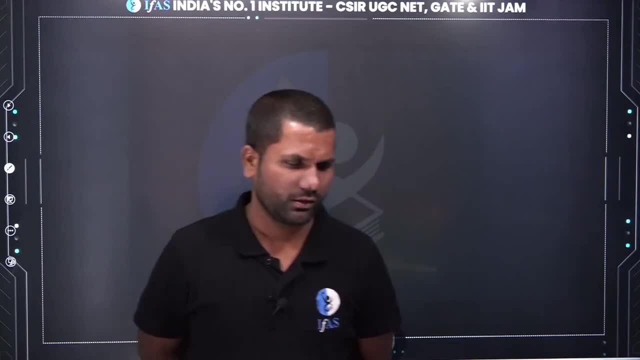 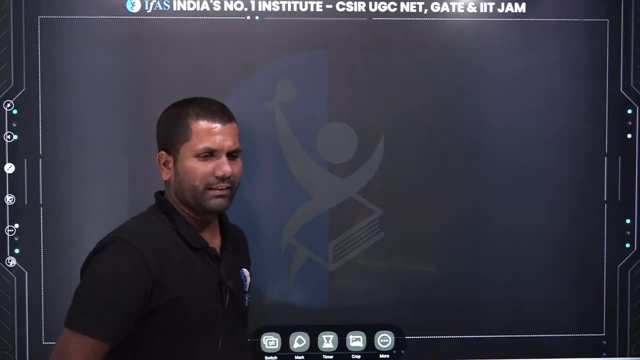 saam ko ek ghante, 2 ghante hoga. phil haal to is week theek hai. aa next CSIR ka exam to kaide se dekhe to december me ho na chahe, agar december me nahi bhi hota hai. 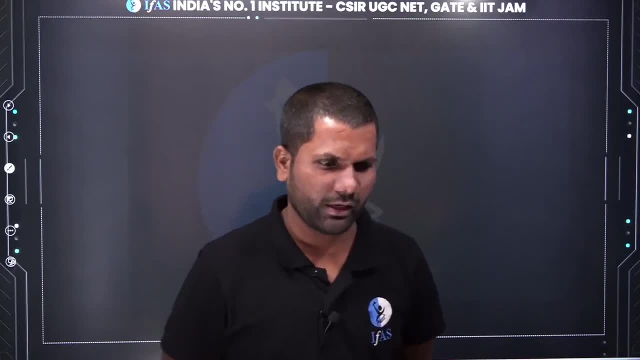 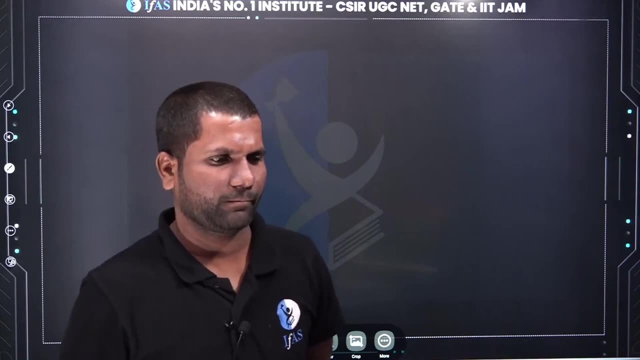 to maan ki chaliye, ki janwari, ya farwari tak to ho jayega theek hai. aa. good morning chandrakant to chalo guys. abhi, abhi tak jenho ne like nahi kiya to aap log. 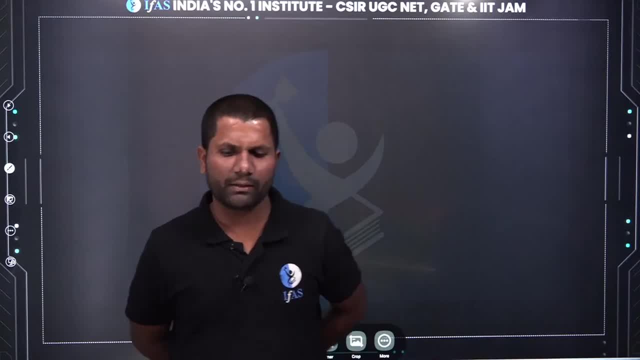 session ko ek bar like kar dije. phir ham start karate hain, to jaisa, ke maine aapko bataye vector space padhne ke liye hamare paas pehle to 2 cheeje honi chahe ek. 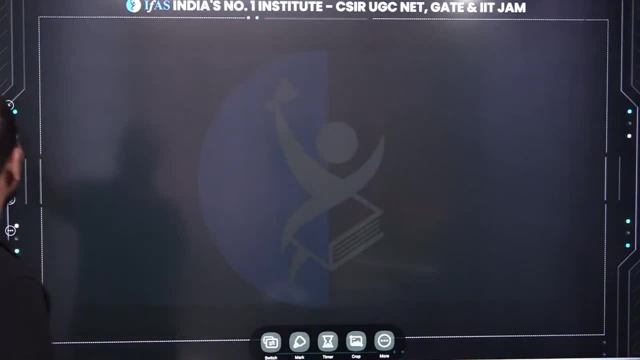 non empty set ho na chahe ek field ho na chahe to yaha par ham sabse pehle kya karte hain. dekho vector space ke liye sabse pehle hamne. ek field le liye aap, field le liye hamne. 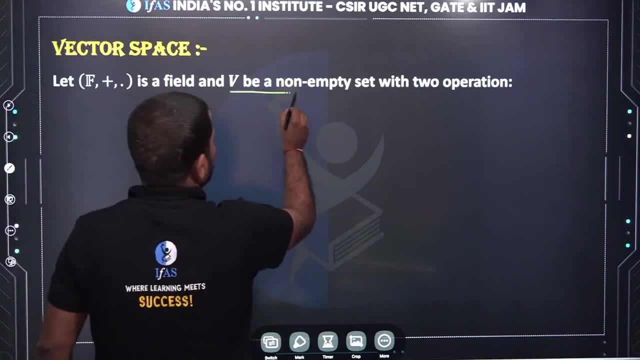 ab uske baad hamme kiske job padhege uske baad aapke paas ek non empty state ho na chahe v hamne liye liya ek field, aapko job. padhege ek non empty state, v ke job. padhege ab uske baad yaha par. 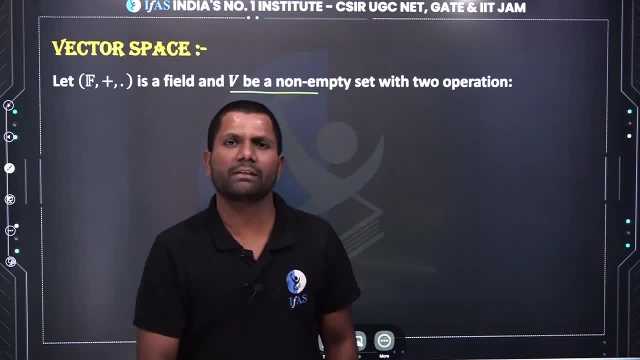 vector space me 2 tare ki operation. hote hai operation? kya hote hai, kaise hote hai, kab hoga, kyu hoga? usse ham discuss karte hai, jise ki maine bataye. vector space me 2 tare ki operation. 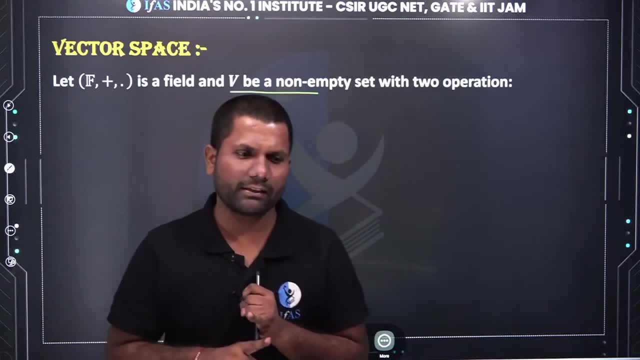 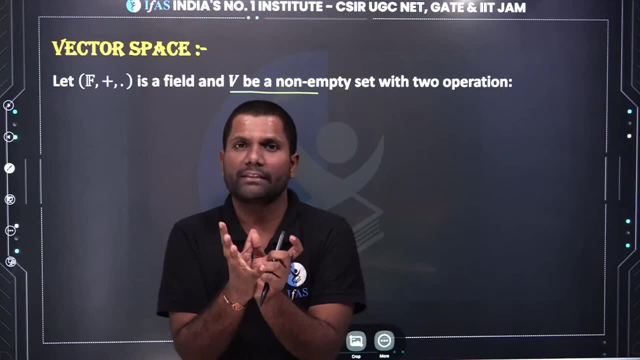 hote hai, ek ka naam hota hai vector addition, ek ko ham kehte hai vector addition. second ko ham kehte hai scalar multiplication, vector addition. naam se hi pata chal raha hai, ki add karna vector addition. hume ye batata hai na. 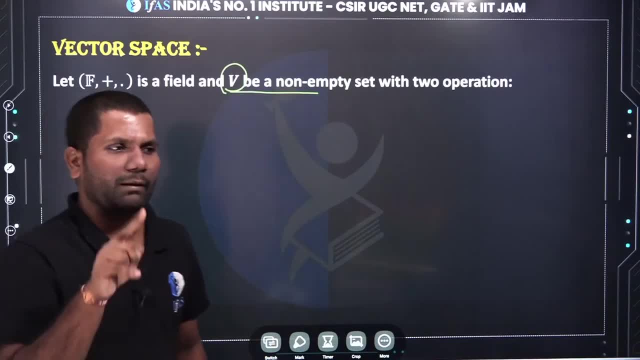 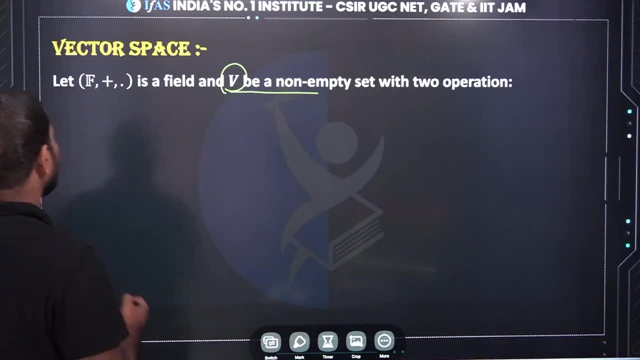 is v ke 2 element ko ham kaise add kare? uske baare me hume kaun jaankari deta hai. uske baare me hume jaankari deta hai: vector addition ab scalar multiplication. scalar multiplication, ye hai na field ka. 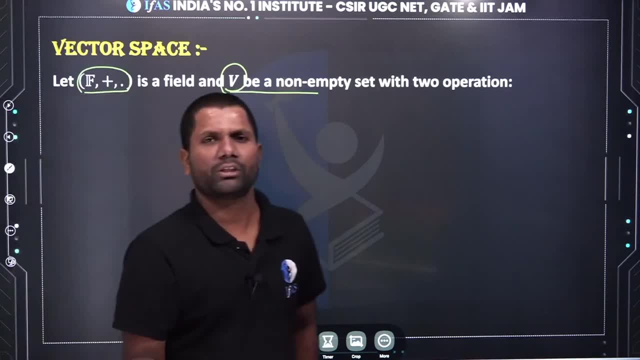 ek koi element, le lo field, matlab, aapka field koi bhi real ho sakta hai, complex ho sakta hai, zp ho sakta hai, jaha par p prime ho ya rational number ho sakta hai. field koi bhi ho sakta hai. 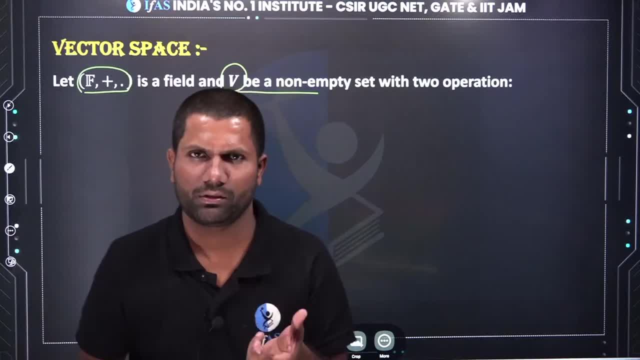 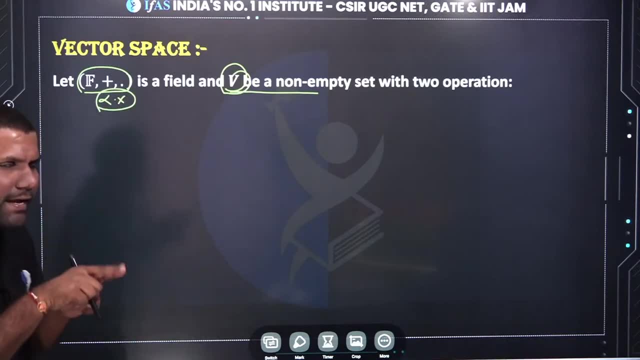 to abhi ke liye samajh lo: field ka element, matlab koi ek number, hamne koi ek number le liya, yaha se ab ek element, yaha se le liya suppose ab in 2 element ko field ka ek element, v ka ek element. 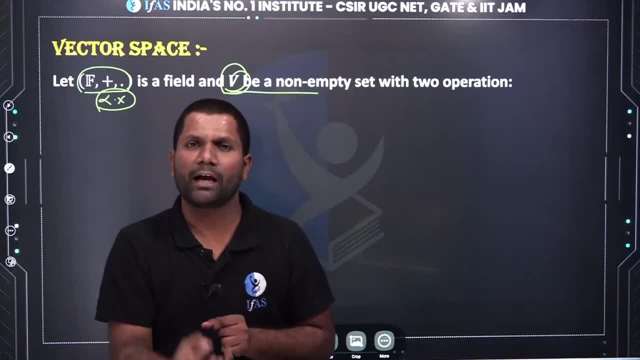 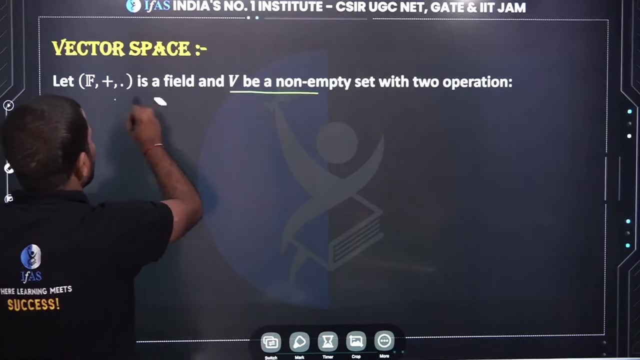 kaisa multiply karna hai? o tarika, ya o rule: hume kaha se milta scalar multiplication se to vector space padhne. ke liye hume 2 chiji chahiye, ek to vector addition, ek to aapko. kya chahiye, field chahiye. 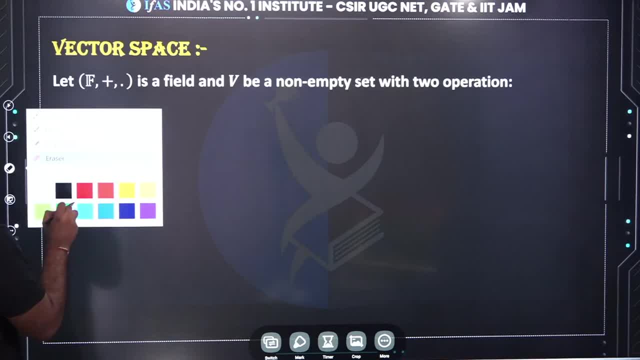 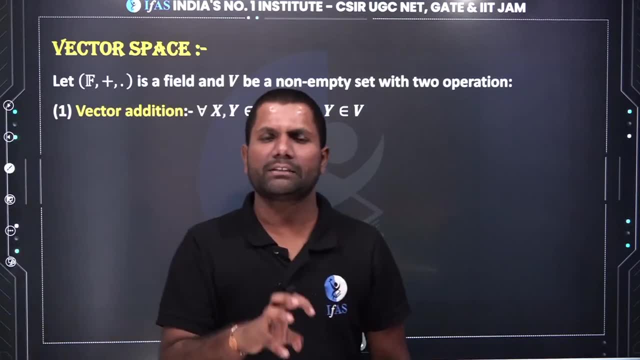 non empty set chahiye. ab uske baar hamare paas 2 operation hona chahiye, ek operation ko hume kya kehte hai: vector addition to vector addition. kya batata hai: vector addition? hume ek rule batata hai ki. 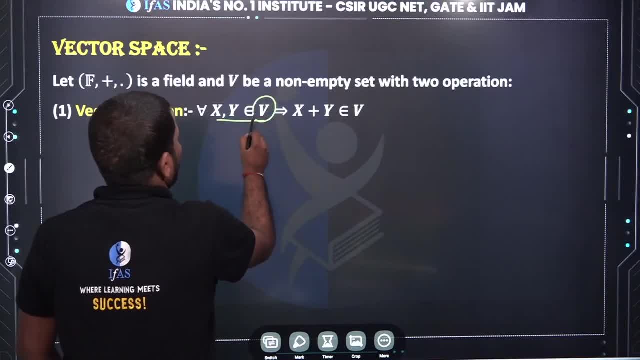 is v ke 2 element ke element le lo v ka koi 2 element lene par aapko kaha par milna chahiye unka addition. unka addition bhi aapko v me milna chahiye, agar v ka koi 2 element lo. 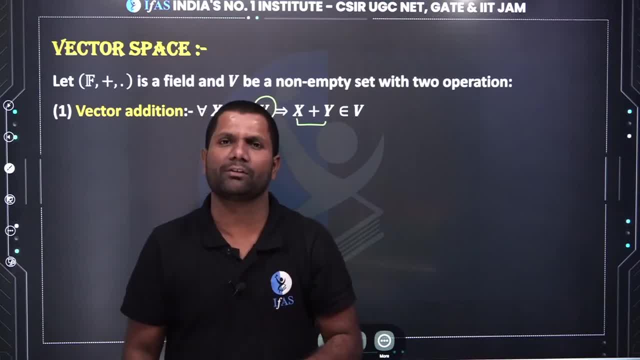 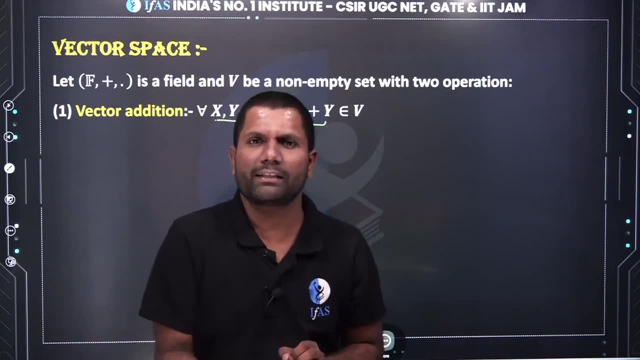 add karne. par firse v me mil jaye to hum. kya kehte hai ki v jo hai na closed hai with respect to addition. v is a closed with respect to addition. iska matlab samjha agar v ke koi 2 element lo. 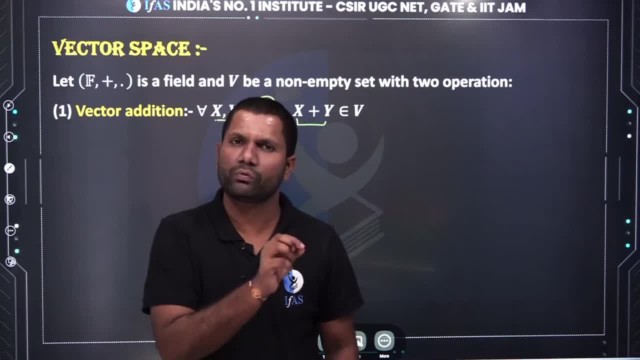 usko add karo. firse v me mil jaye na koi bhi 2 element to aap. kya kahoge jo v hai na v closed hai under addition. abhi to baat hoge vector. addition to 2nd operation kya hai? 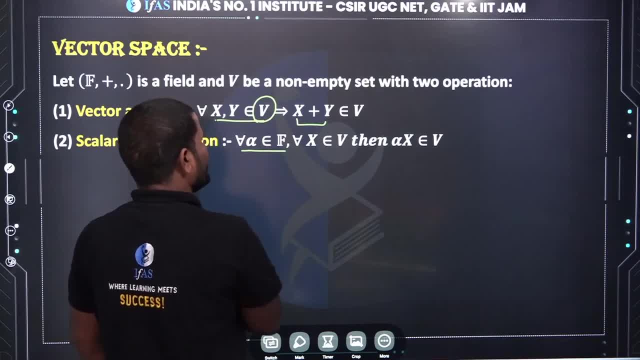 scalar multiplication. jaise ki aapne koi ek number le liya, field se ek koi element le liya, v se to us case me yaha par aapko ek rule diya jayega ki aapko alpha dot x kaise multiply karna hai. 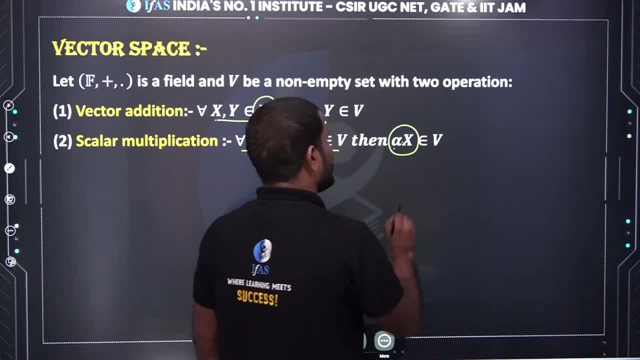 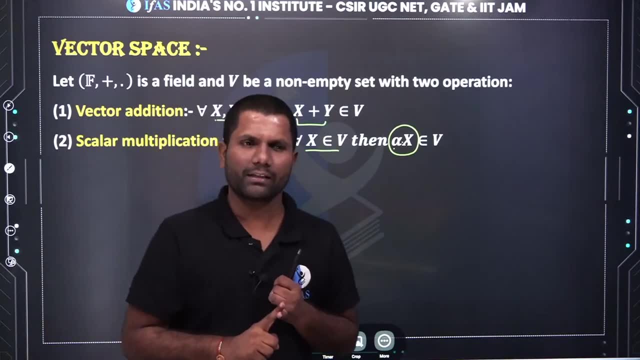 aur jab aap multiply karoge, na to multiply karne ke baad, aapko v me hi milna chahiye. agar aisa hota hai, to hume kehte hai: v is a closed under scalar multiplication. to yaha tak abhi aap log ko clear hai. 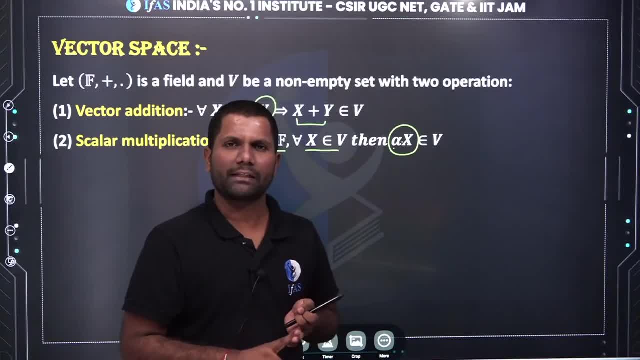 vector space padhne. ke liye hume ek field chahiye, ek non empty set chahiye, 2 operation, ki jyot padhti hai, aur dono operation, kya hone chahiye, closed hone chahiye. vector addition bhi closed. 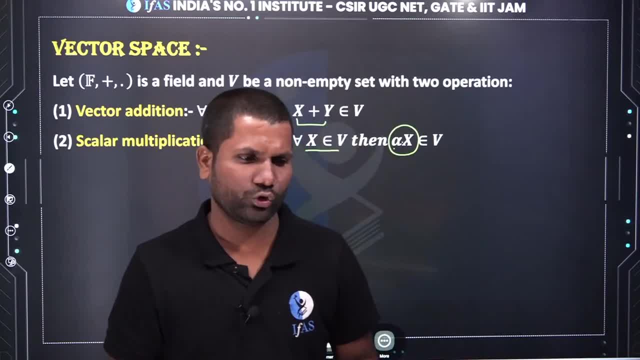 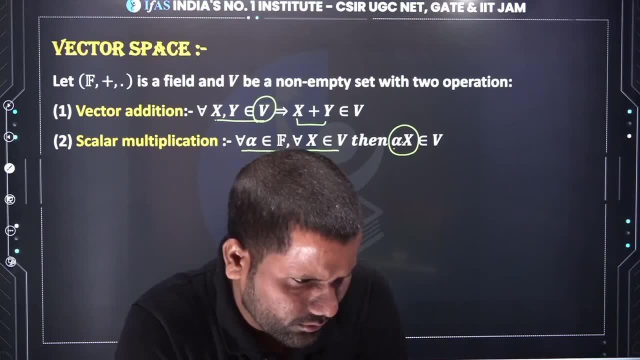 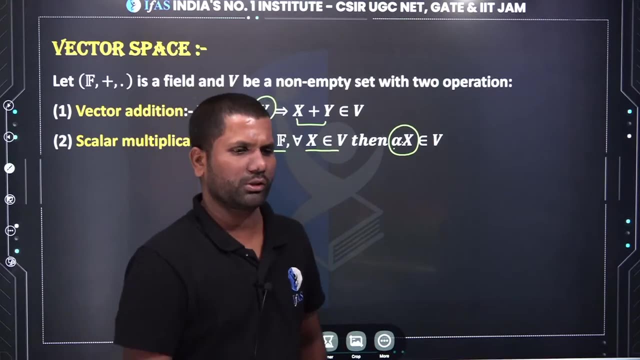 hona chahiye aur scalar multiplication bhi. aapka kya hona chahiye? closed hona chahiye. good morning, sadhavana, rastogi ji sadhavana. ok, ok, sadhavana, good morning. normally session saam ko hote the to good. 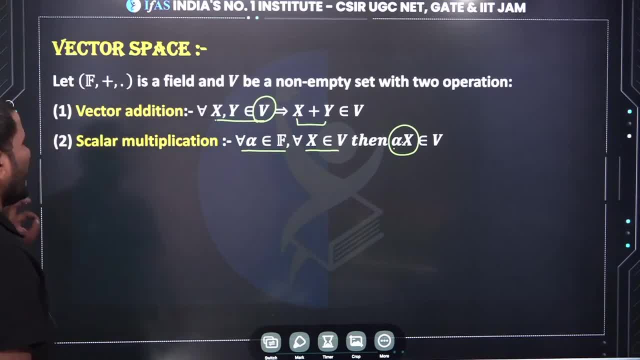 morning hi nikal jata hai mo se ab baad karte hai ki isko hum aakhir vector space. kab kahenge to us case me? v is called vector space over a field if following axioms hold for any vector: xyz to agar koi non empty set. 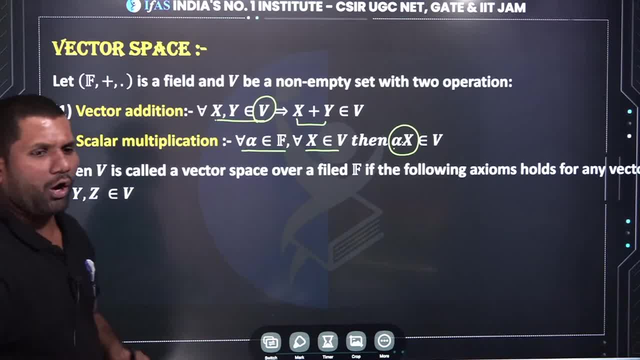 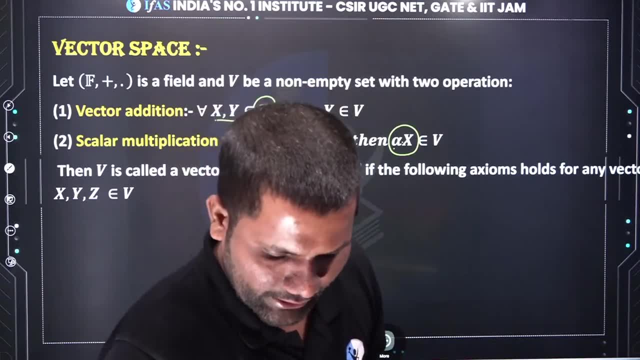 jaha par ek vector addition ho, ek scalar multiplication ho, aur ho kya kare, 8 properties ko satisfy kare. agar 8 properties ko satisfy karta hai, to usse hum kya kehte hai. us case me hum kehte hain: ho kya hoga. 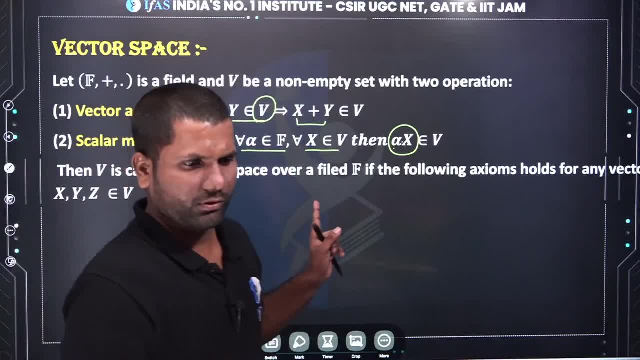 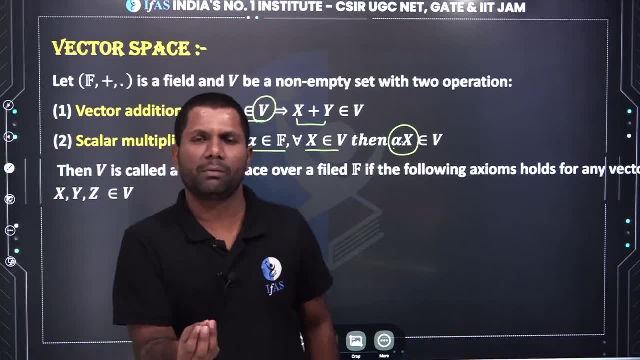 vector space form karega tika. good morning rahul tika. so yaha par dekhe kaun kaunsi property hai. group theory me aap logon ek property pada hoga. group theory me kya hota hai? ek to aapka closure hota hai. 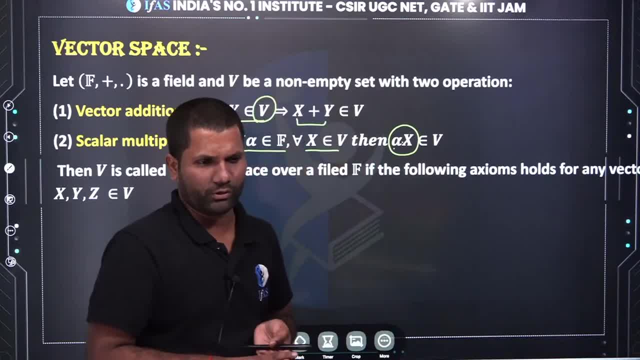 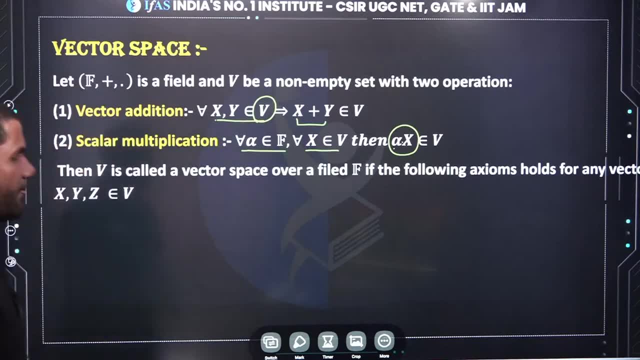 associative hota hai, uske baad identity hota hai, inverse hota hai to saare property. yaha par bhi hoga real. saam ko chal raha hai ultra easy mathematics. saam ko chal raha hai real tika 6 beje se. 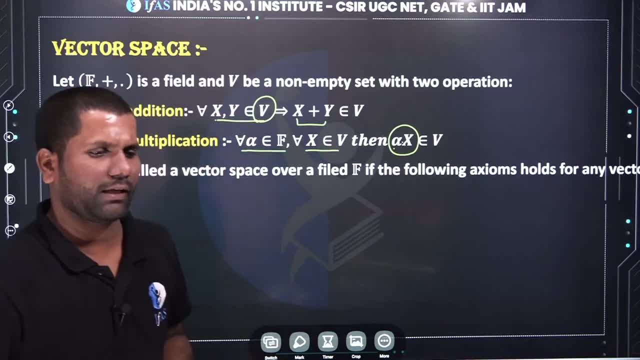 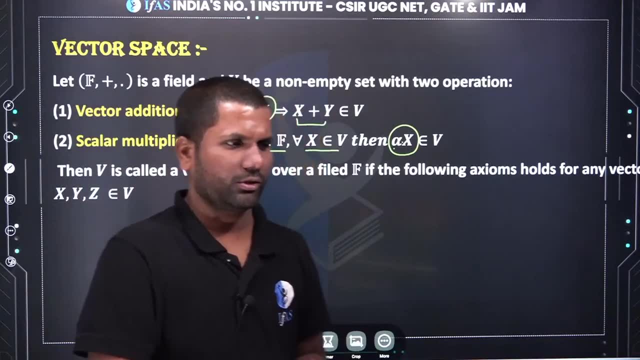 ha ha, bilkul tanu, pehle ek baad definition bata leta ho. fir example bhi aap logon ke liye lekar aaya ho. example, bilkul, hum discuss karenge. good morning, show them, tika. so chal, ye jo log abhi jod rahe hain. 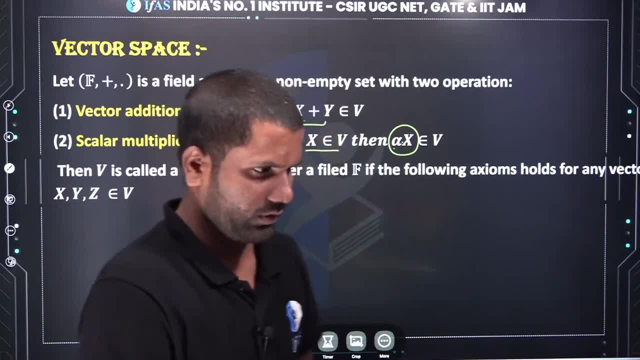 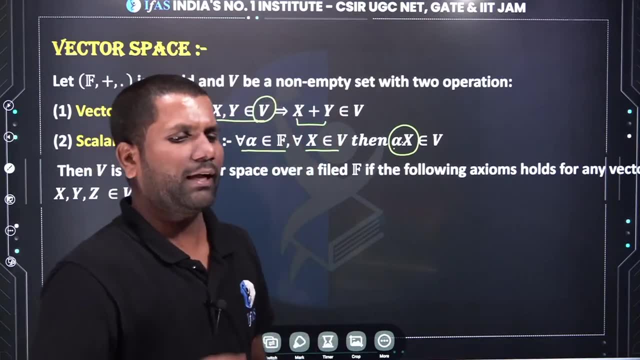 agar aapne session ko like nahi ke haon to fada, fada like kar dije session ko youtube par. jo bhi hota hai, sandesh kumar, free hi hai youtube wala, agar aap paid padhna chahte hai to aap. 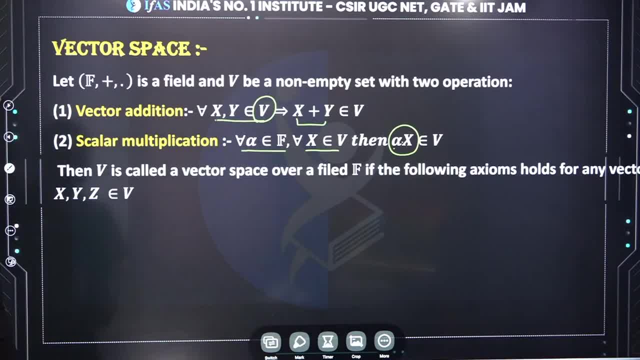 amare saath paid bhi jod sakte ho. chalo ab yaha par. dekho ab yeh pehla property kya satisfy karna chahi associative. yeh jo addition hai, ta hai na addition kya hona chahi associative hona chahi. 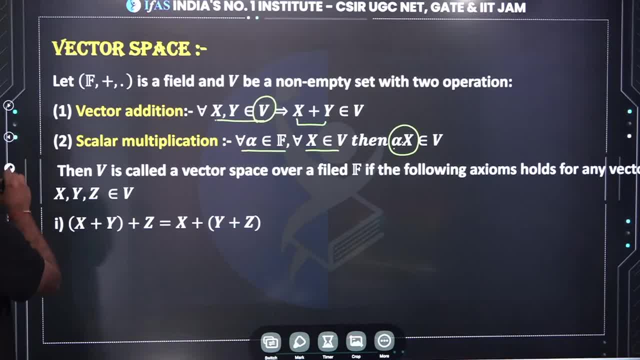 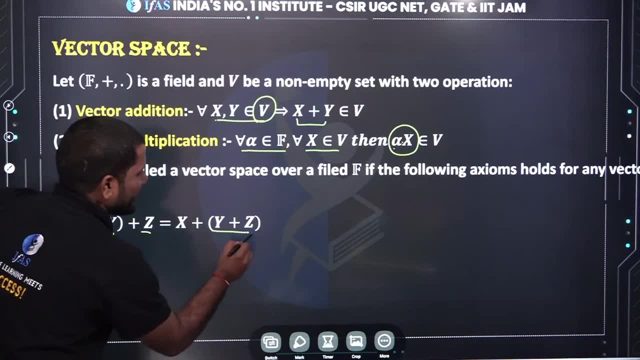 associative hone ka matlab kya hota hai. dekho, associative hone ka matlab ek hai. na ki chahi aap pehle in 2 element ko add karke, fir iske saath add karo, ya last ki 2 element pehle add karlo. 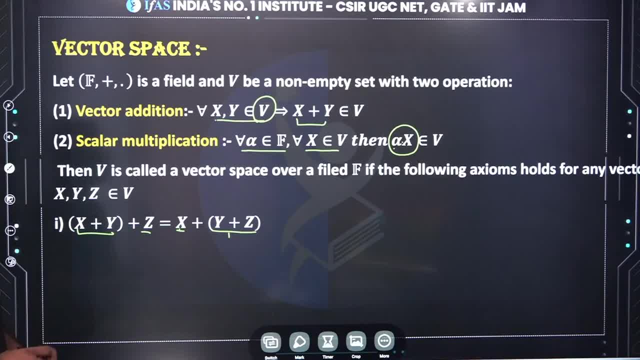 fir, jo bhi iska answer milega, isko iske saath add karo dono case me aapko result: kya milna chahi, same milna chahi. agar aisa hota hai, hum, kya kehte addition, kya hai associative? 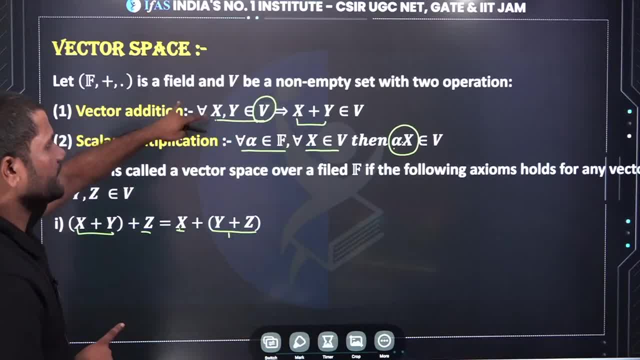 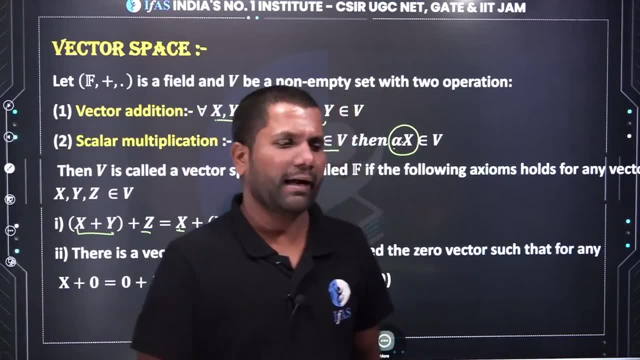 hai tike associative wale property satisfy karne chahi. abhi hum addition ke property dekh rha hai. second, second aapko kya karna hai? na second, aapko identity find karna. identity find karne ka matlab kya hai? 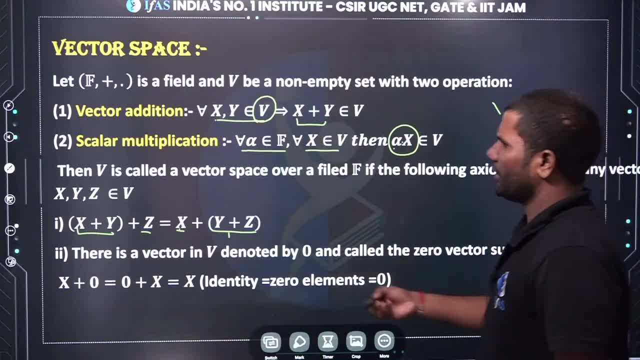 hota hai. jase ki maine aapko koi ek element de diya, chala example ke liye samajh lete hain, maine ek element aise de diya. abhi koi real number le liya. v maine real number, for example, hai. 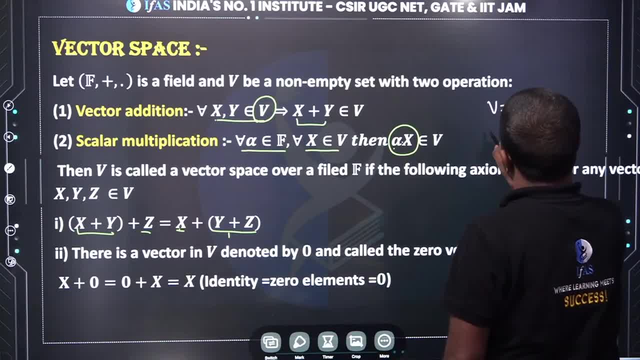 v maine kya le liya, real number le liya, abhi yaha par koi bhi ek element le liya, jase ki suppose maine phai le liya, abhi phai me mai aisa kya add karo. 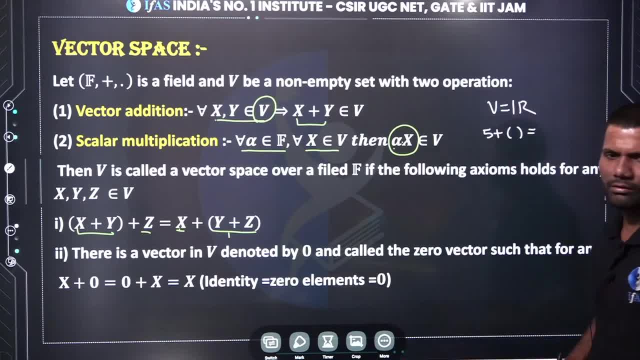 matlab: mujhe phai hi mil jaye. batao aisa mai kya add kar do, ki mujhe phai hi mil jaye. batao aisa kya add karoge ki aapko phai mele, aapko jabab hai. 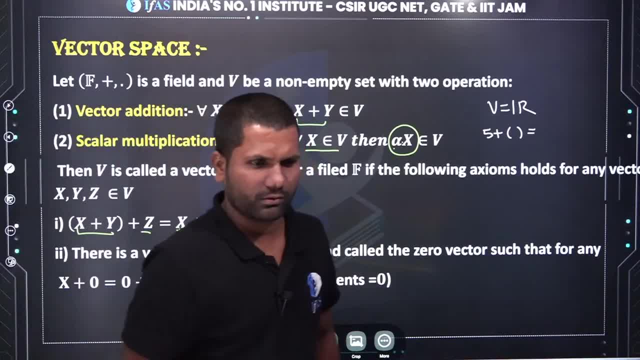 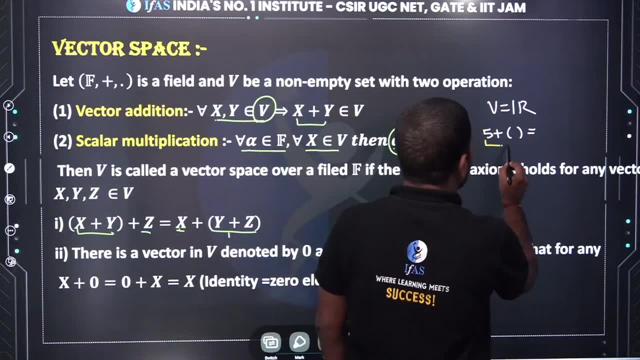 is phai me. aisa ham kya add kar de ki aapko phai hi mele, aapko phai me le. bilkul unstoppable study, bilkul so yaha par. agar ap dekhoge, agar aap phai ke sath, yaha par. 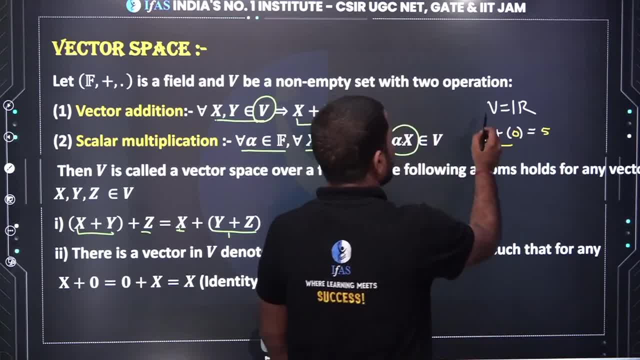 zero. add kar do to phai hi mele ki aise kya ja sakta hai ki v ka koi bhi element le lo usme aap kya add karogi ki wohi hamesa element mele aap dek sakte ho ke zero? 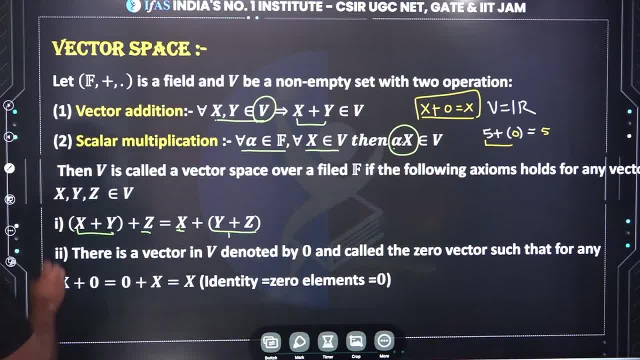 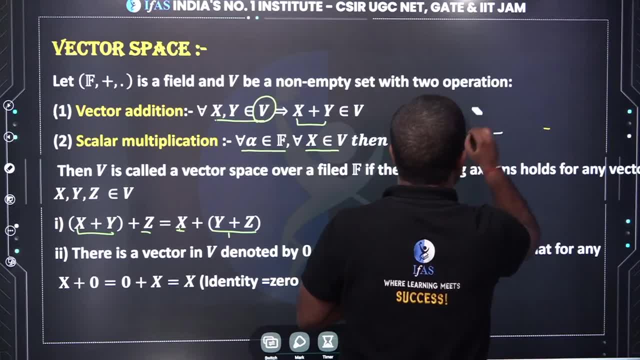 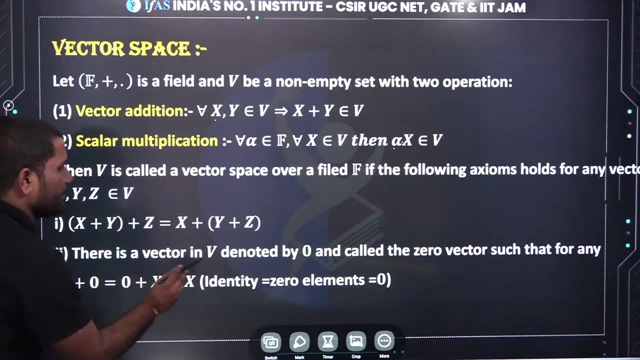 ko add karna padega, only so yaha se hume pata chalata hai. e The zero that you have found in a different way. we call it identity element or additive identity. Here you can see that there is a vector v denoted by zero. 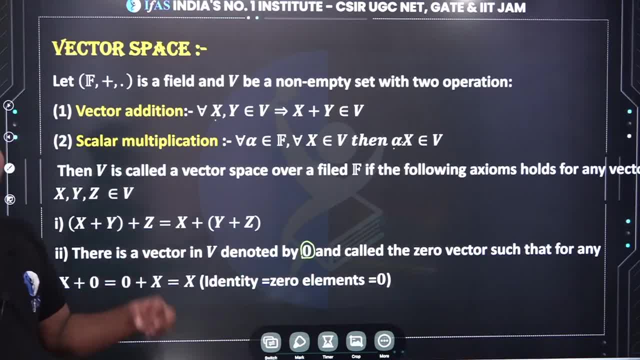 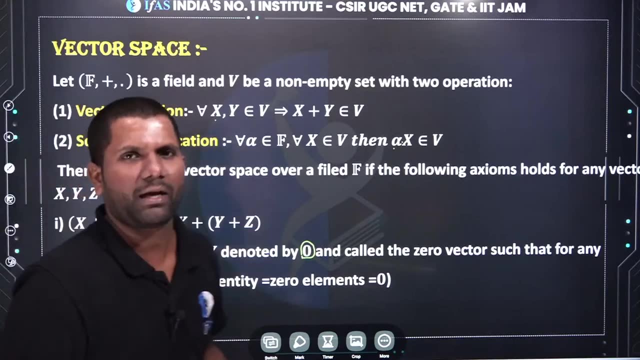 You have to find a vector which you will call zero vector or represent by zero. Call the zero vector such that means: add that zero vector with any vector. Add from left or right. you should always get the same vector. If you are able to do this with every element, in that case, what do we call this zero? 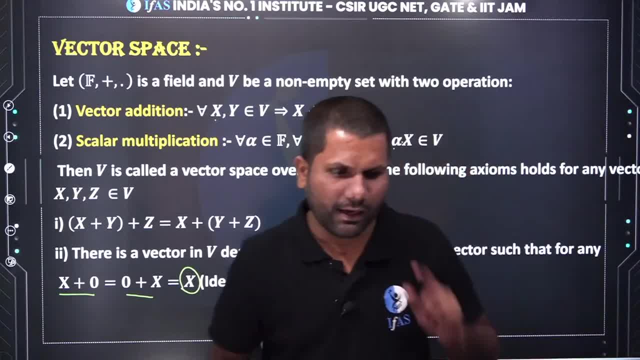 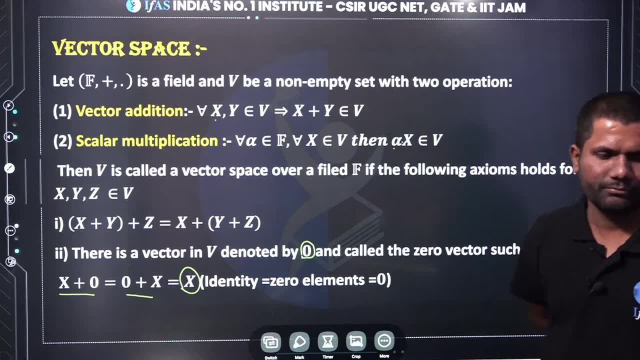 It is called identity or zero vector. Is it clear so far? Is it clear to everyone so far? Take a look. Okay, This is the identity element. As I said, eight properties. The first should be associative, the second should be an identity element. 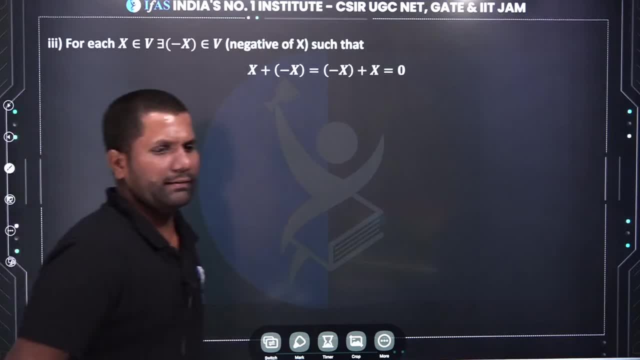 Now let's talk about the third property. The third property says that you have an identity Now. x is your a Now, with this x, which element should I add to get the identity? Now, tell me, who will you add with this? 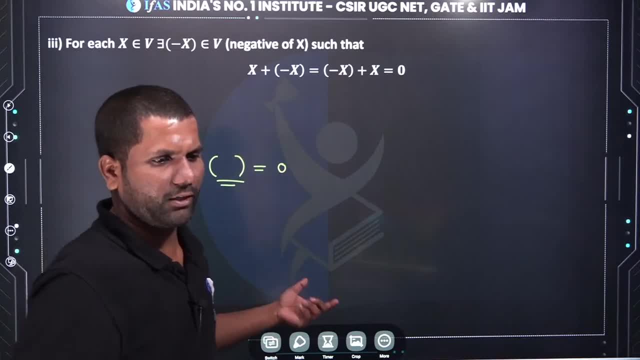 Yes, it is also called additive inverse. With this, who will you add? Tell me, what do you think? Who will you add to get this zero? So here you can clearly see that if you add x with minus x, then you get zero. 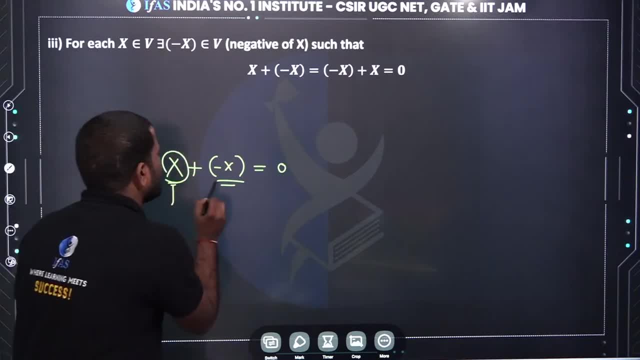 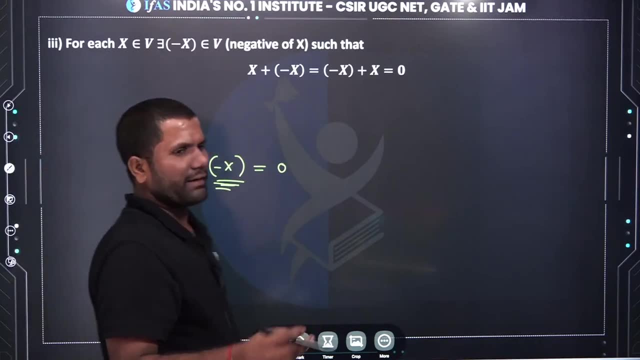 This means we say that what is the inverse of x? What is the inverse of x? It is minus x Meaning. Did you understand? So here, what will be the inverse of x? It is minus x Meaning. if you want to find the inverse of any element, then you have to add such an element. 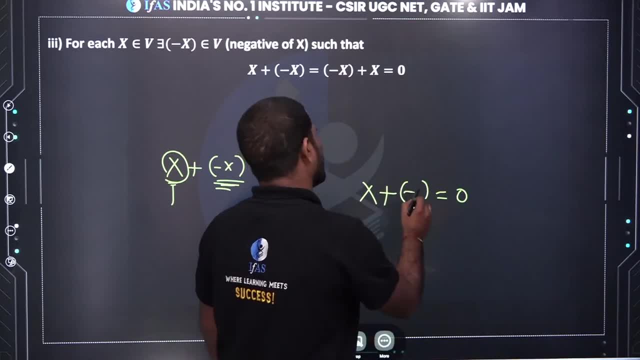 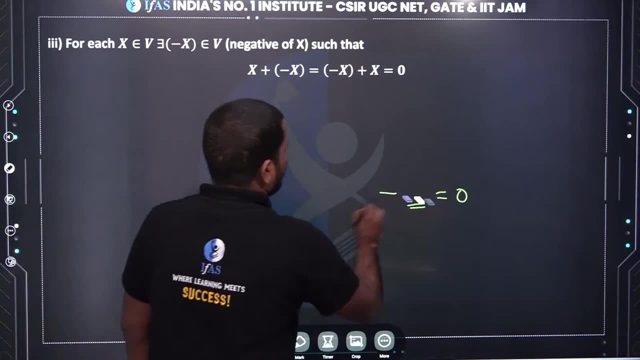 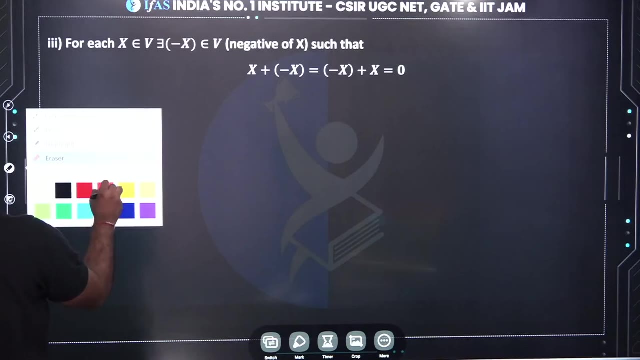 here so that you get zero after adding it. What will be the inverse of x? It will be minus x. Okay, So every set that you are going to make, V as a vector space. what should be there for every element? There should be an inverse for every element, or we also call it a negative element. 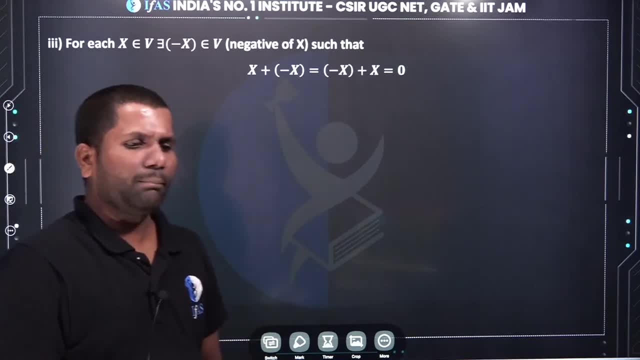 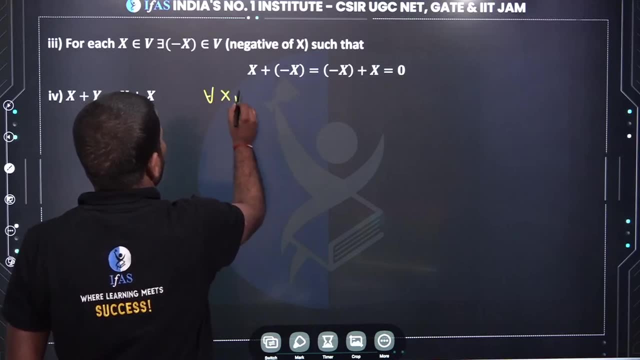 Okay, Is it clear to everyone so far? Okay, Now let's talk further. What is the next property? The next property says that take any two elements of V. take any two elements of x and y from V. Either do x plus y first or do y plus x first. 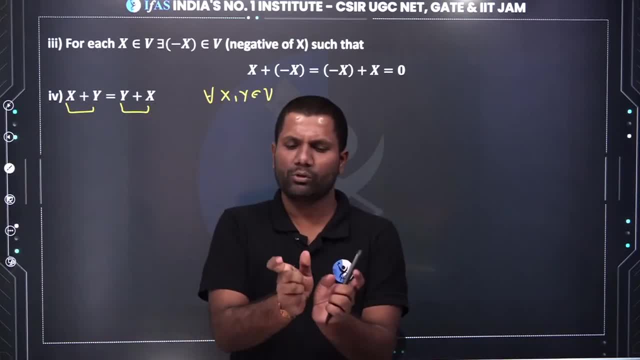 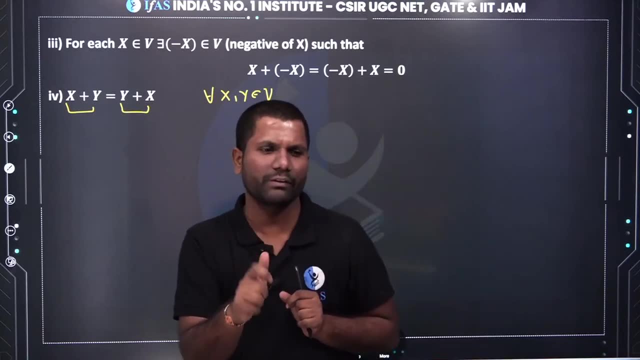 You should always get both the results same. Either do x plus y first or do y plus x first. What should you get? both the results. You should get the same Meaning. the element should be commuted with respect to addition, So Okay. 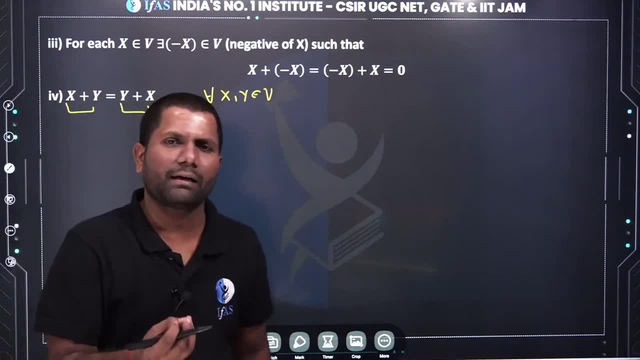 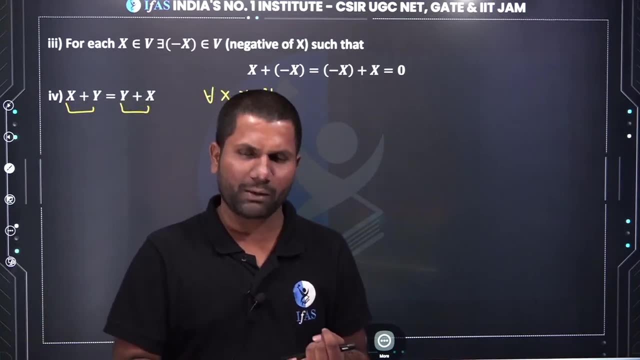 Okay, Now you have read some of the group theory so far. Do you remember We say that G under addition abelian group? Abelian group means that every element will be commuted. What does group mean? Closure property should be satisfied. 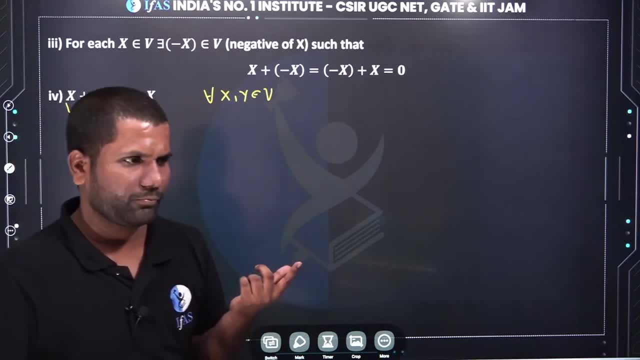 So we have taken closure property here at the start. Okay, So what we have seen so far is that your V. under addition, you can still say that it is an abelian group on this property. Tell me the strategy of jam Home car jam strategy. 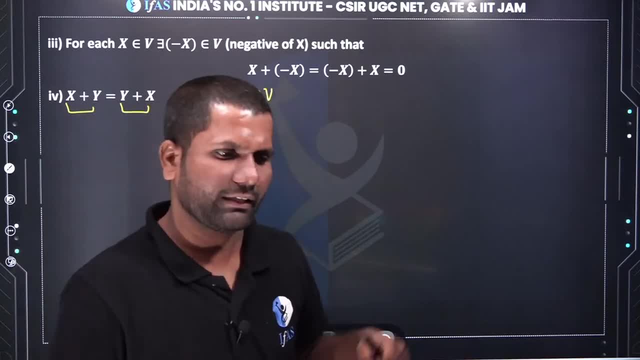 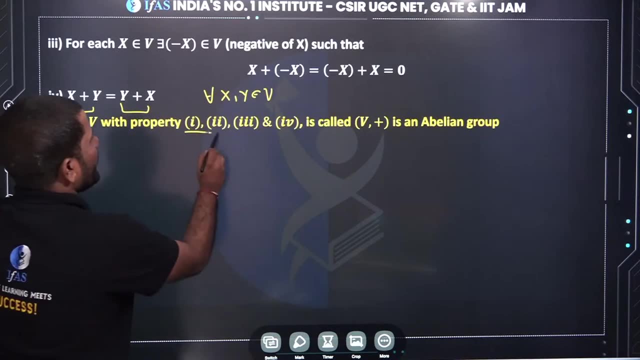 So we have already talked about the jam channel. If you have not seen, then also go and see. Okay, Now let's move ahead Here. see V with property one, two, three and four is called V. under addition is an abelian group. 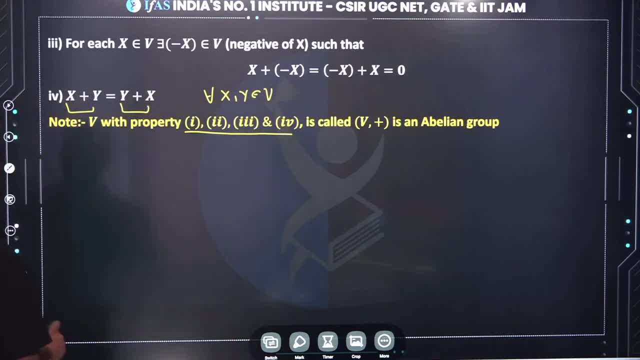 If you have read the group, then you know this. If you don't know, then nothing. Okay, Let's go. What is the sixth property? Whichever two elements or any two number you have taken, You have taken one element from V. 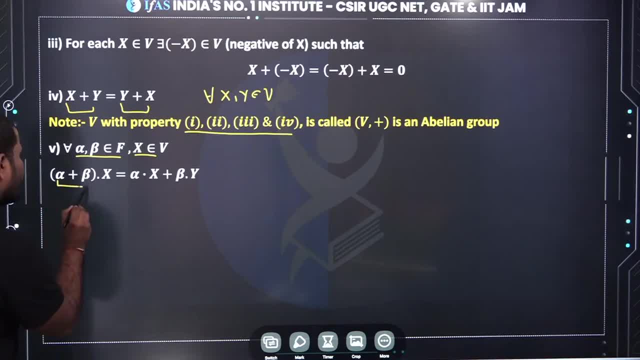 Now, whatever you do, first add those two numbers. You will not add two numbers, you will add those two numbers. there are numbers you will get the number after adding, after adding those two numbers, after adding those two numbers. multiply with any vector or what to do first. 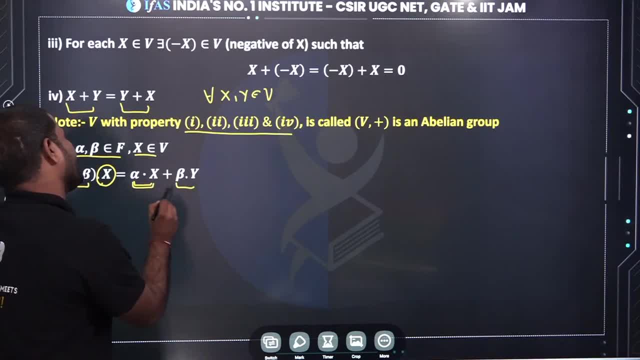 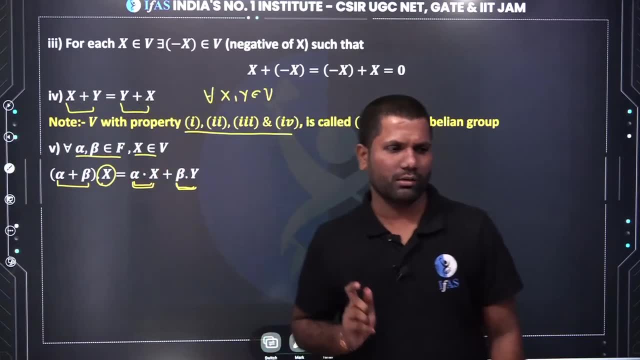 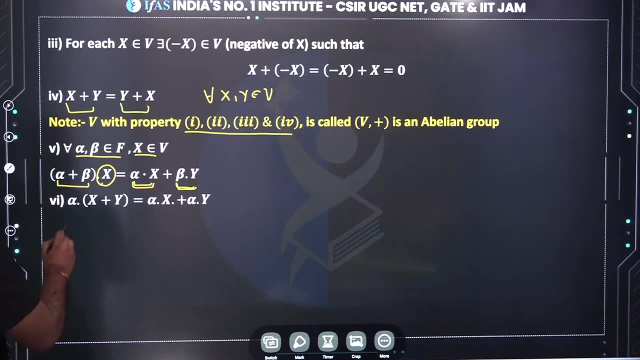 multiply with separate. separate vector means: take separate, separate scalar multiplication, then add in both cases, the result you will get will always be the same. good morning, sujata. ok, and sixth property is that you have taken one element. field side means you have taken one number. now you have taken two vectors of that number. 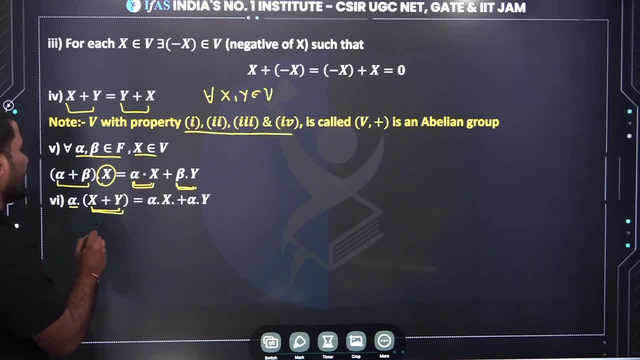 x and y. you can add two vectors first. after adding the vector, you will get a new vector. take scalar multiplication with it, or separate. separate scalar multiplication. take and add then in that case you should always get the same result, ok, ok, now let's talk about the next property, property number seven. 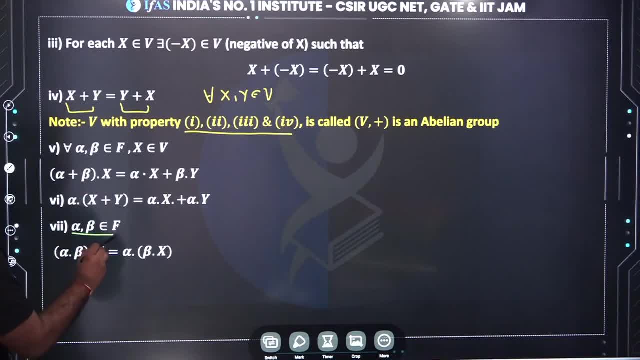 what is property number seven, that you have taken any two elements field side? and where did you take one element? you took it from v. so first multiply those two numbers, then take its scalar multiplication with x, or what do you do? first take the scalar multiplication of x with it. 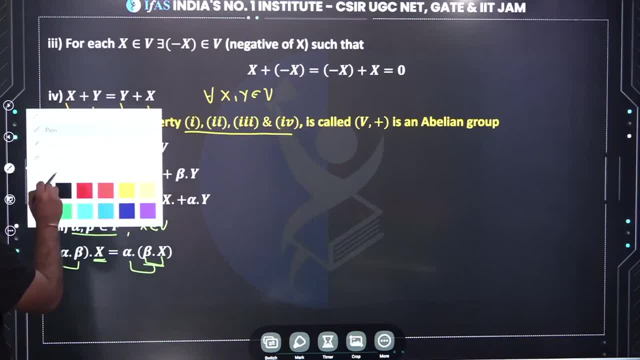 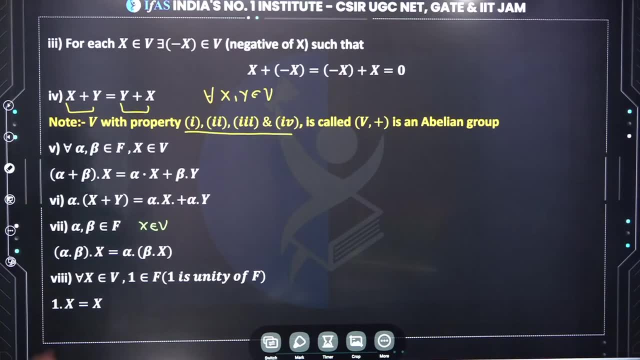 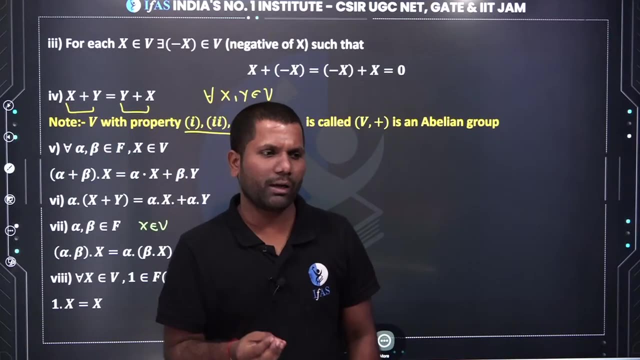 then take its scalar multiplication with it. you should always get the same result. and what does the last property and the eighth property say? see field, field has a unity. unity means multiplicative identity. multiplicative identity means: do you understand multiplicative identity? do you know? 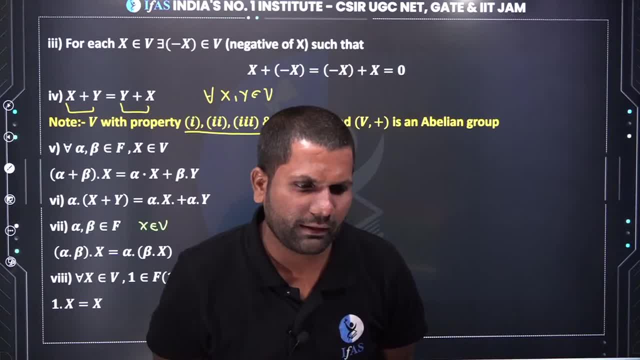 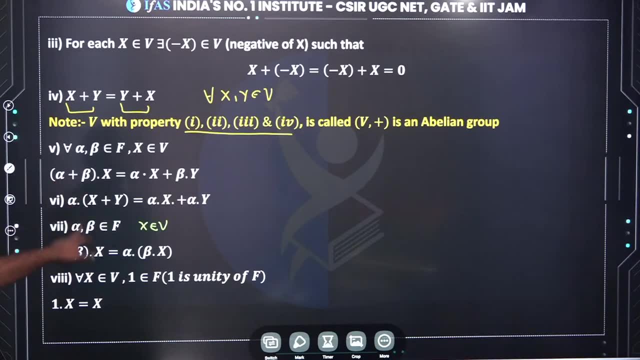 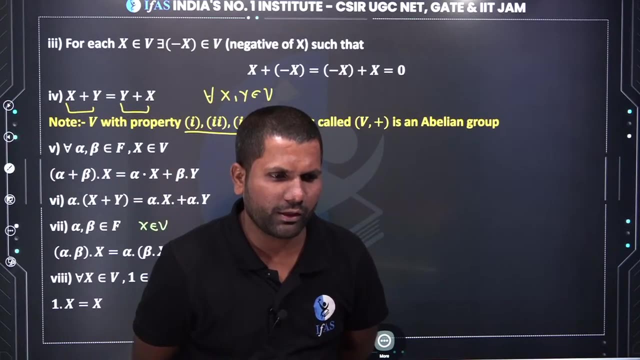 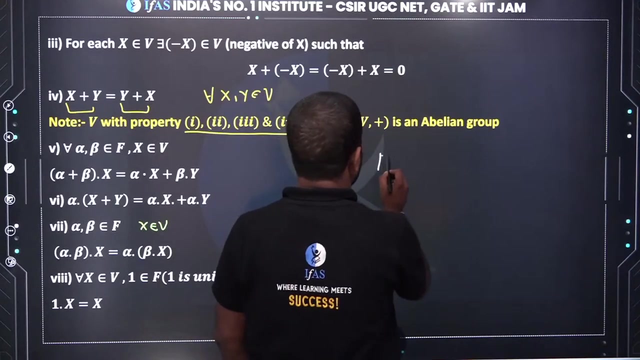 say max, sir, here it will be beta into x. where is the max here? no, no, ok, beta into x. there can be properties back and forth. these are the properties. ok, good morning, rajneesh kumar. ok, now here see the meaning of unity. as I say, I have given you a field as it is. 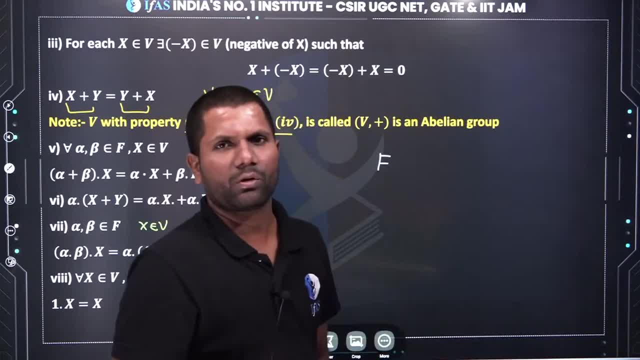 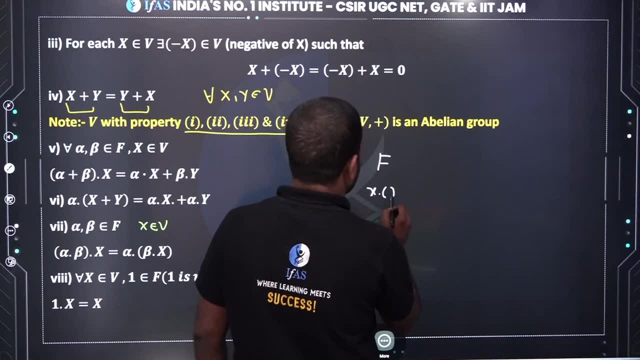 now I say that finding its unity means that now in that element from whom I multiply, you will get the same element. means, like I took x, now you have to multiply here. suppose y is from whom I multiply it, you will get it. if you get it from x, then will you do it from 1?? 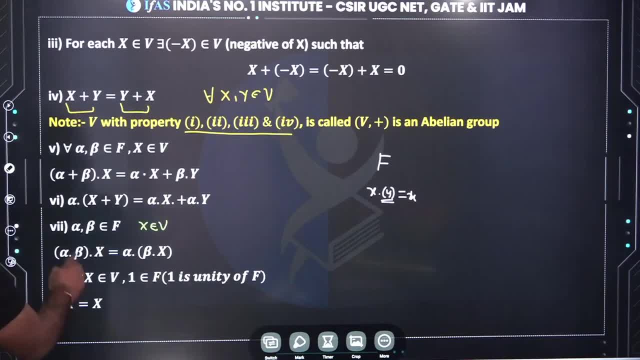 no, so here we call unity multiplicative identity as unity. like, suppose, what is x here? x is the element of v 1. we took unity of the field, so in that case you should always get 1.x equal to x in the fifth property. wait a minute, let's see. 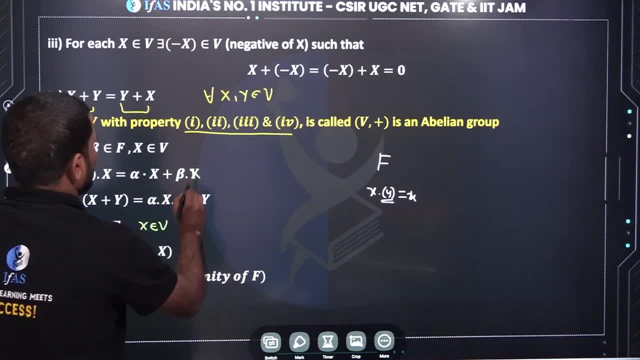 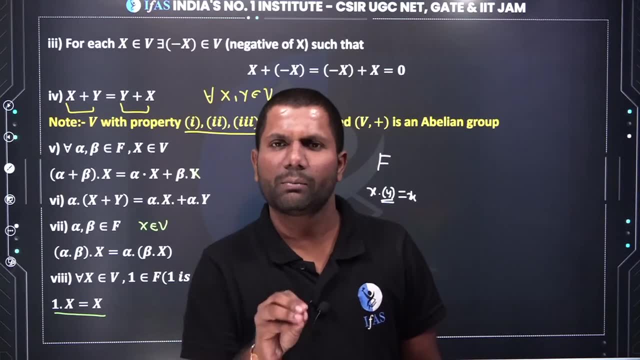 ok, yes, yes, here y will be. x will be absolutely correct. this typing was a mistake. ok, yes. like you ask yourself, what is unity in the real number? what does unity mean? what will be multiplicative identity in the real number? tell me. 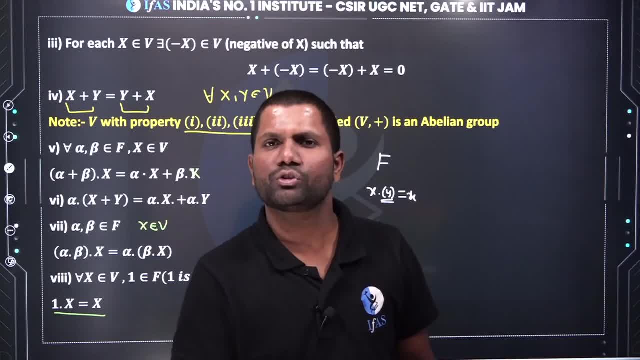 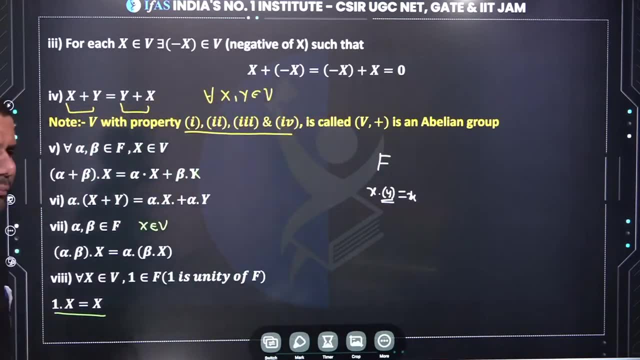 in the real number it will be 1,, in the complex number it will be 1 plus 0i, and in the rational number it will also be 1. do you understand multiplicative identity? see, it is clear till here. look at the definition. 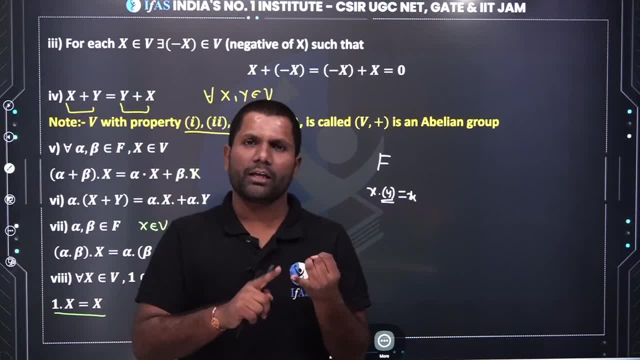 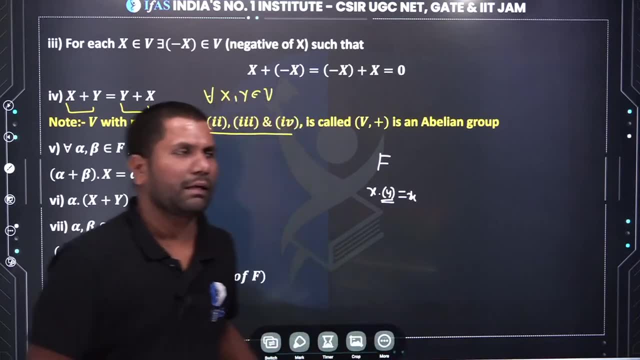 so if any non-empty set v, where a field has been given to you, there are two operations, one vector addition and one scalar multiplication. both the operations should be closed after that. if it satisfies these eight properties, then we call it vector space. 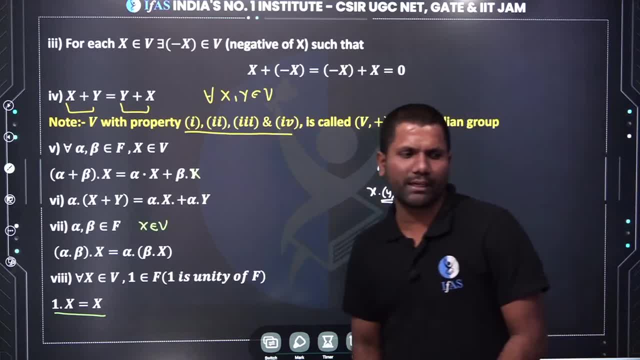 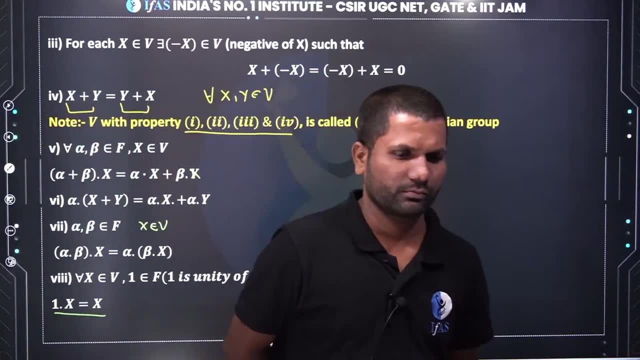 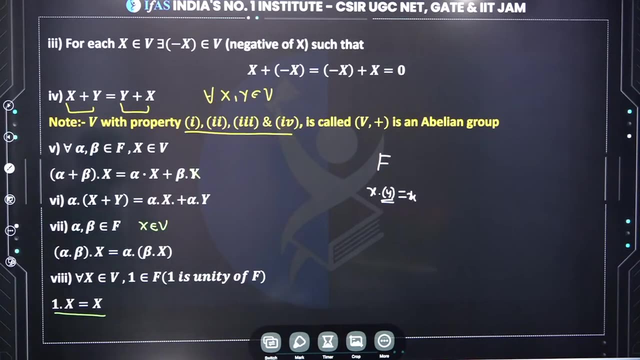 it is clear till here. see, so let's go. let's do some examples in vector space, the standard ones. see once: ok, go ahead, let's go. now we move ahead, let's go to the next slide. so here one thing to keep in mind. 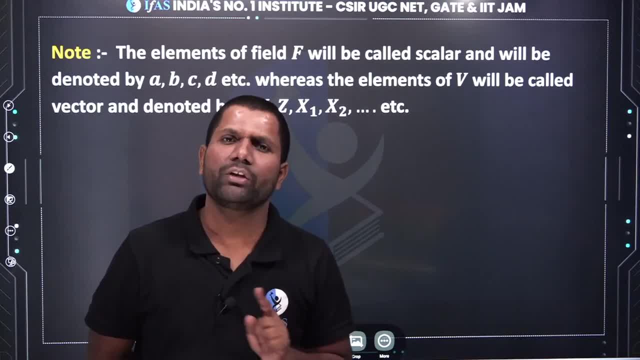 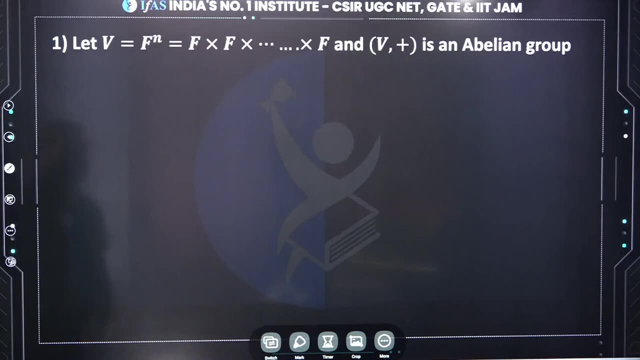 that the element of the field we call scalar or number, and the elements of v we call vectors. what will we call the element of the field, scalar, and what do we call the elements of f? sorry, we call the elements of v, vectors. ok, now here suppose I have now what can be your field. 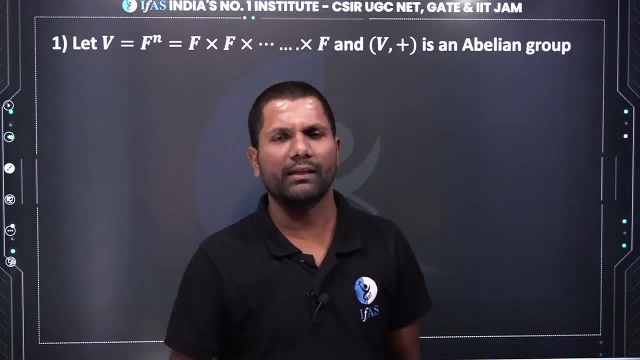 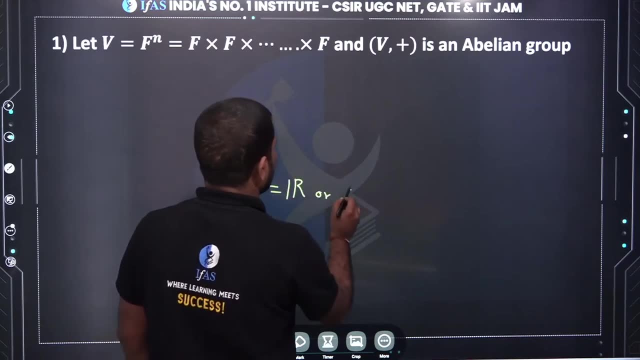 do you know? as you know, the field is fine or not. listen for now. you can read the field later. if you don't know, I will tell you some examples of your field. it can be a real number. it is complex, it is your rational number. 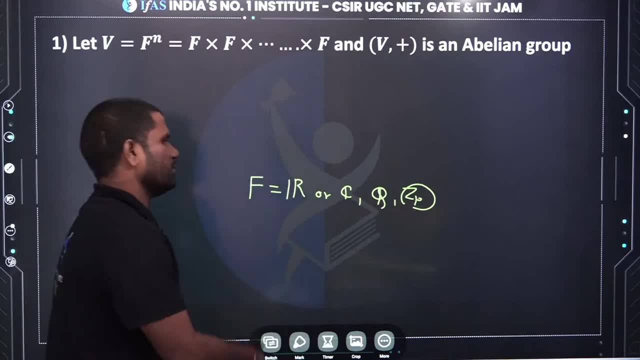 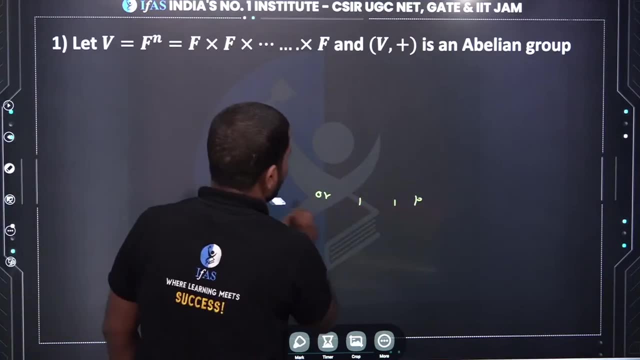 it is zp where p is prime. ok, so many infinite fields like this you will get ok. so what did I take here? see here, I took the field. how many times did I take the field f into f, into f. this is the field, like, suppose you took r, then the field will be your rn. 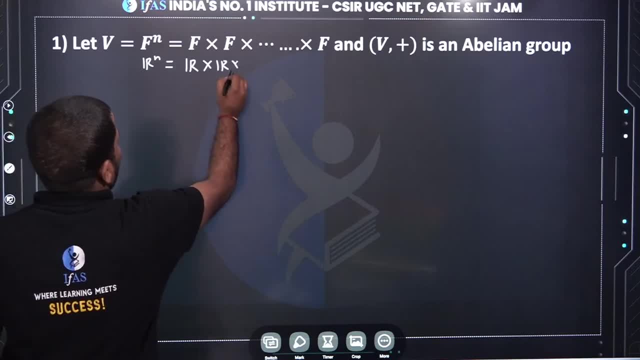 so what will be r into, r into and so on, what will this be r? so this will be your rn, ok, so in the same way, if you take c, then it will be cn, if you take q, then it will be qn. so here I have taken a field. 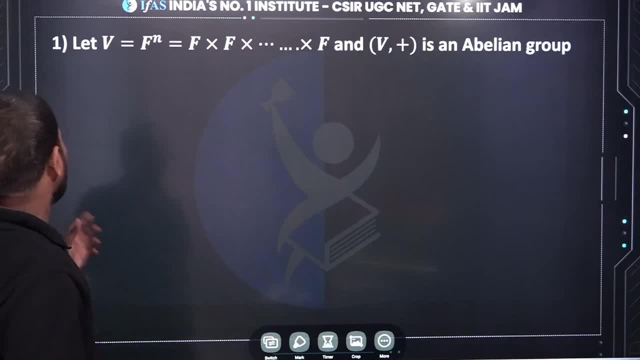 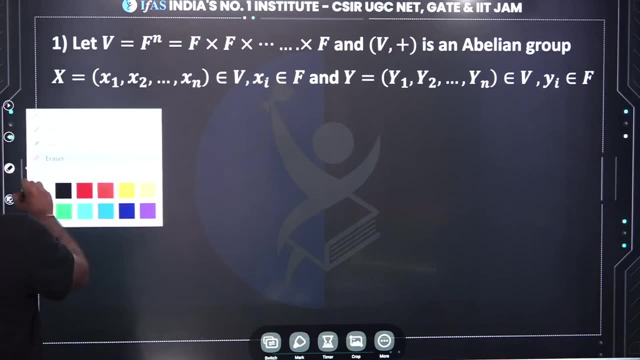 v is some non-empty set. ok, now what I will do. I will define two operations. now keep one thing in mind: the element of v. what kind of elements come in v? n-tuples? because see, one is its element, one is its and one is its. 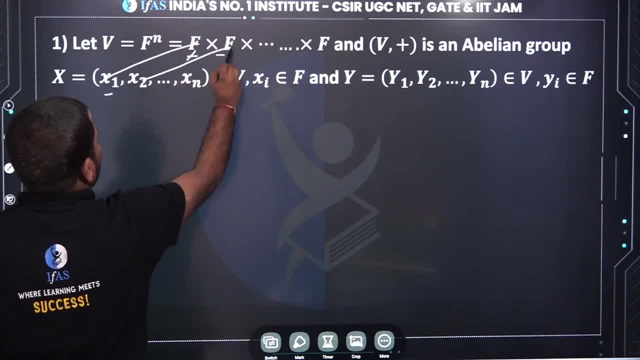 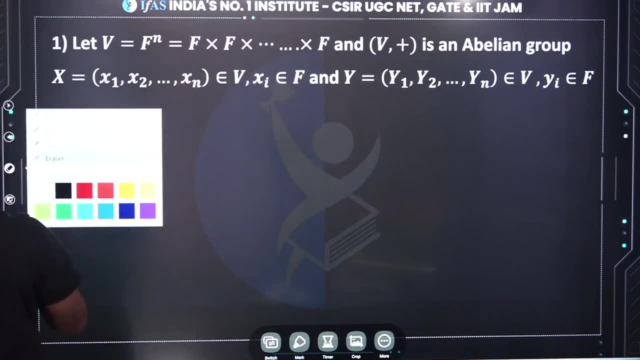 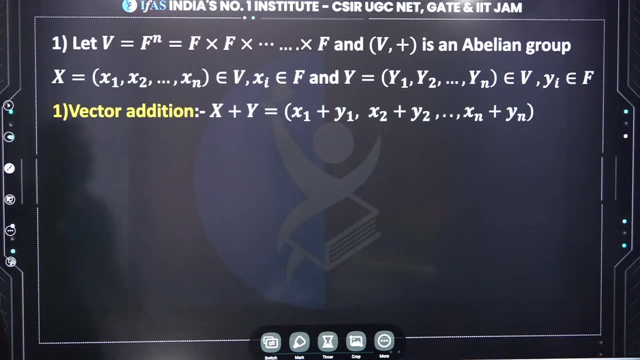 so x1 belongs to this f, x2 belongs to this f, xn belongs to this f. ok, so what did I do here? I took two elements from where from v, one took x and one took y. ok, now what do I do? vector addition. 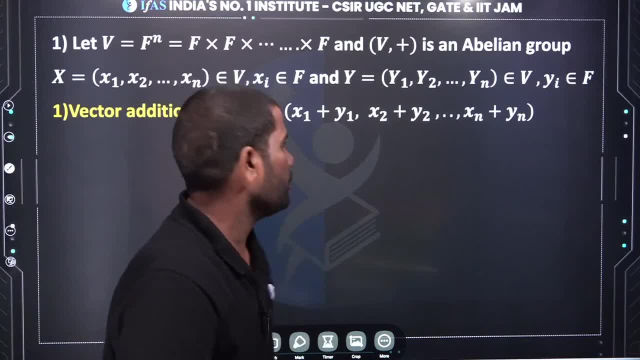 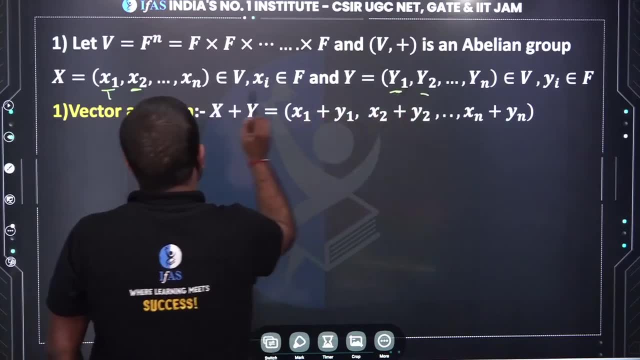 now I will show you how to add two elements here. you have given the rule of adding two elements. what is the rule? add this first element with this first. add this second element with this second. add the last element with the last means you have been given. 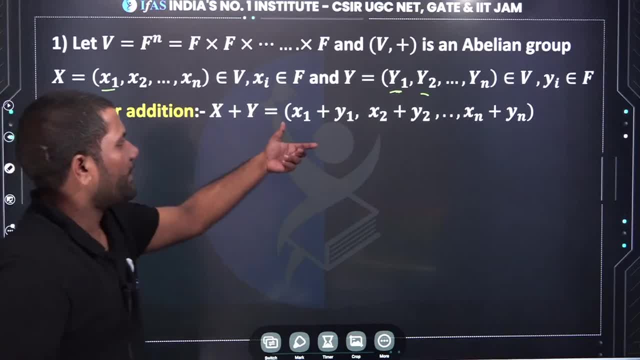 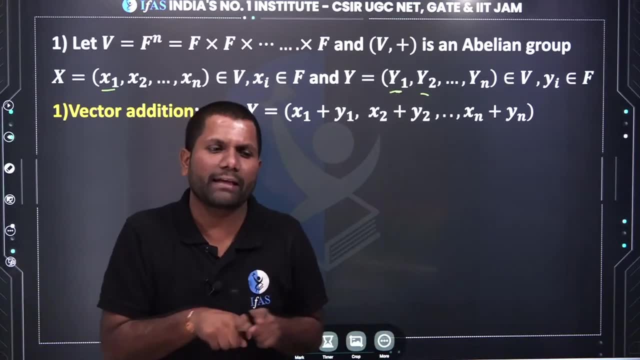 component wise addition. ok, so in this way you have been given by defining their addition. here you have been given a rule, you have been told a way how to add the two elements of v. rule of adding is a ok. good morning, shapna kumari. 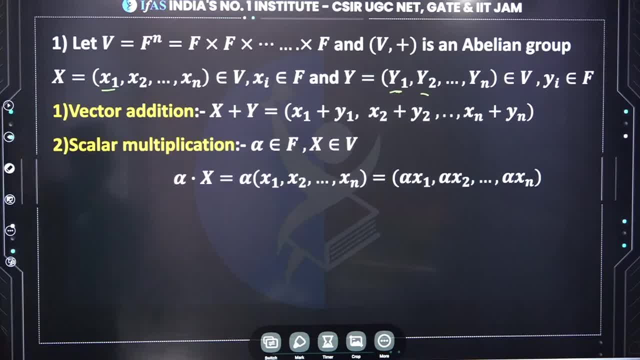 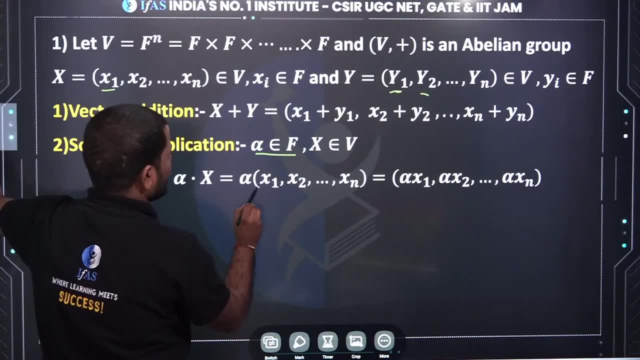 good morning, shapna kumari. ok, now here see what is given to you in the scalar multiplication. in the scalar multiplication, you have been given any element we took from the field. we took one x, so alpha into x. what will you do? you have to do alpha into x. 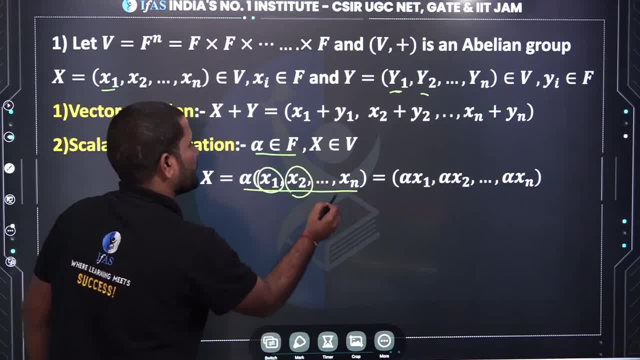 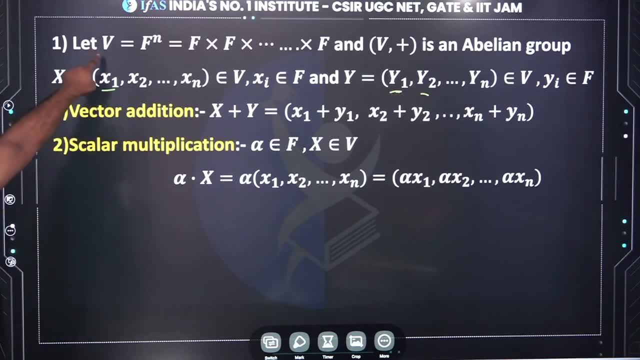 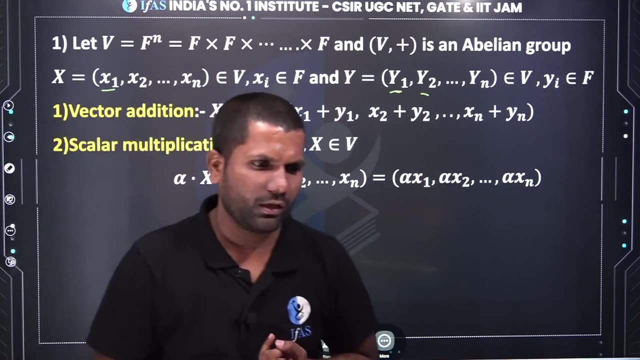 means: multiply alpha with this, multiply with this, multiply with this, multiply with this. in this way, what is given to you? scalar multiplication is given. so you have a non-emplicit v. now you have been given the operation vector addition. scalar multiplication is given. what to repeat max. 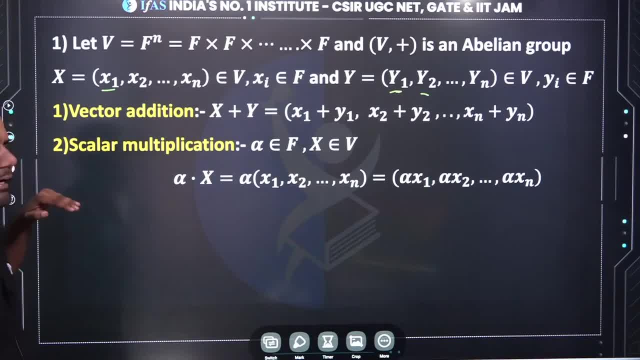 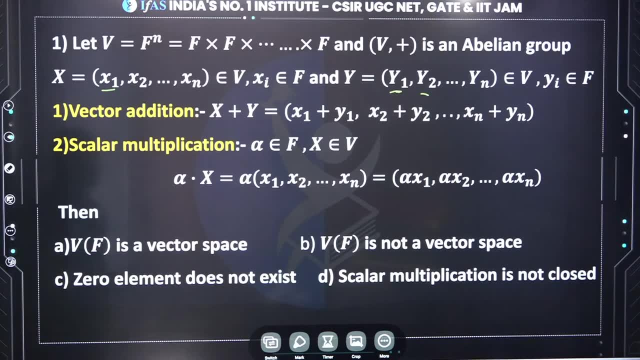 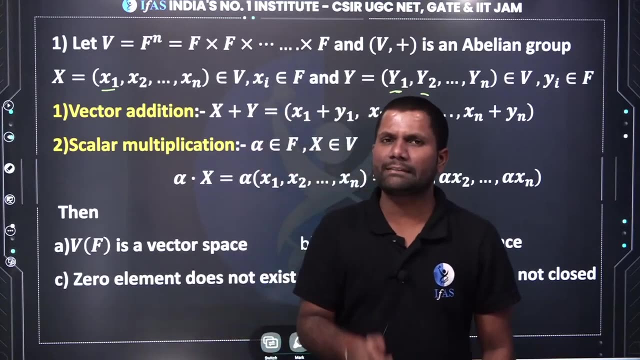 tell me. vector addition and scalar multiplication is given to you. ok, now tell you which one will be correct. will there be vector space of v over f? v over f is not a vector space. zero element does not exist. scalar multiplication is not closed. see if any non-empty state. 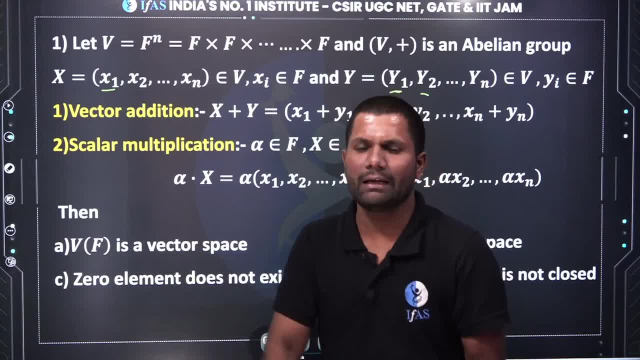 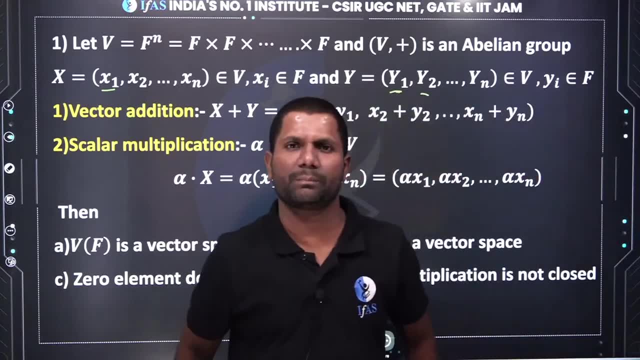 will form vector space. so see: vector addition should be closed, scalar multiplication should be closed and 8 properties should be satisfied. so overall you have to check 10 things, but we will check 10 again and again. or there is an easy way, absolutely easy way. we will discuss it in the coming lecture. 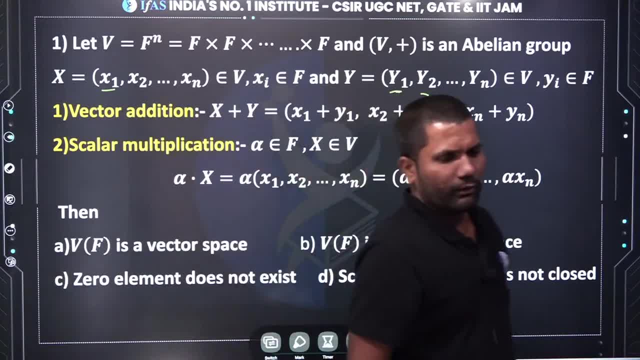 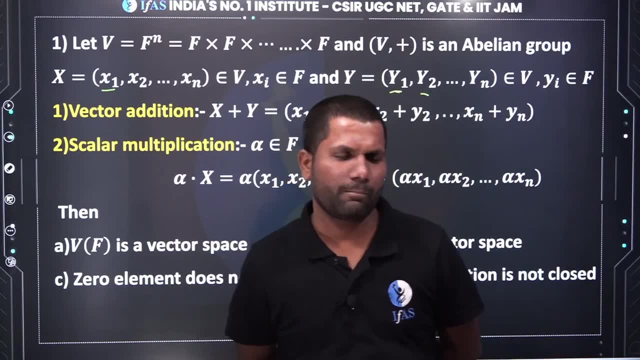 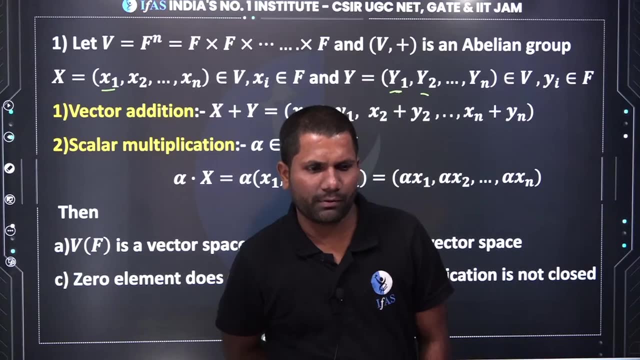 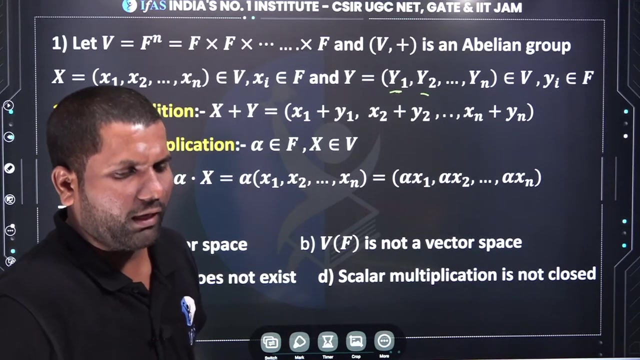 how you get to know. ok, for now, tell me about this. what will happen? chandra khan is saying this will happen. ok, max, what didn't you understand? prabhakar rao is also saying this will happen. ok, so, max, here this fn we took. 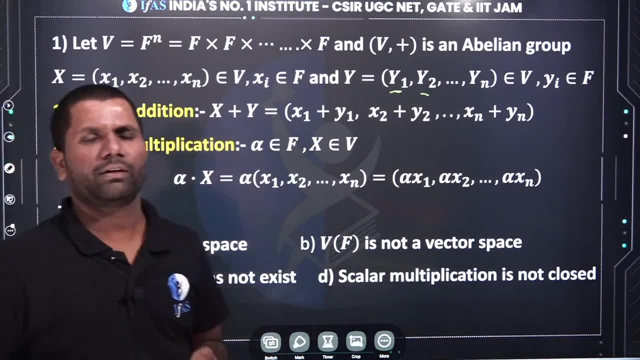 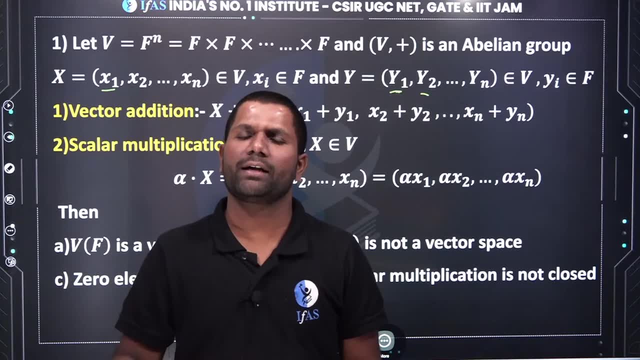 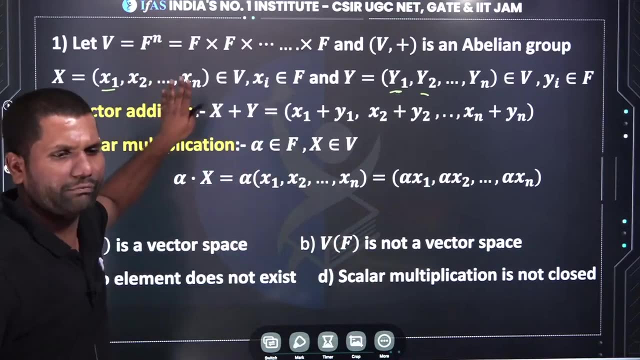 this is a field. what is a field? you take r like rn, cn, qn, zpn. if you take rn, it means r into r, into r. how many times? n times. by the way, taking cn means c into c into n times. we took a field. this is not a set. 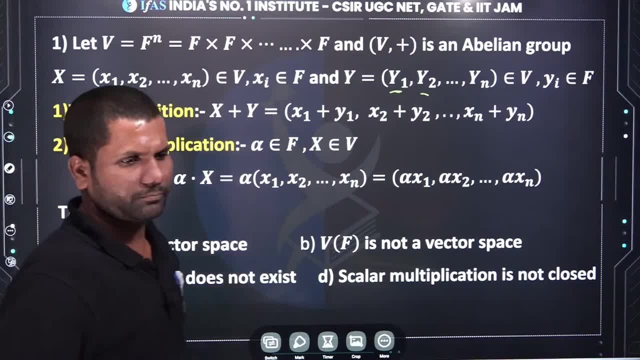 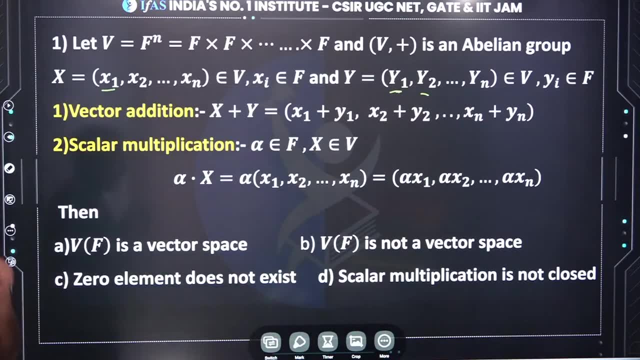 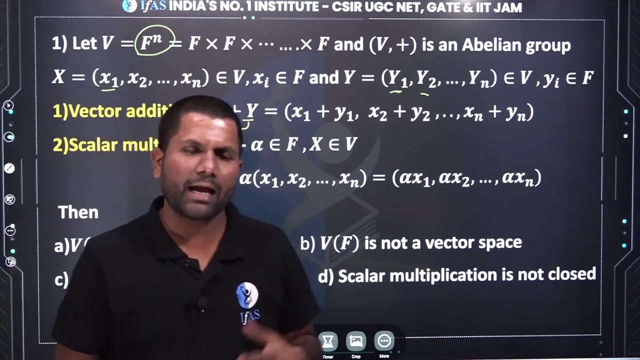 we have taken a field. ok, almost everyone is giving a answer. ok, now look, tell me first one thing: why I have vector addition closed. first tell me once: here is vector addition closed? vector addition close means what happens, that you are a from where it is from, and means 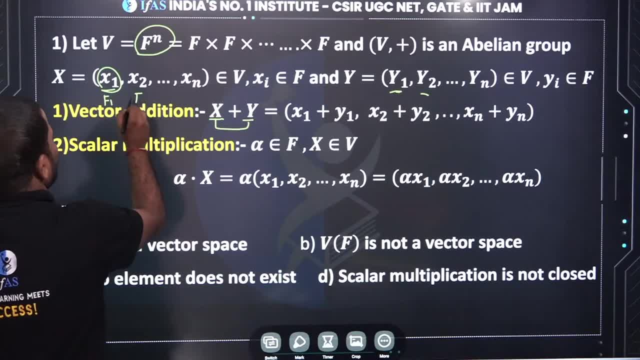 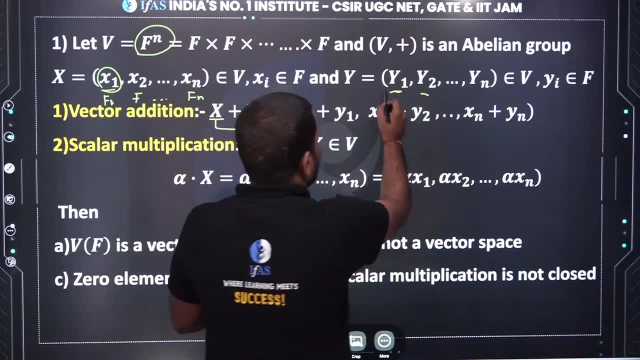 a is in element fn, a is in element fn. in F. A is belonging to F, A is belonging to F. similarly, A is belonging to F. so now our F is field. Where does this element belong? A also belongs to F. it belongs to F. it belongs to A. 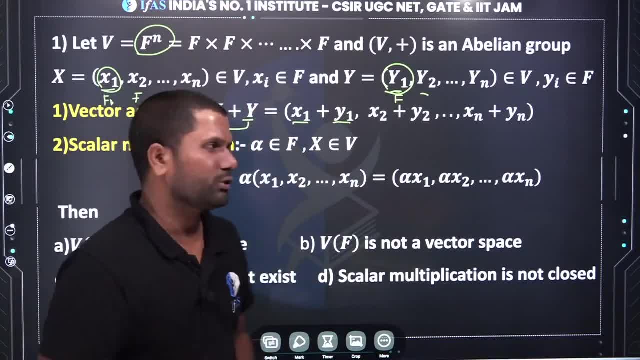 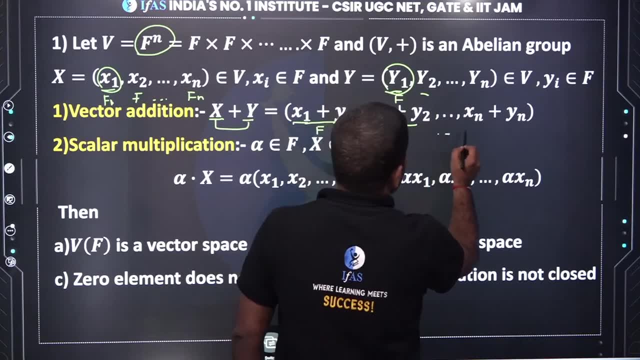 F is your field. in the field, the addition is closed, which means that when you add them, it will belong to F. when you add it, it will belong to F. similarly, when you add this, it will belong to F. 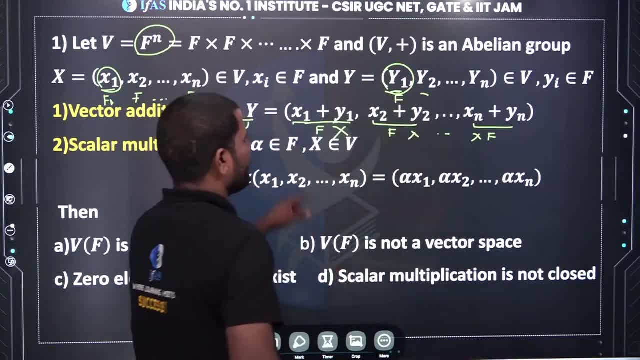 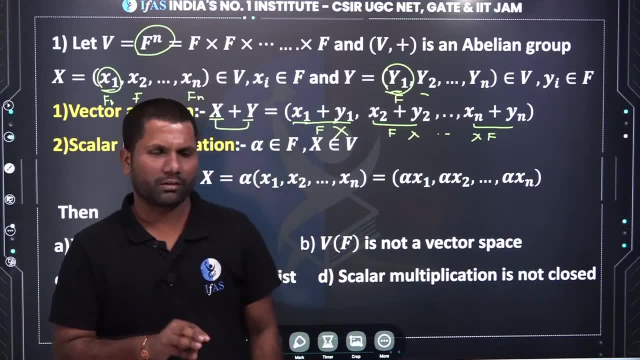 it means that it will belong to F. now we have seen before that F is belonging to theniejsze one. it will belong to F. this means that from here you can see what is vector addition here Closed. See, you have got a vector addition close. now if the vector 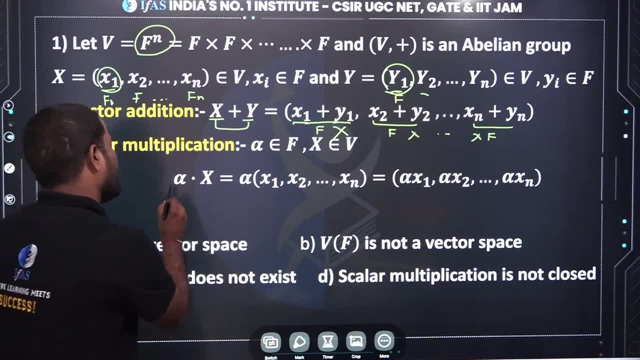 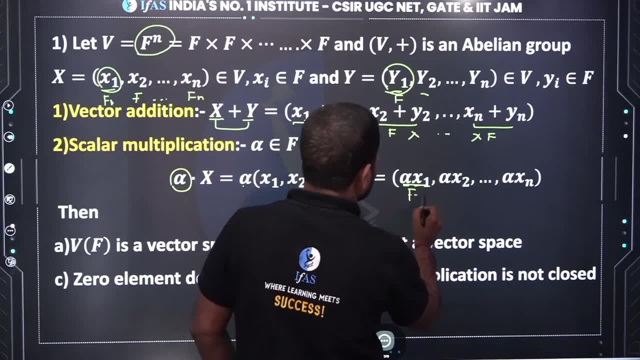 Addition is close. so next we are going to see what is scalar multiplication. so it is the Indiana element of alpha. is it the element of field? now? Now see alpha. see, this is the Blooda element of a Representatives of the field. multiply it again and multiply it again. then again, the 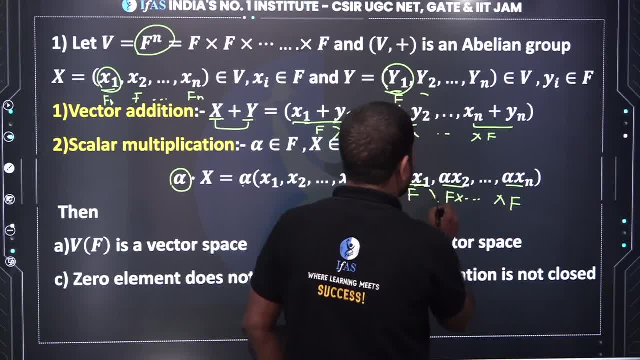 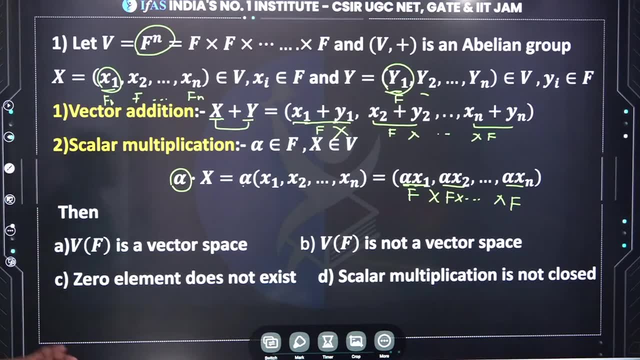 if you multiply the last, then again it is in the field. so overall it belongs to where overall it belongs to fn. so from here we are getting to know that vector addition and scalar multiplication both are closed. so it is saying that scalar multiplication is not closed. 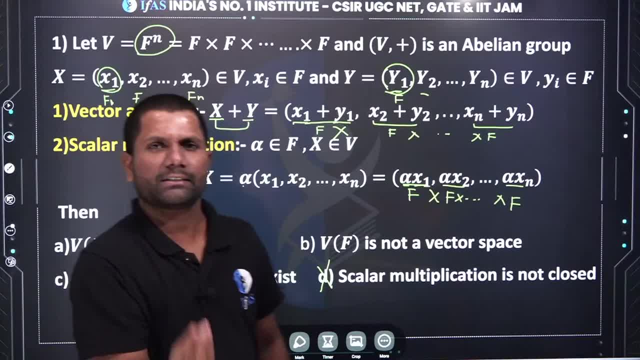 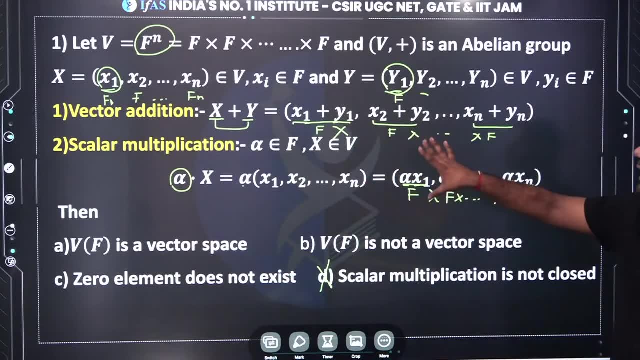 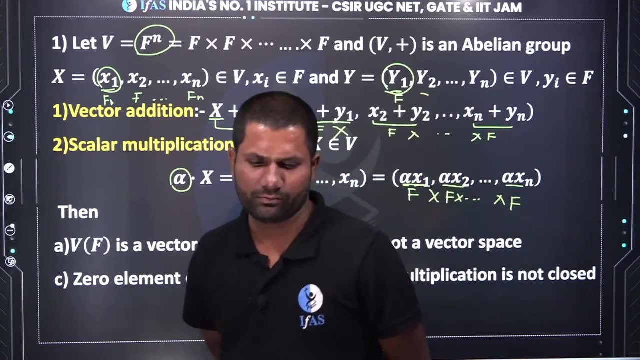 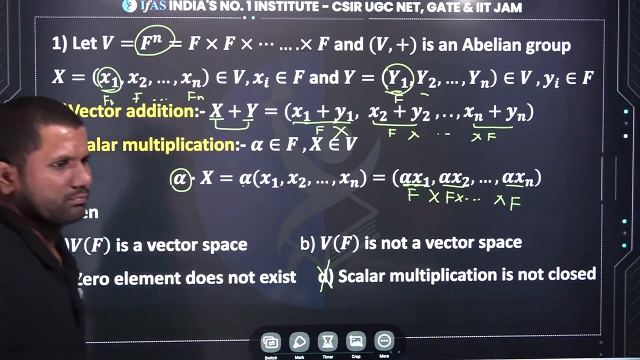 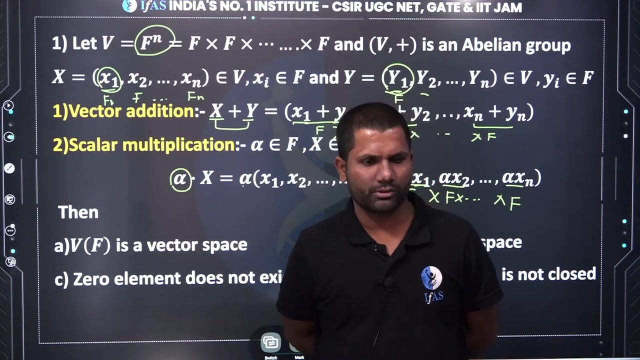 it is incorrect. so two properties of start- vector addition and scalar multiplication- are closed. we have verified it. did you understand that vector addition and scalar multiplication are closed? see, did you understand till here now we will move ahead. now we will check its one by one properties. associative property will satisfy. 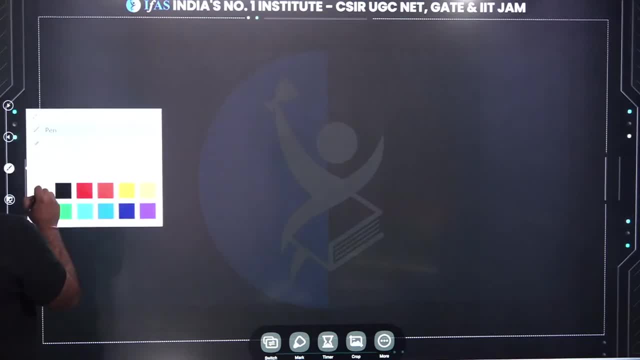 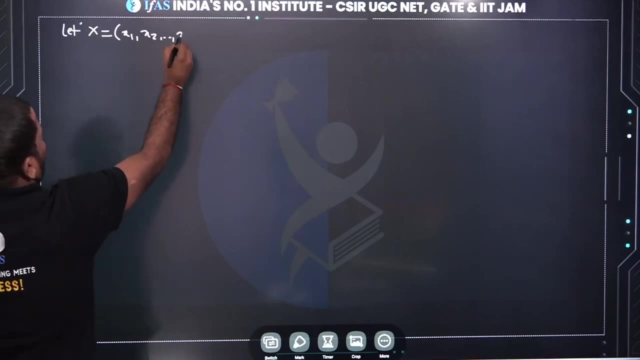 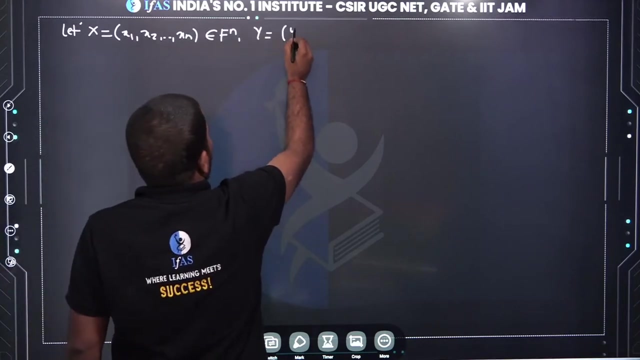 first property, what you have to tell, first property you have to tell: take any element, let me take it again and again. suppose I take let x equal to x, equal to say x1, x2 and so on. xn, which you will see where it belongs. it belongs to fn. 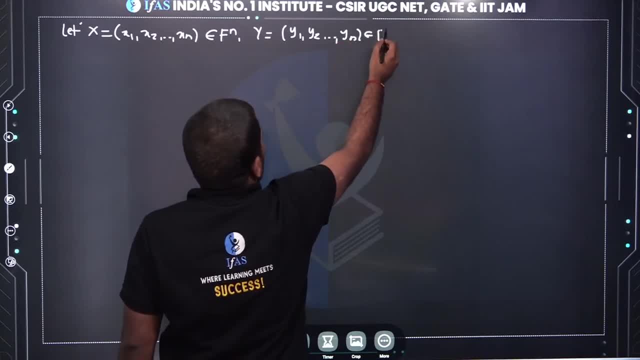 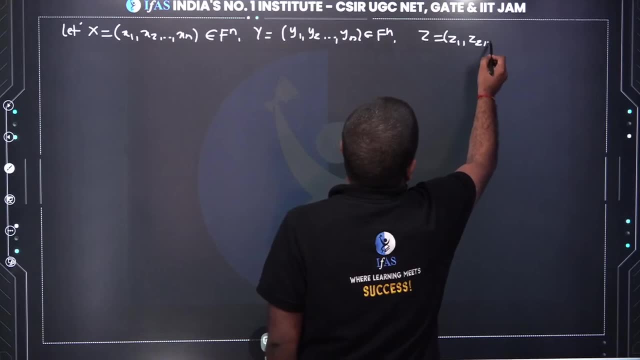 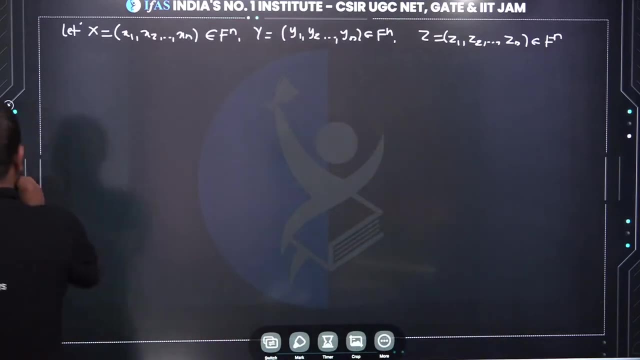 and y, we took y1, y2 and so on. yn, we took it belongs to fn, and here we took z. z is equal to z1, z2 and so on. and where does a belongs? it belongs to fn. now, what does the first property say? if you see the first property, 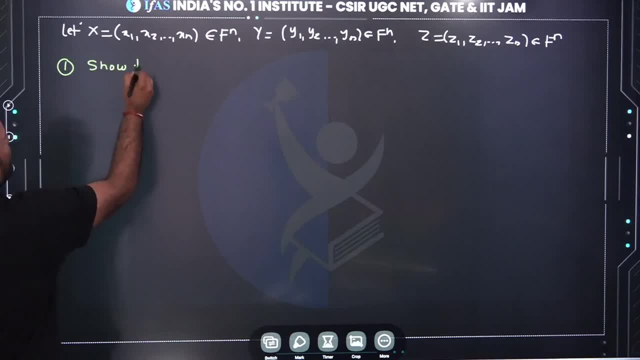 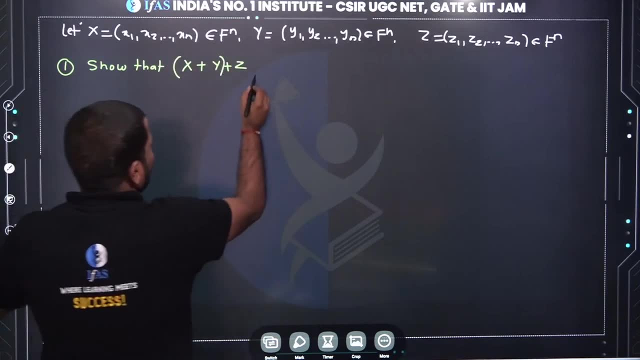 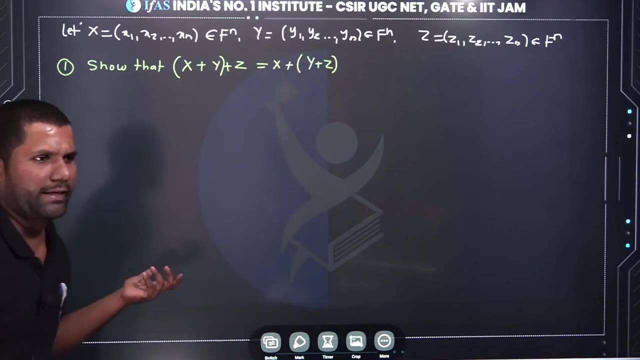 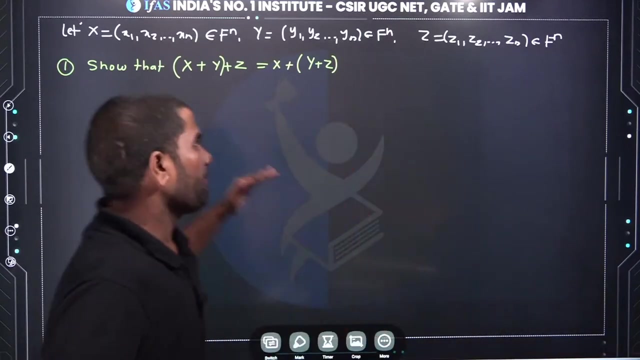 what is it first you have to show, so that x plus y plus z. first add x plus y, then you add y plus z first, then add it with x. both should be same, so you can verify it easily. first property: you can verify first property. here is x, here is y. 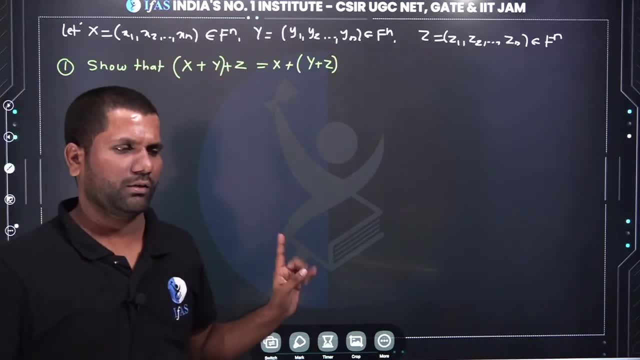 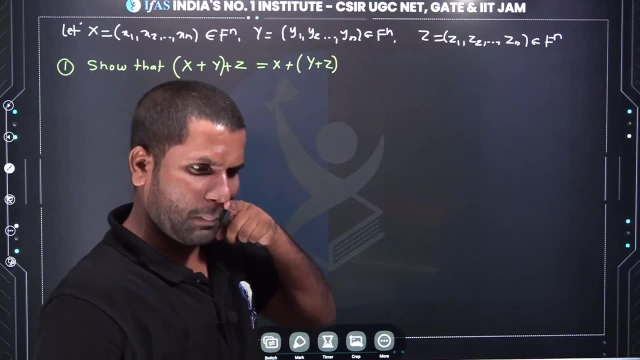 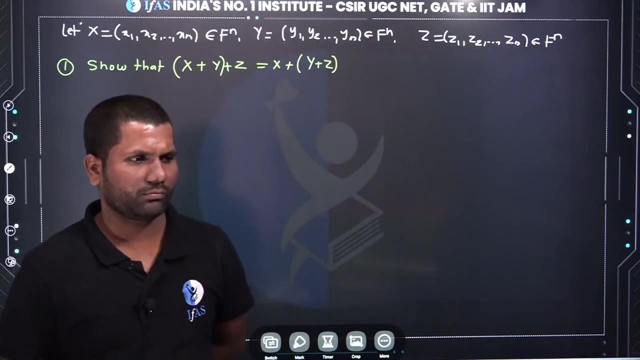 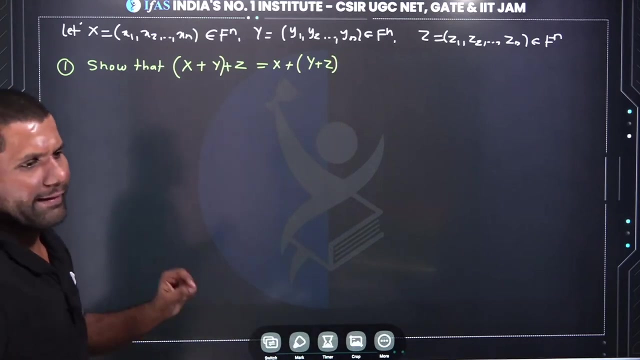 here is z first property everyone can verify. I don't think there will be any problem in first. you can do first see, see. can you verify first property easily? can you verify first property easily? can you verify first property easily? ok, do one thing: start with lhs. lhs is equal to rhs. 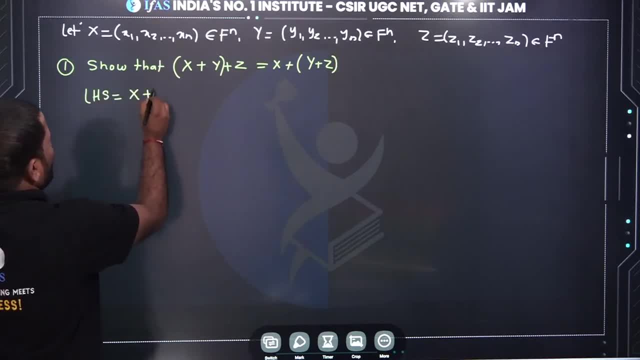 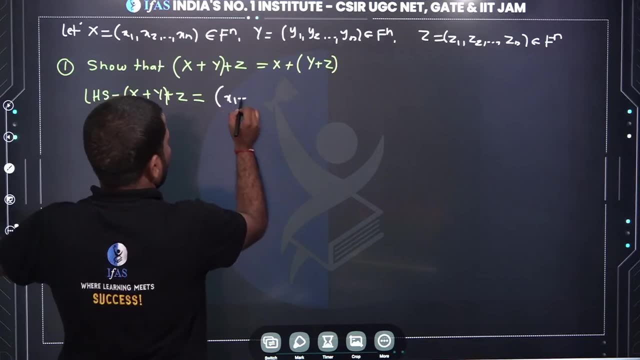 if you take lhs, what will you get? you will get x plus y plus z. so what is your x? x is equal to x is equal to x1 comma x2, x1 comma x2, and so on. xn is given plus y1 comma y2. 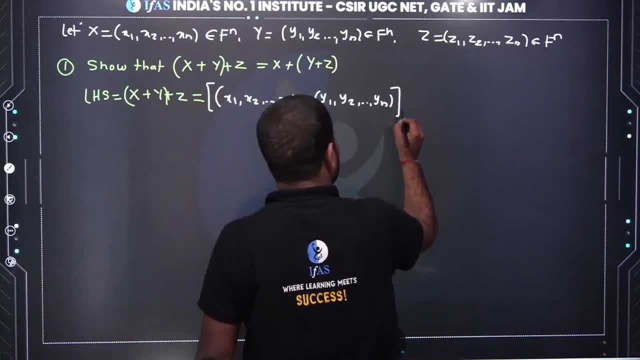 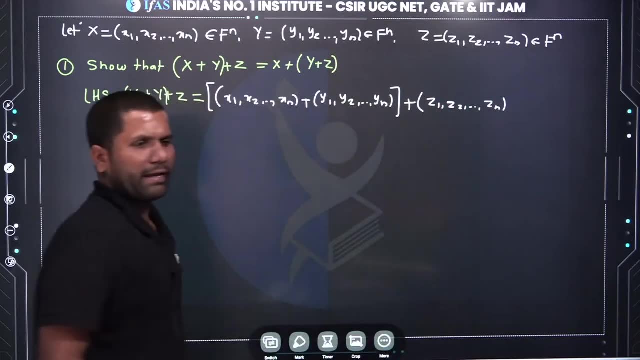 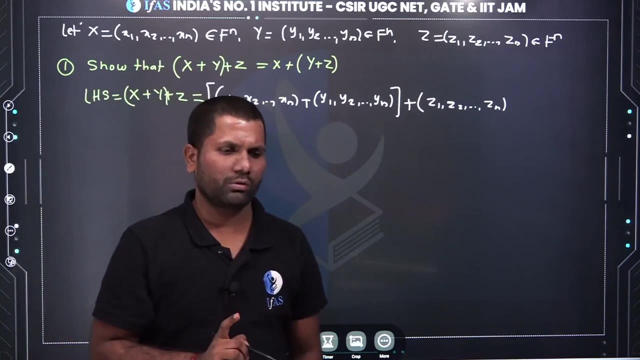 and so on. yn is given. with whom to add plus z. you have to add it like this: ok, I think you can verify it easily. I think you can verify it easily. I will leave this homework for you. if no one can do it, then you tell me, I will solve it. 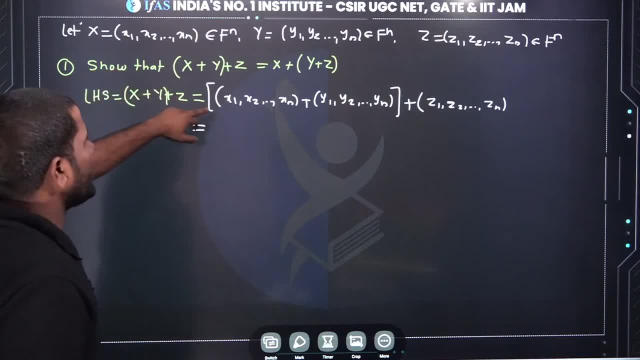 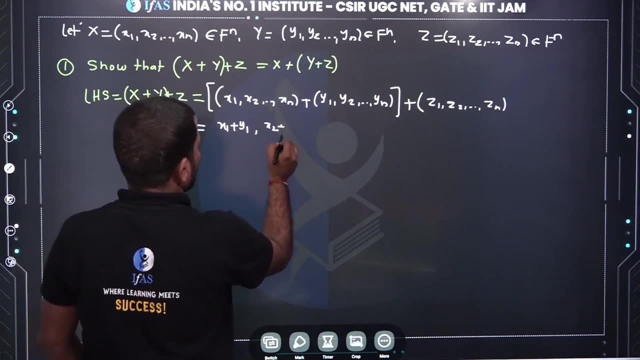 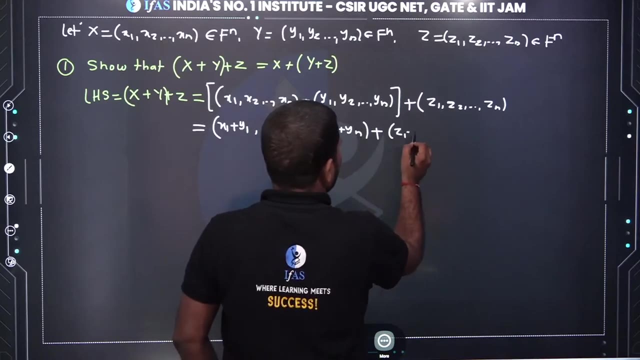 this is the first property. lhs is equal to rhs. start from here and solve it. you can write it like this: x1 plus y1, x2 plus y2, and so on. xn is given plus what will be here. z1 comma, z2, z1 comma. 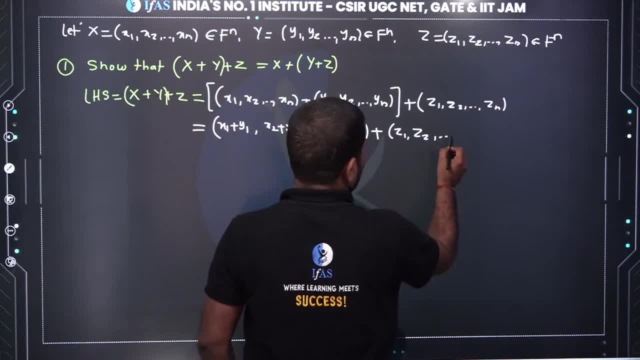 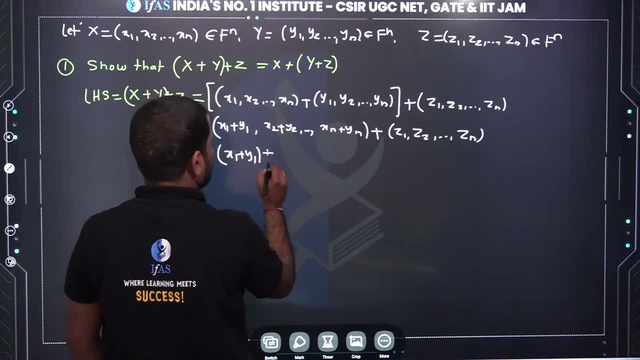 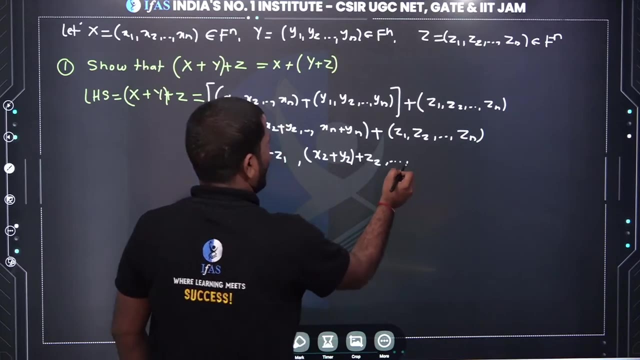 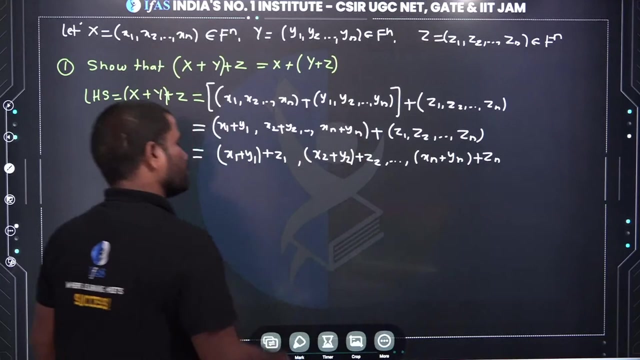 z2, z1 comma, z2 and so on. what will you get? x1 plus y1 bracket plus z1, x2 plus y2 bracket plus z2, and so on, plus xn plus yn plus Zn. so you can write it like this: how can you write it? you can write it like this: 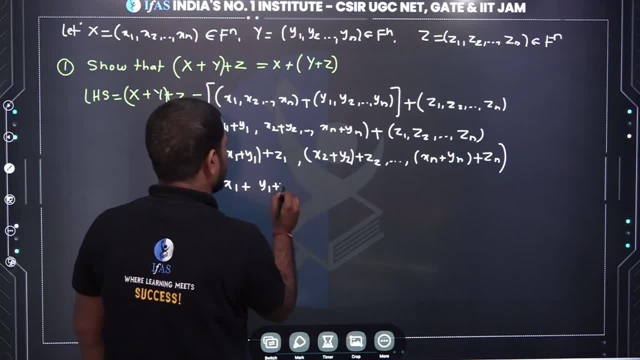 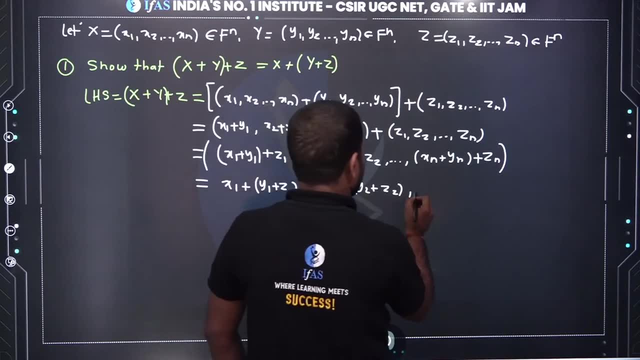 here, for example: x1 plus y1 plus Z1. you can do this comma: x2 plus y2 plus Z2. you can do this plus, and so on. you can write it like this: xn plus yn plus Zn. you can write it like this: ok. 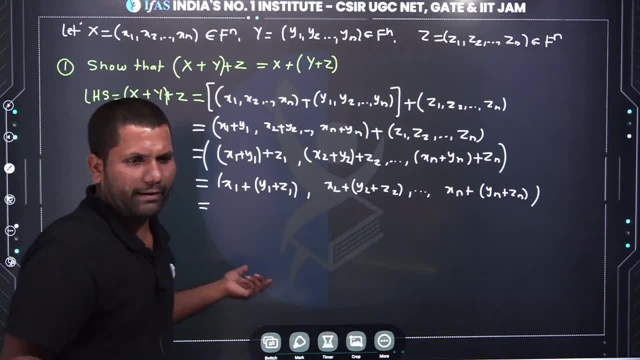 so what will you get? if you simplify it once, divide it into two pieces, you will get n tuples in all three. yes, we are taking n tuples. ok, don't do it. ok, do it. so let's do it here now. you have written it like this: 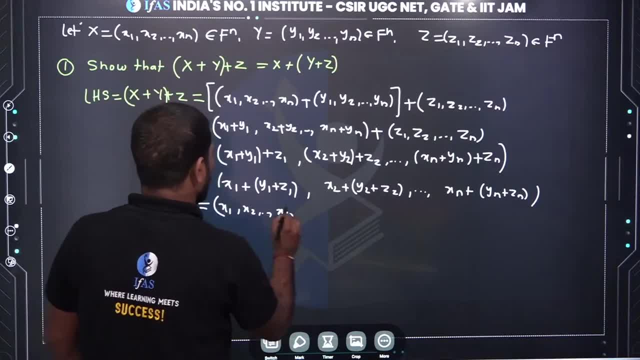 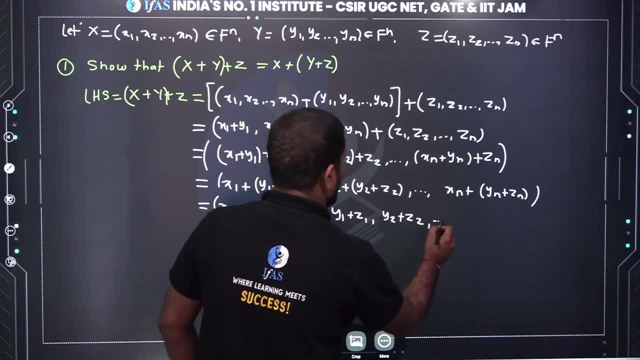 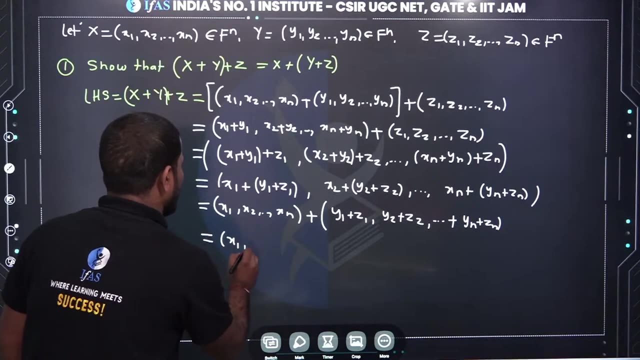 now what I will do. I can write it like this: x1 comma x2, and so on: comma xn plus y1 plus Z1, y2 plus Z2, yn plus Zn. so here, if you separate it, what will you get? x1 comma x2, and so on. 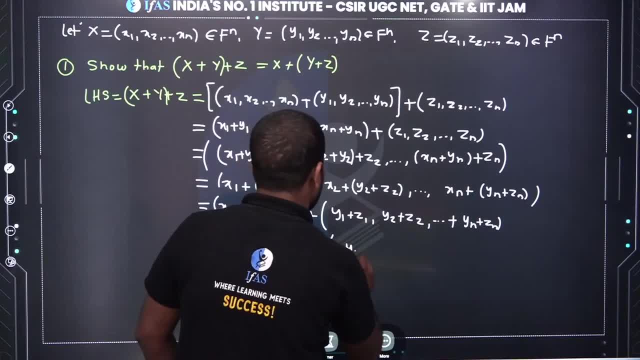 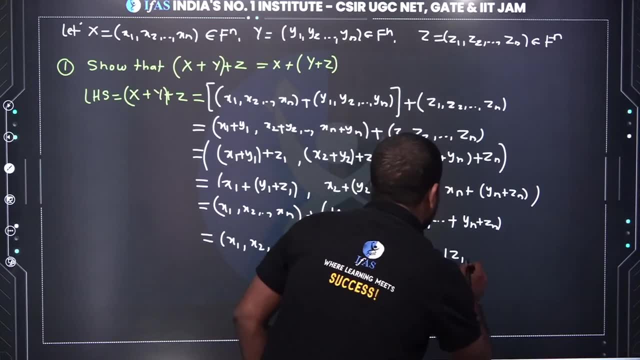 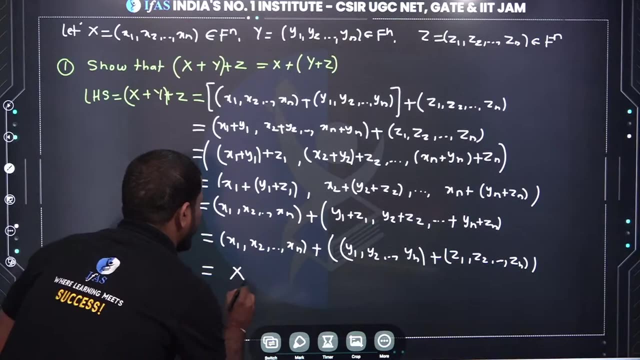 xn plus what will you get? y1 comma y2 and so on, yn plus z1 comma z2 and so on. if you write it like this, so this is equal to x plus y plus Z. this is equal to. this means the first property is satisfied. 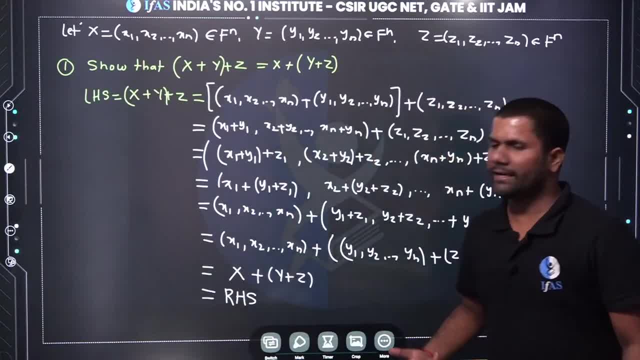 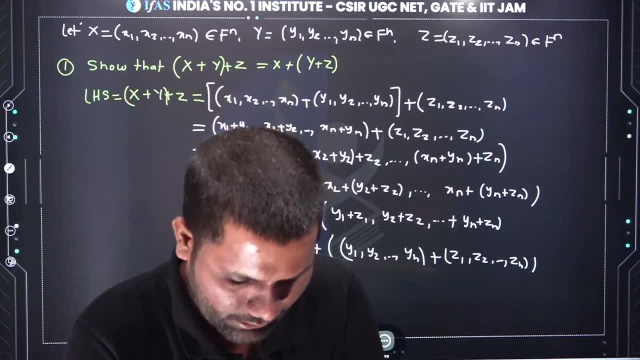 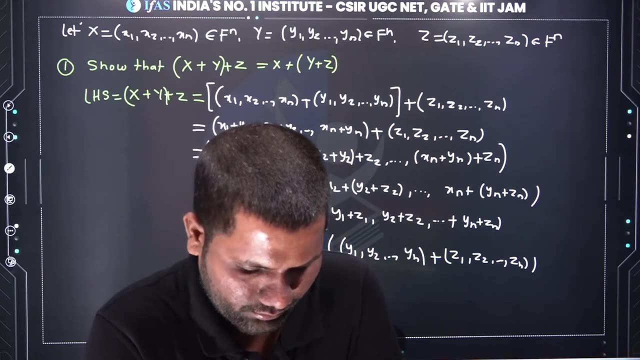 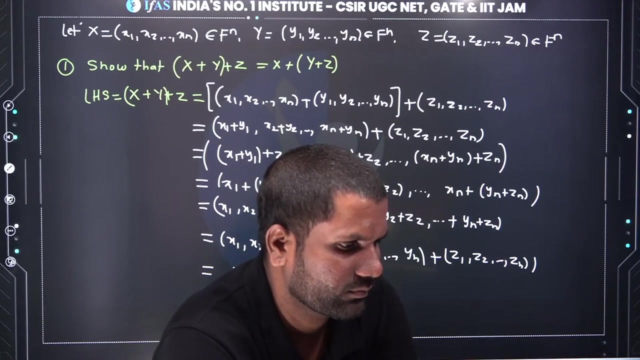 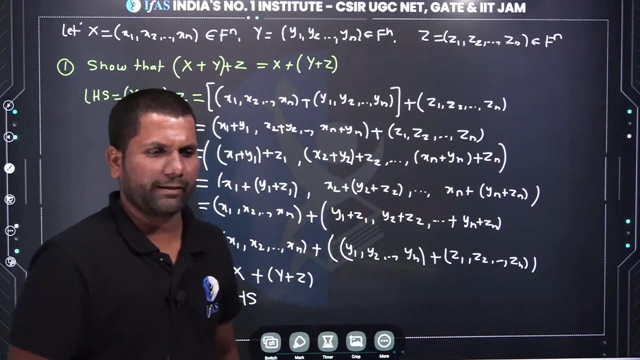 the addition given to you. what will be the addition n tuples? is it clear? I hope it is clear. if you have any doubt, then you can ask. ok, everyone understood. ok, ok, so let's move ahead. so the first condition is satisfied. second, what we need here: 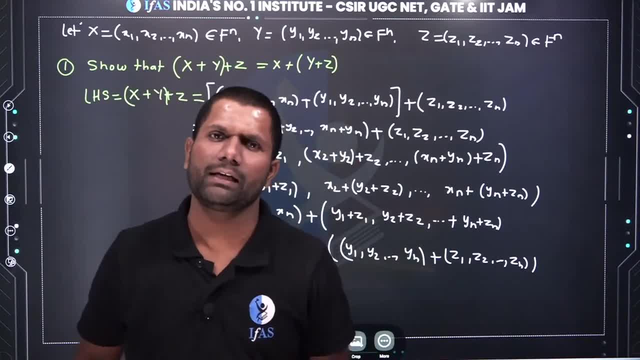 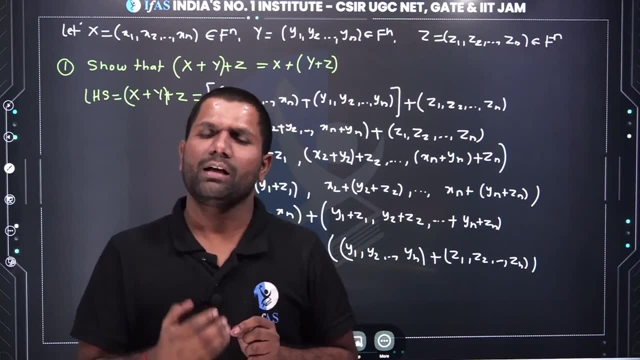 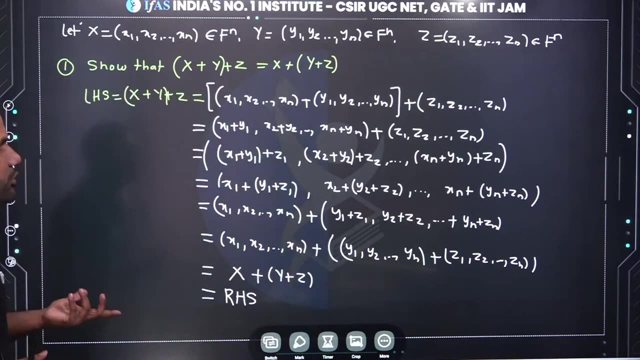 we need the addition of identity. so what do you think? what can be the addition of identity? like in R in real number, whatever number you add, you will get 0. similarly, if you write R x, R, x, R x R, what can be the addition of identity? 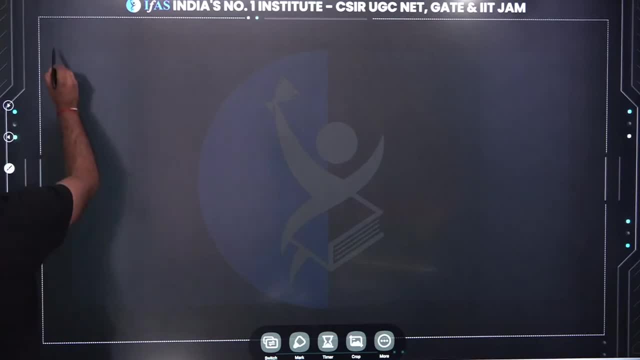 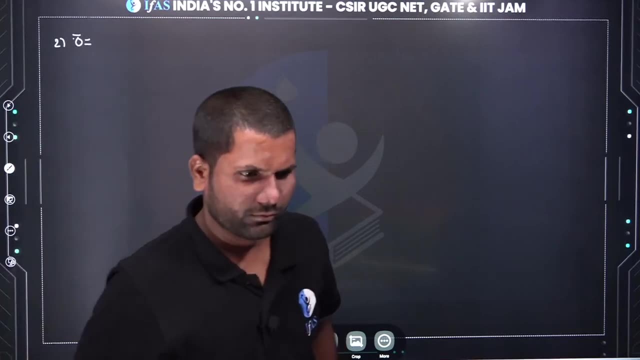 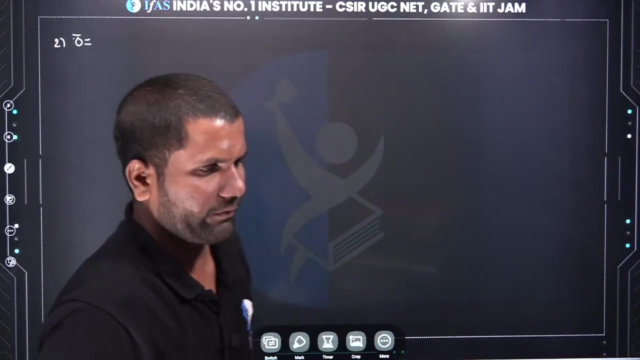 now. second, we talk about identity element. so here identity element means zero vector. so here what will you get? see here. see here: suppose the class will be one hour every morning and one hour in the evening. morning will be at 11 o'clock and evening will be at 6 o'clock. 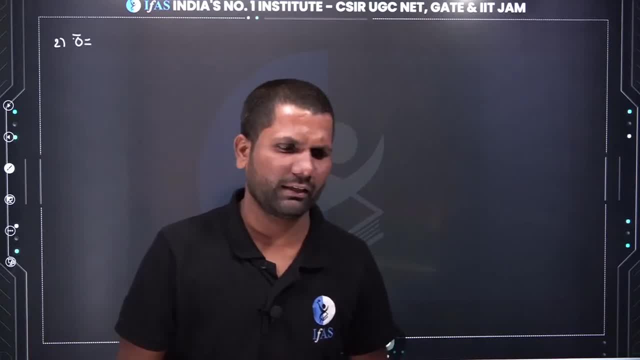 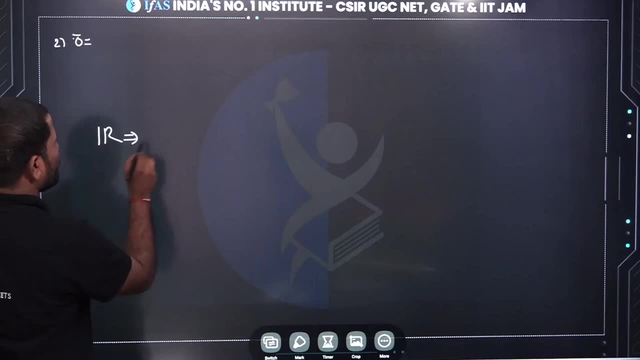 ok, not necessary that one hour. if needed we will extend it a little. see now, if I give you a real number- so here I say there is a real number with whom I add it, then I will get this number. tell me: add with zero if I give R2. 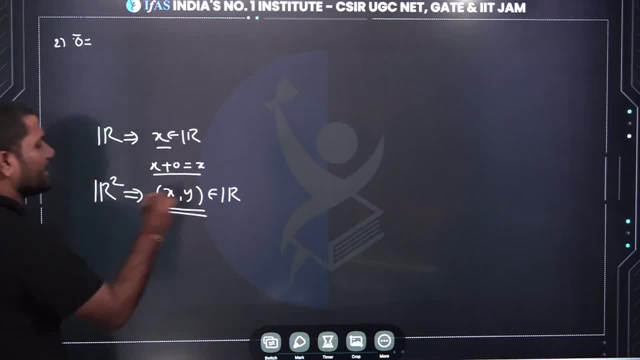 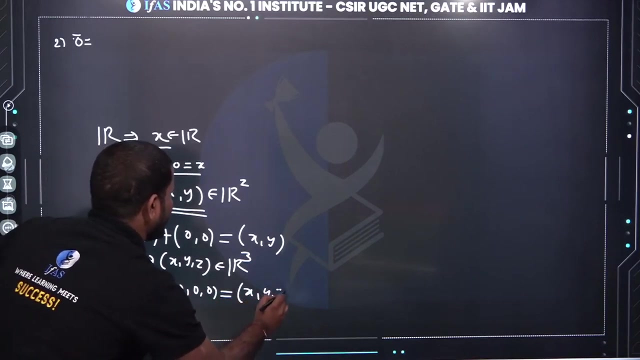 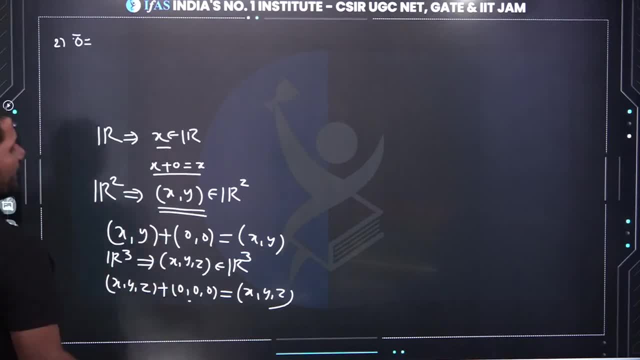 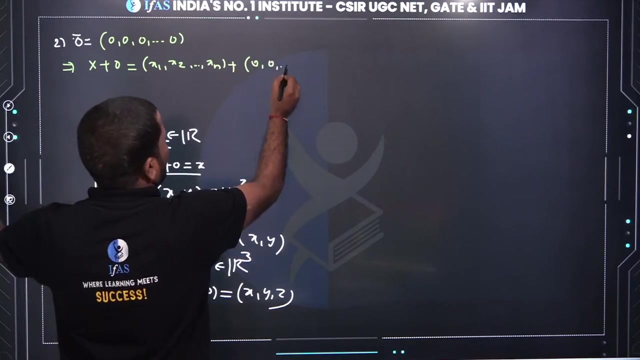 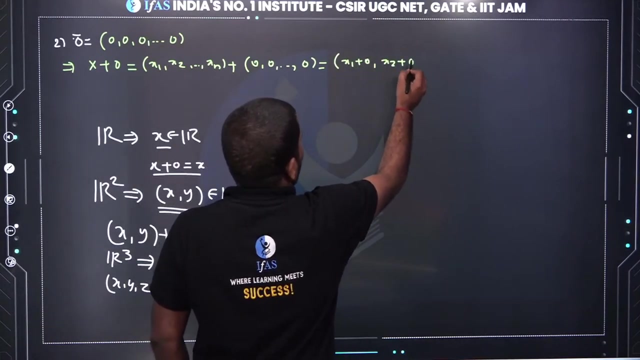 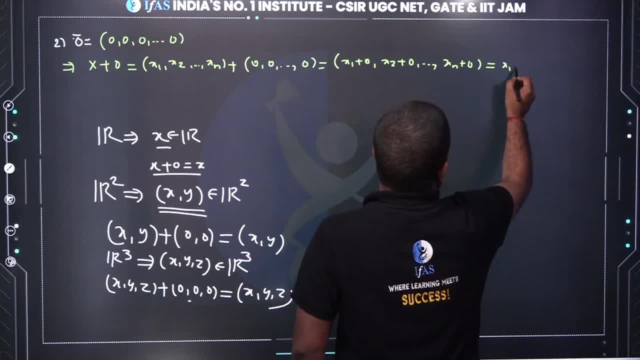 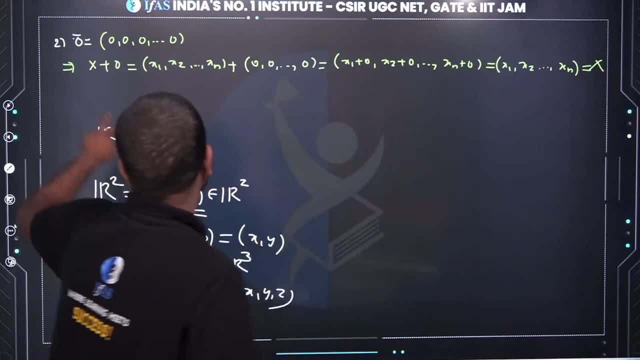 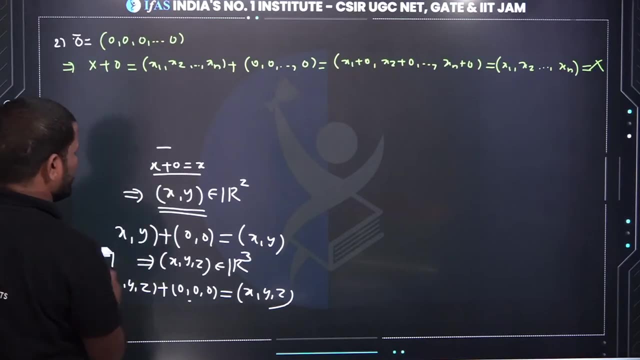 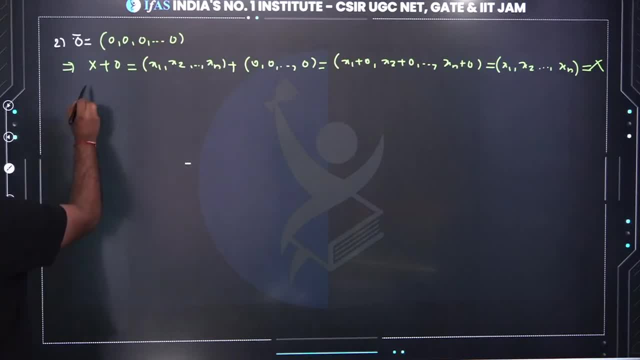 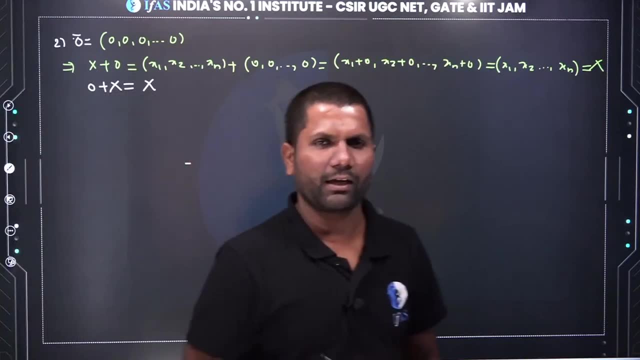 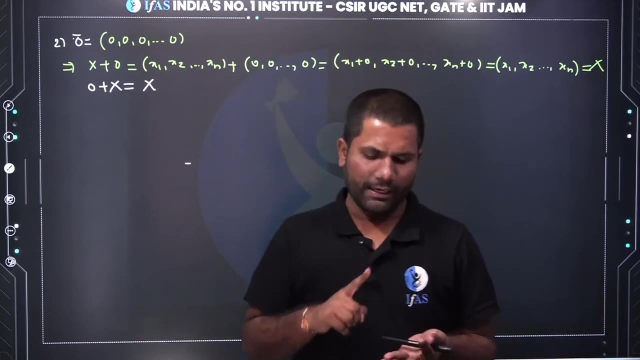 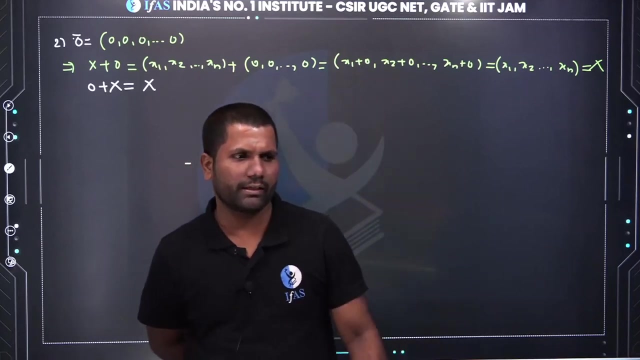 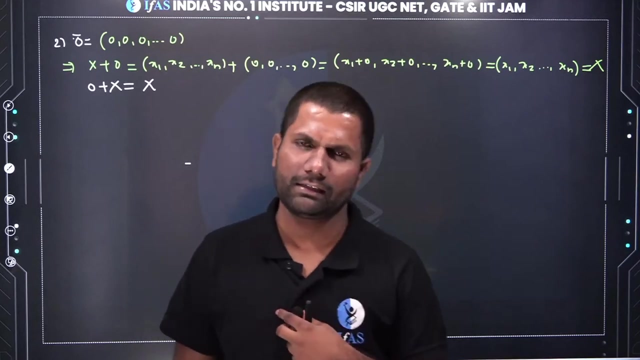 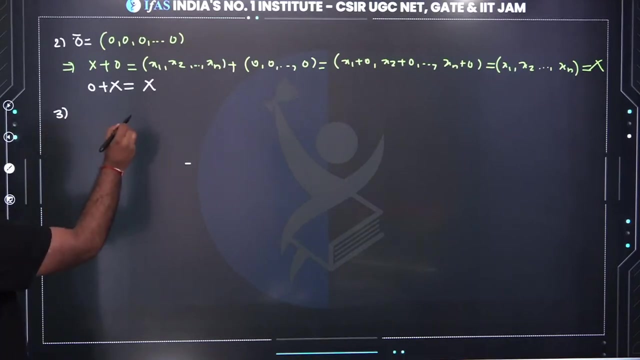 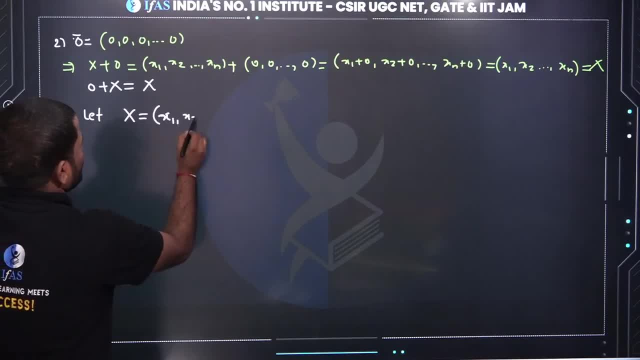 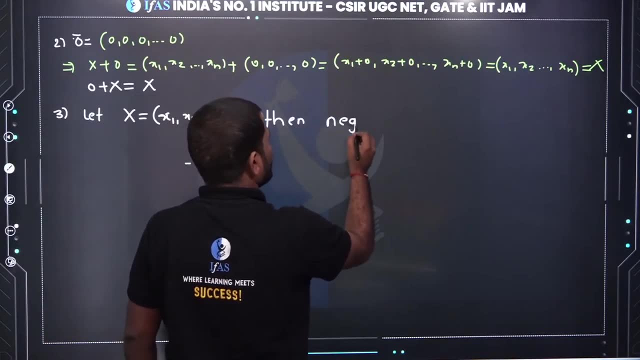 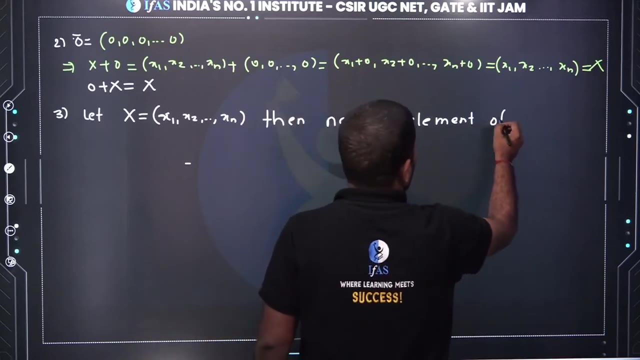 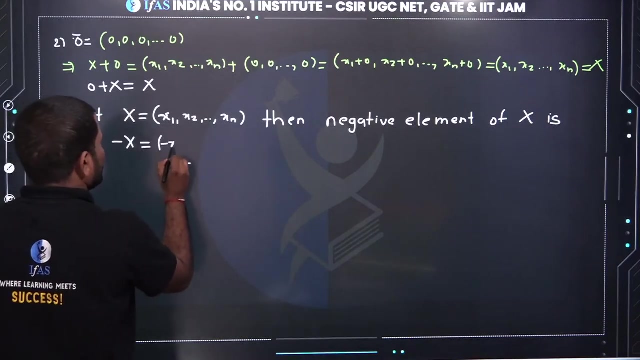 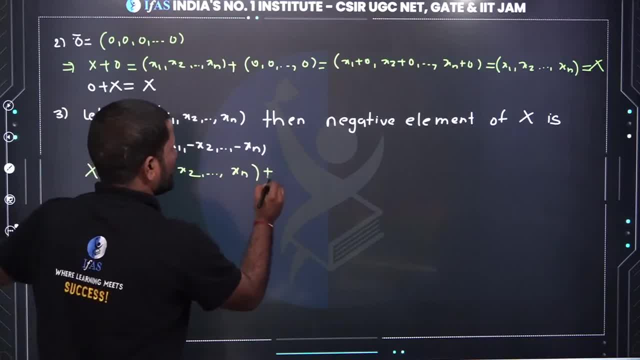 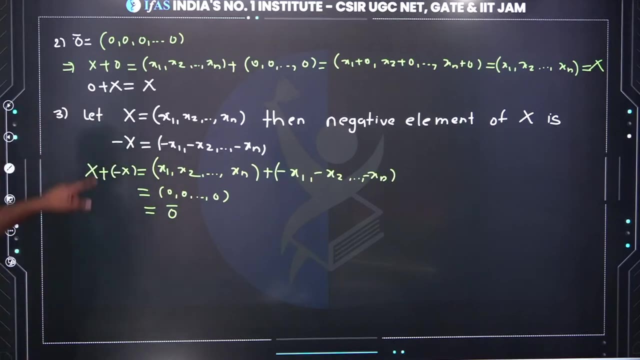 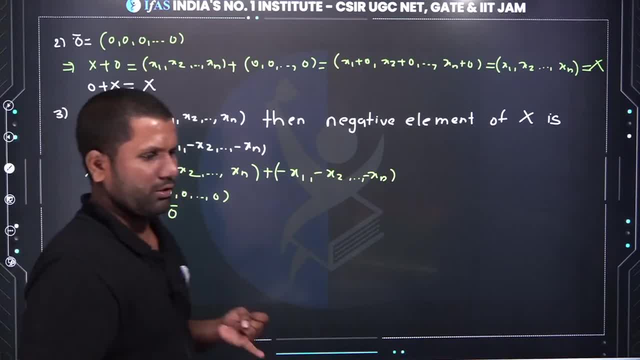 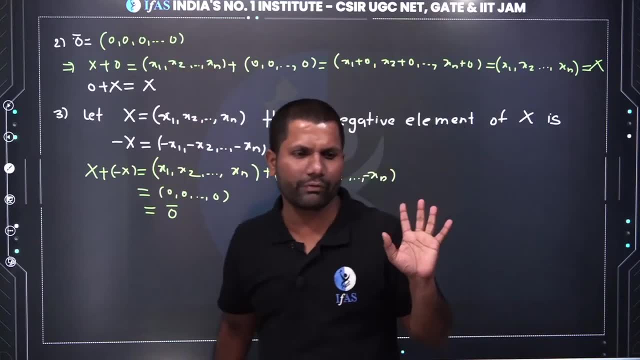 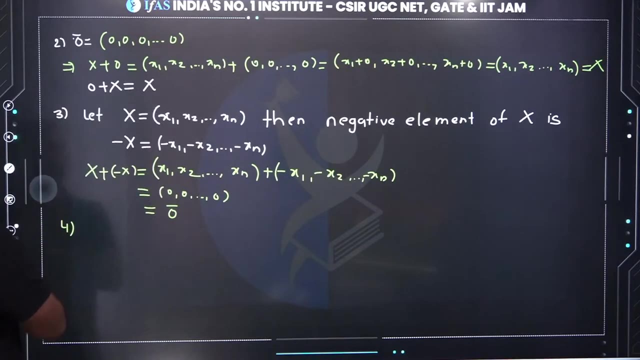 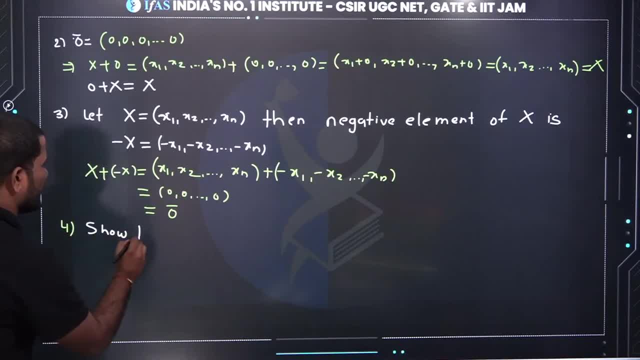 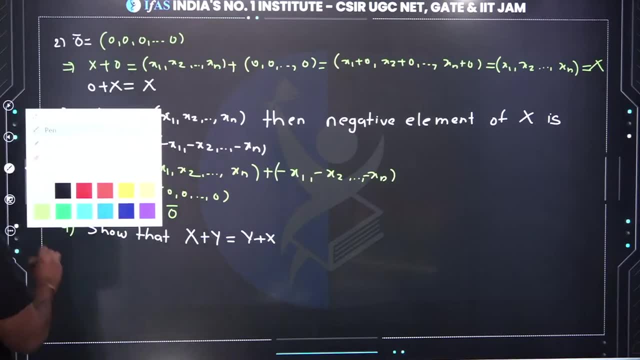 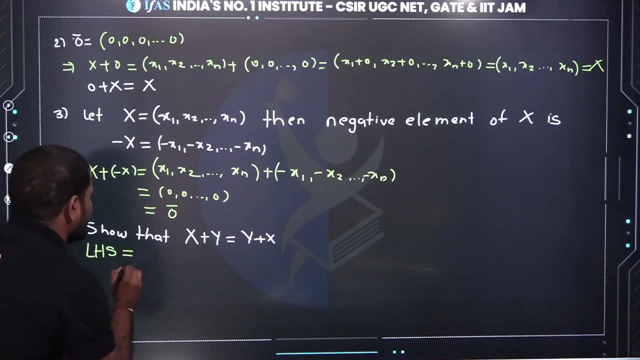 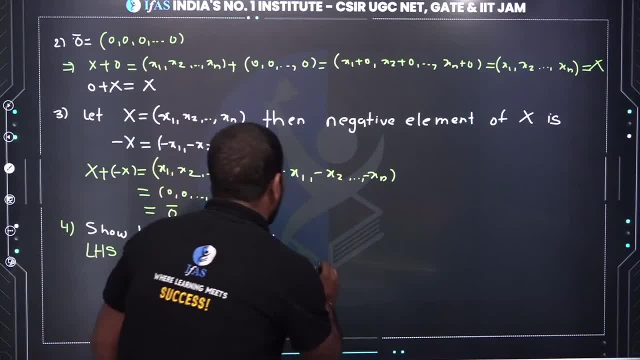 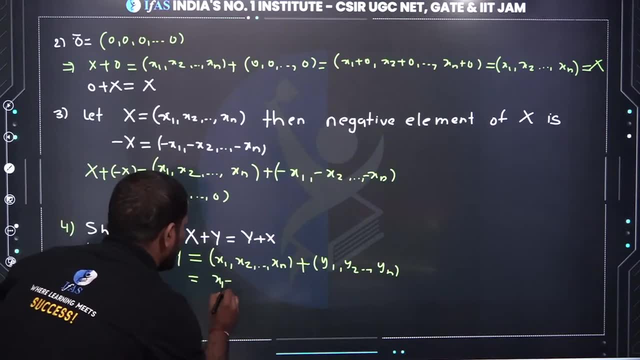 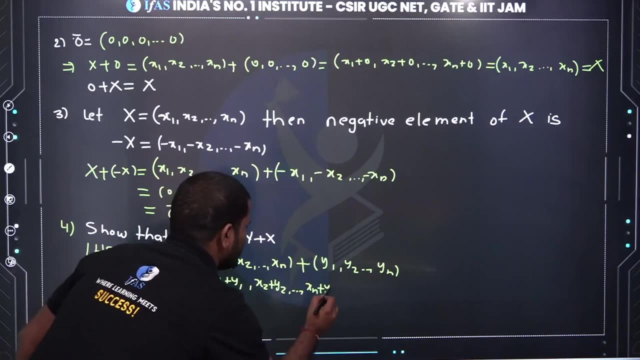 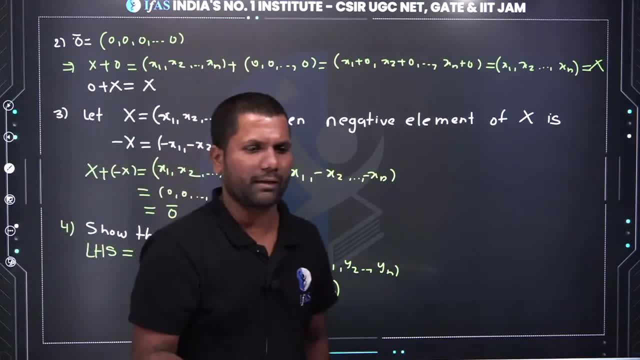 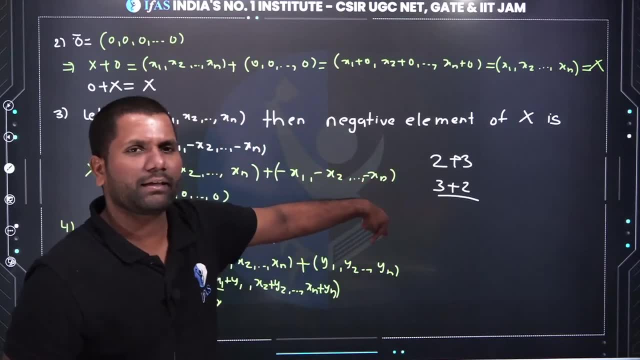 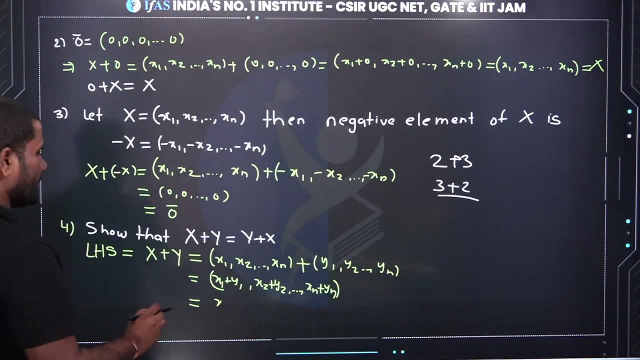 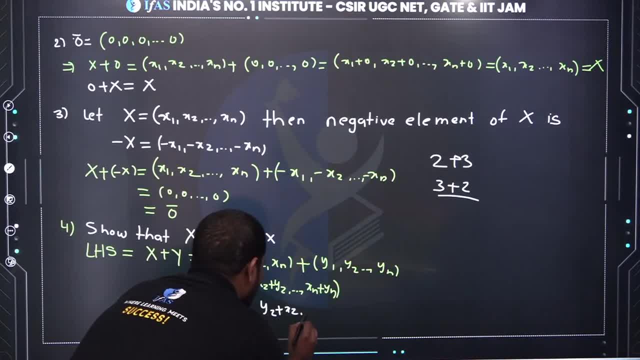 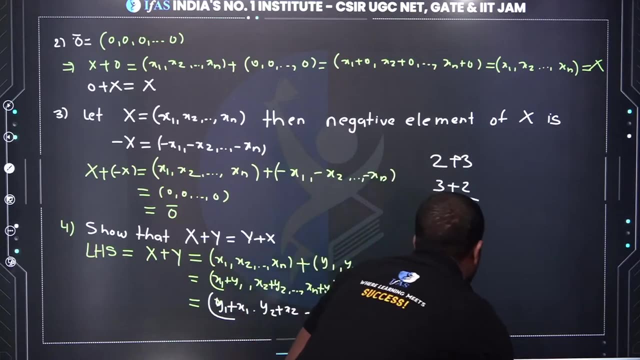 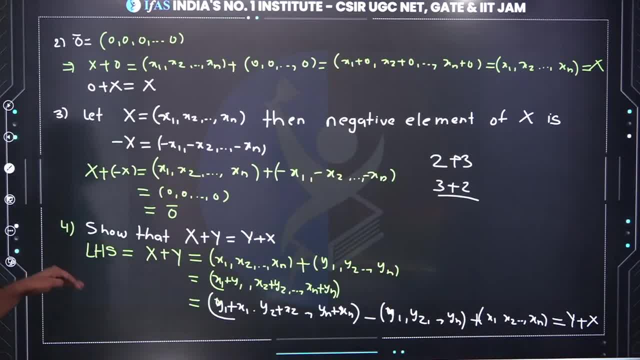 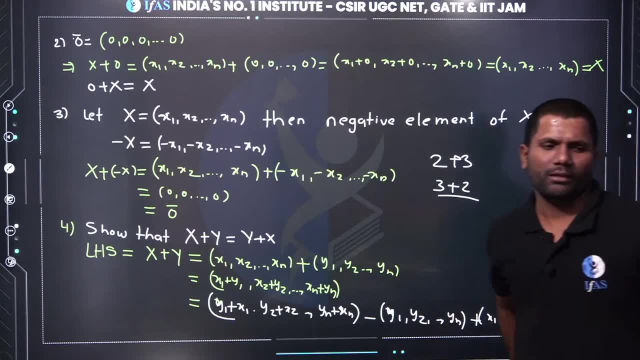 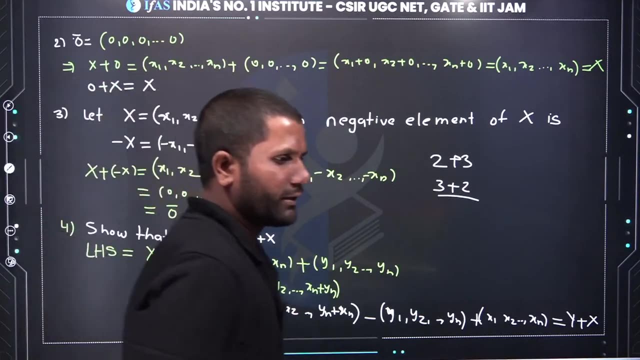 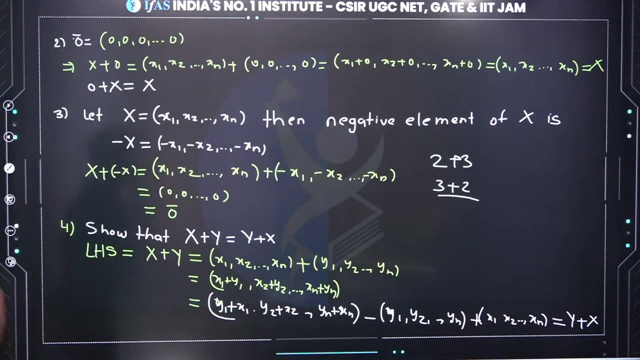 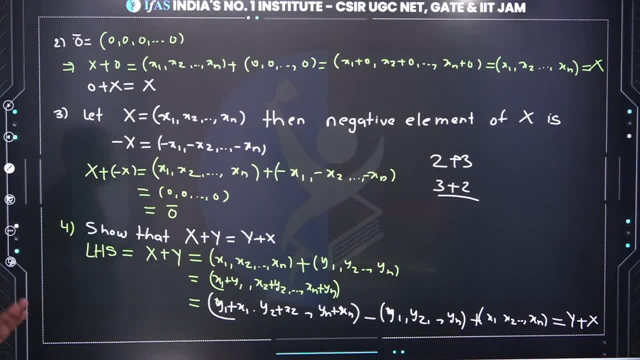 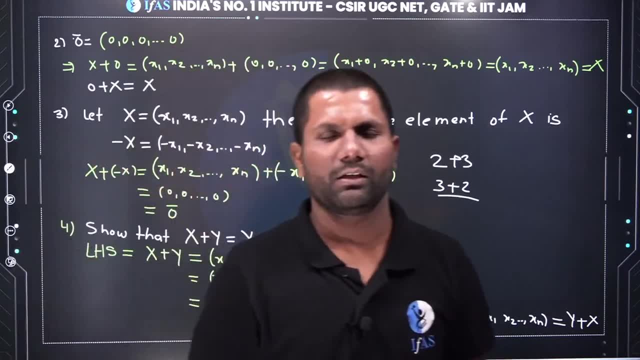 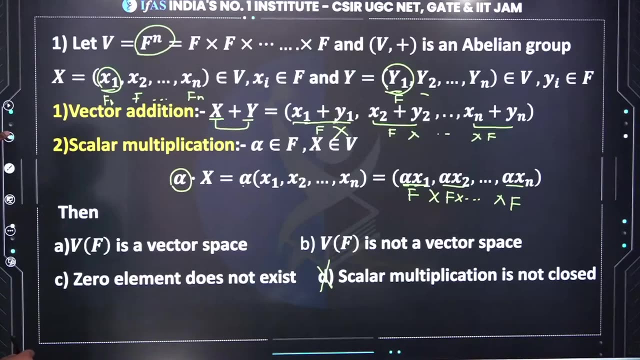 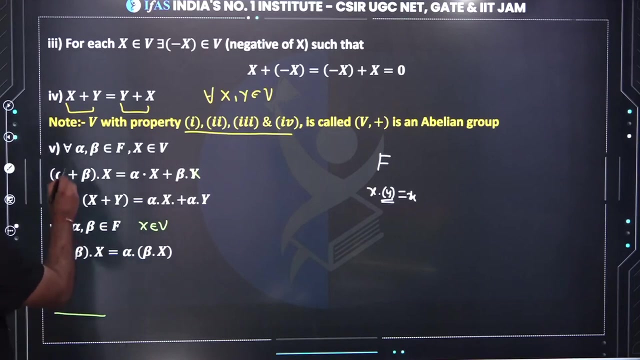 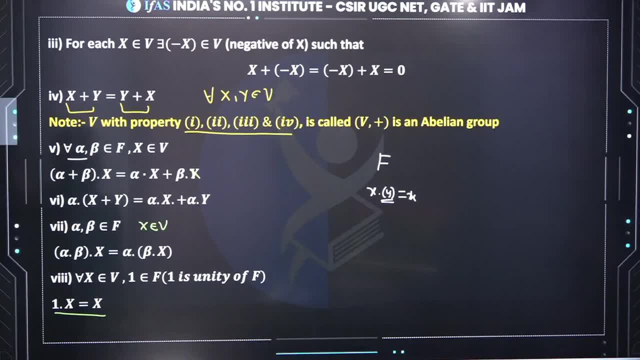 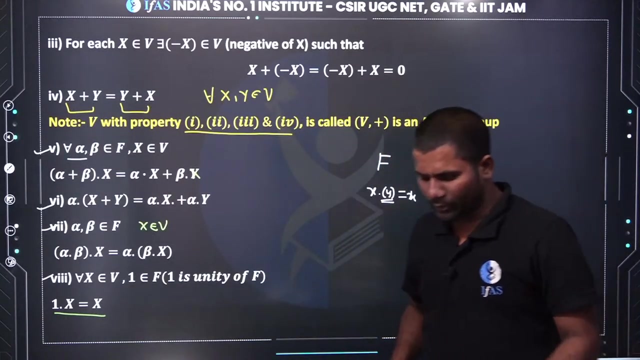 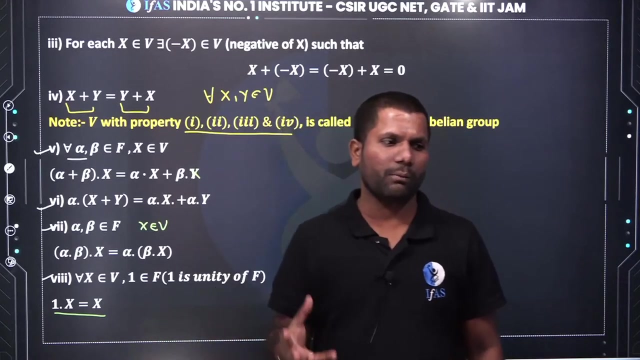 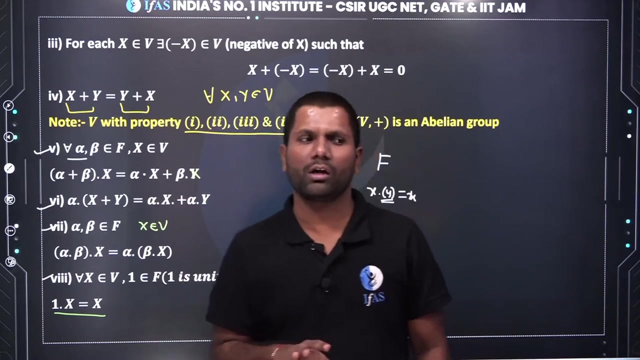 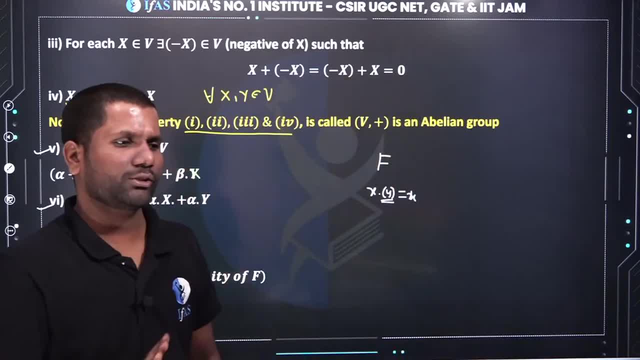 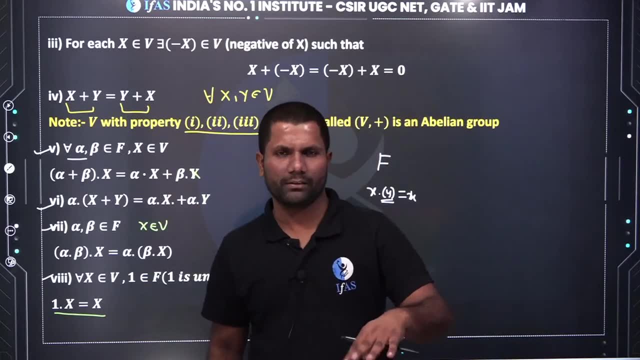 But if there are questions in the exam then you do not have to solve in 10 ways. you will know by looking at the question whether there is vector space or not, For example. if we solve it first, then we will have an infinite number of examples of vector space. 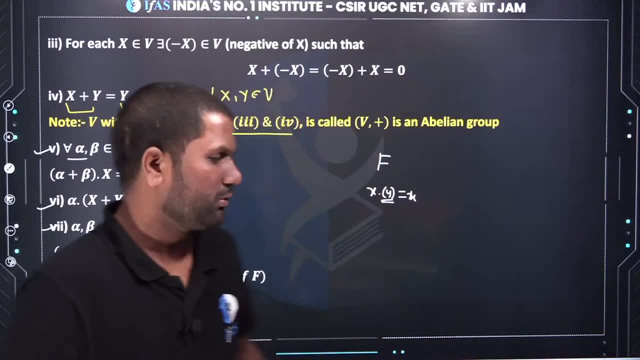 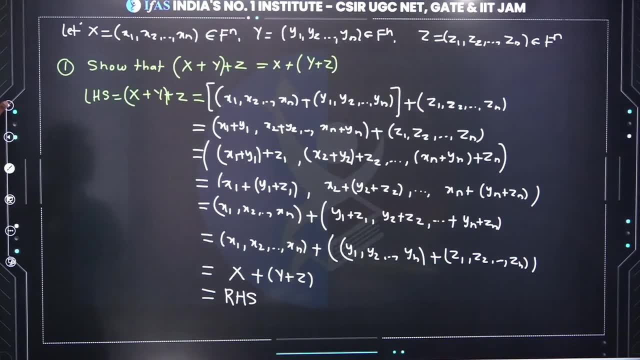 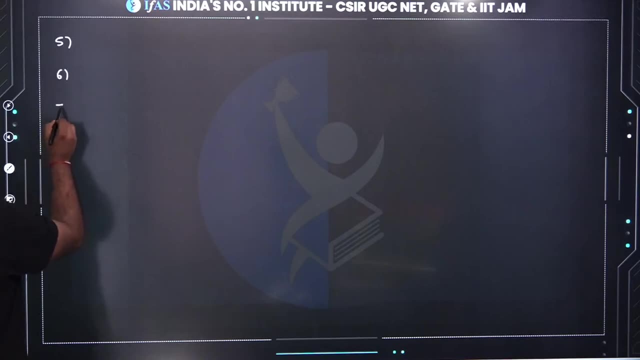 Let's see how. so see here what I do: property number 5,, 6,, 7,, 8, I leave homework for you. See here property number 5,, 6,, 7 and 8,. if you see here, 1.x, what is the value of 1, here it is only 1.. 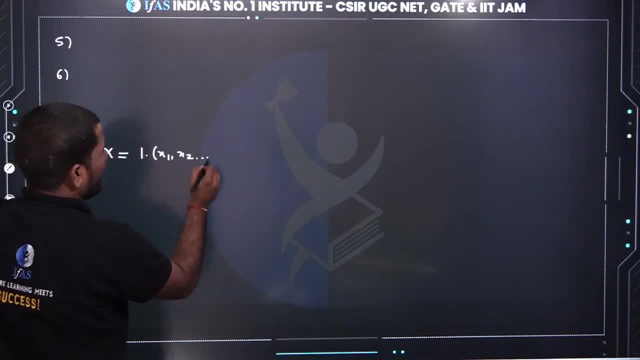 What does dot x mean? x1, x2 and so on. xn will be, which is equal to what will happen: 1 into x1,, 1 into x2, and so on: 1 into xn. so what will you get? 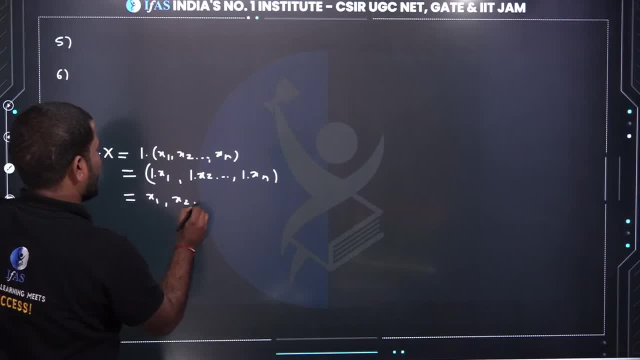 You will get x1,, x2 and so on, xn. so here you can tell that 1.x is same as x. So here, finally, what did you tell? Therefore, all these properties are satisfied. V is a vector space. therefore, V is a vector space over a field F. 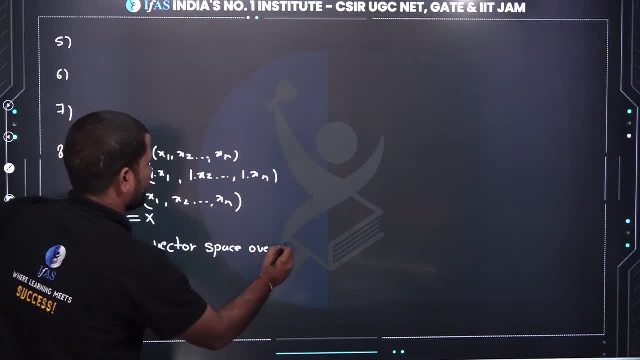 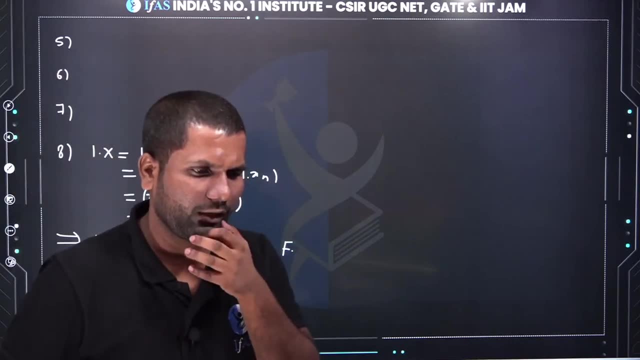 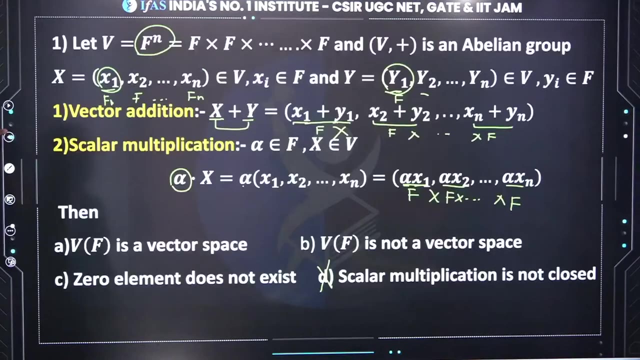 V is a vector space over a field F. So here you know what will happen: Vector space. for whom I am saying this? What is the doubt? Just type it once Now. here you have to keep one thing in mind, Like suppose you have seen here. 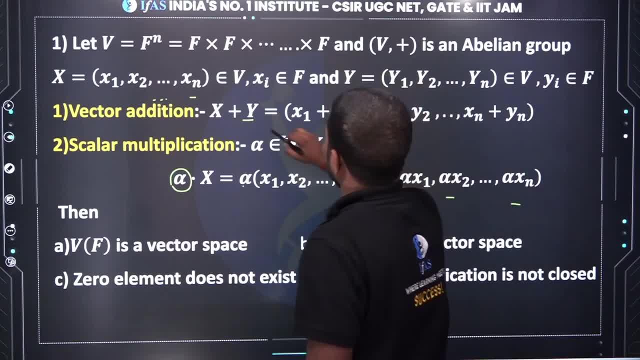 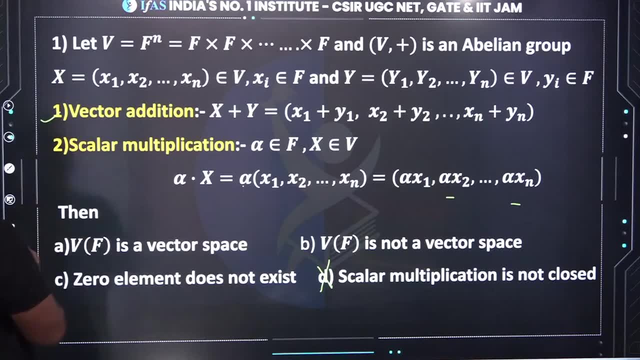 Now, what are you seeing Till now? you know this. now there are 4-5 types of operations of it you have to keep in mind. See now here. we know that if you have given vector addition A, scalar multiplication A. 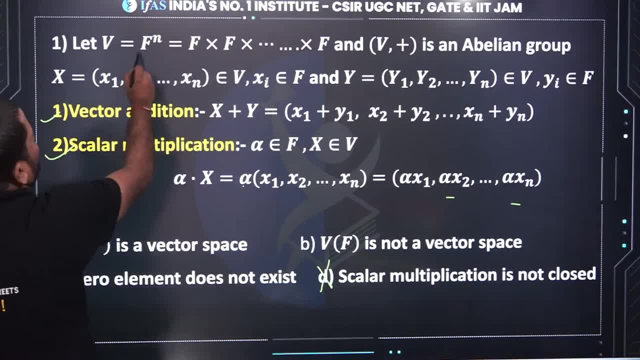 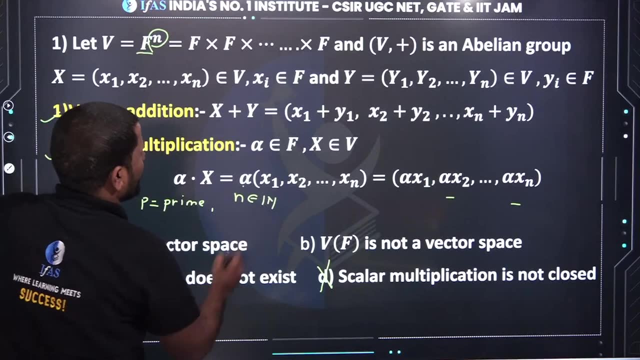 Vector. addition is this: scalar multiplication is this. Field can be anything. Field can be your real number, rational number or complex number, or ZP, where P is a prime. Field can be anything from this And the value of n, n can be anything, any natural number. 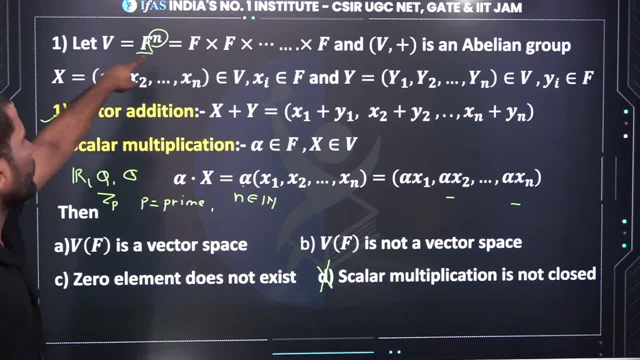 1,, 2,, 3,, 4,, 5,, 6,, 7, take anything, Anything in this. If you have infinite field, then you can keep infinite field instead of F. Keep any field. So what will it always do? 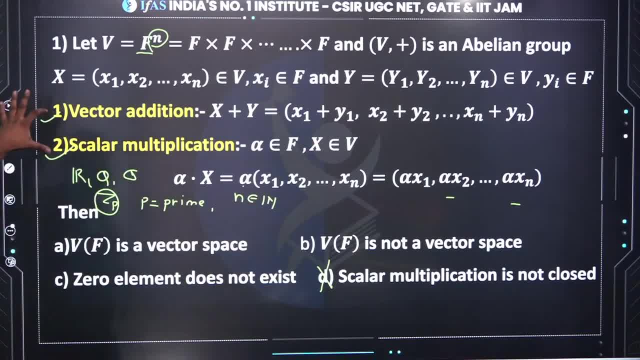 Vector space will form. What should happen to you? These two operations should be known. Whatever will be Fn, always, if your vector addition is given, component wise, scalar multiplication is given in this way, then what will it always do? It will definitely form a vector space. 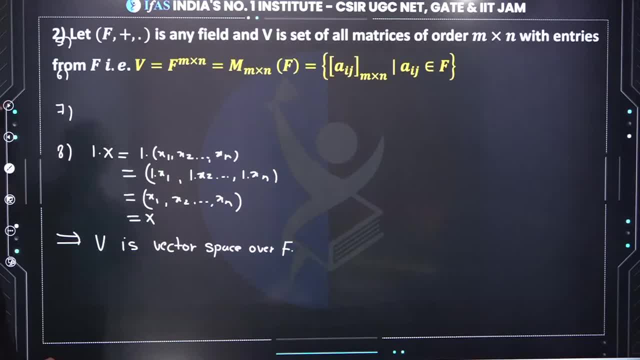 Like, for example: now I keep the operation same. Like, suppose, what did I give here? Did I write on this? What, Wait, wait, wait, This is fine, It was empty. I wrote like this: No problem. Now see here, for example, what did I give? 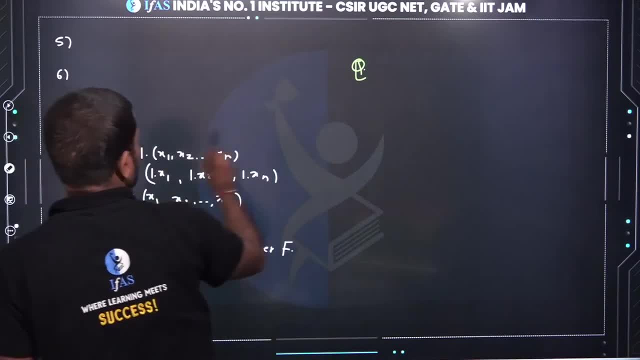 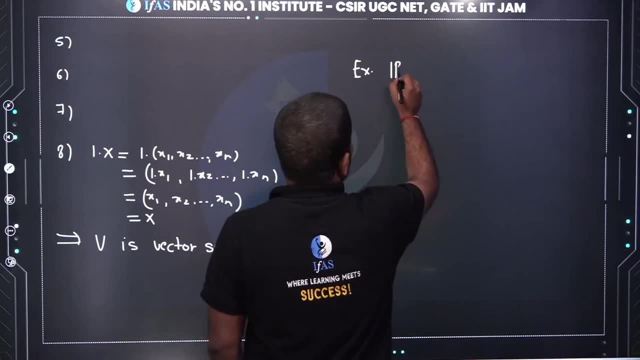 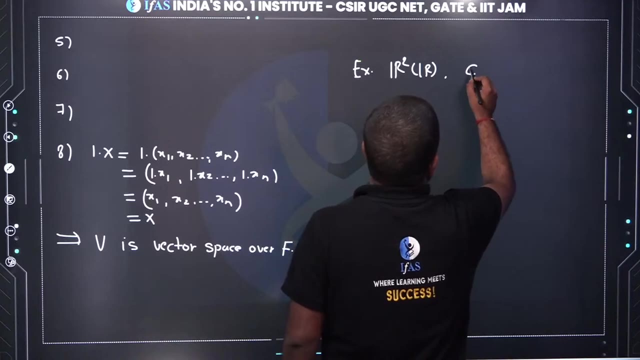 For example, what am I saying? Take R2 over R, The operation is the same. I am keeping vector addition and scalar multiplication the same. Take R2 over R. Or take C3 over C. Or you can say ZP raised to N over ZP. 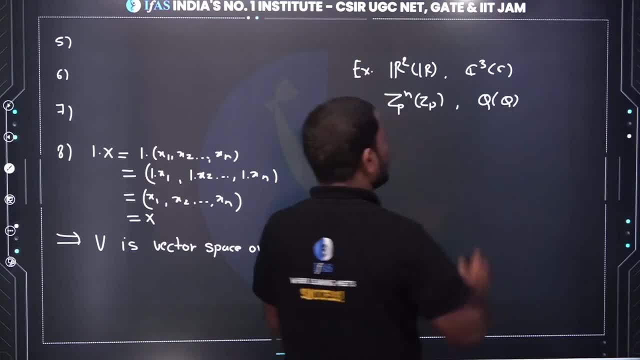 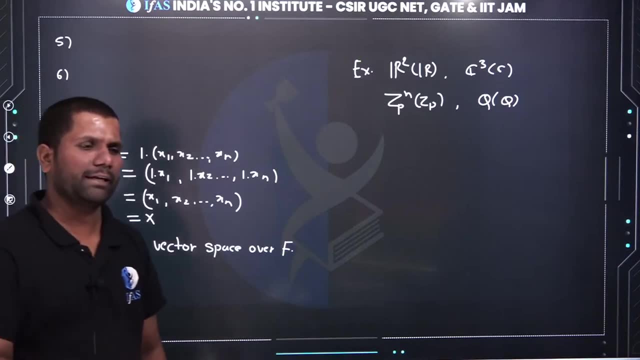 Or take Q over Q. All of these with respect to that operation. it is vector space. Keep any value of N, keep any value of field. So what will we always form? We will form vector space. This means you have infinite number of examples for vector space. 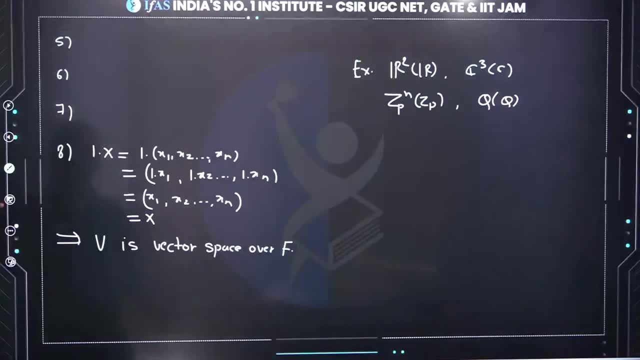 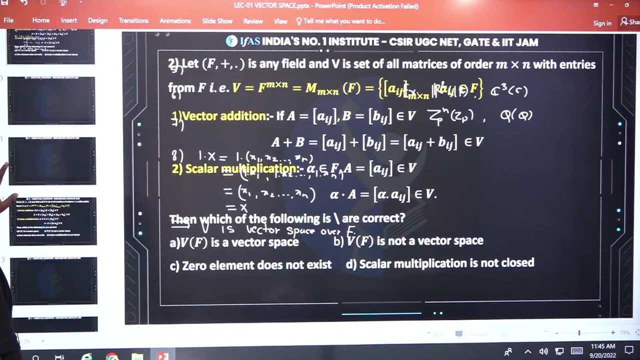 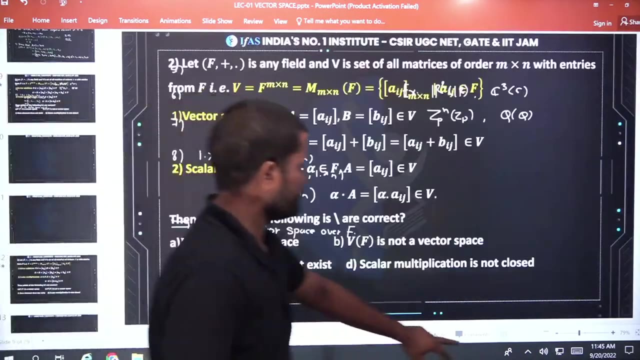 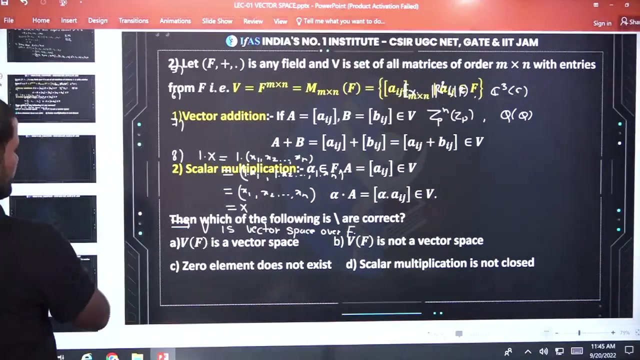 Is it clear? See till here. Okay, I hope you have understood till here. Okay, I hope you have understood till here. See, if anyone has any doubt, you can ask. Okay, All the students are clear. till here. See once. 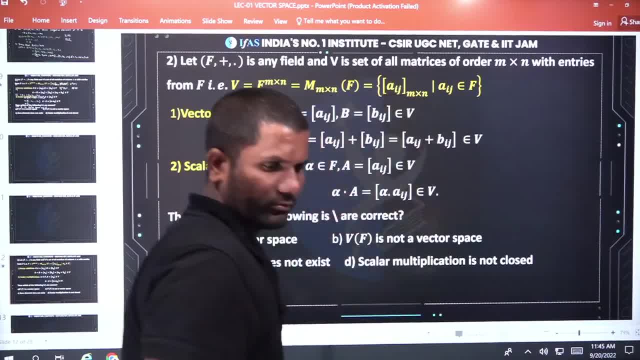 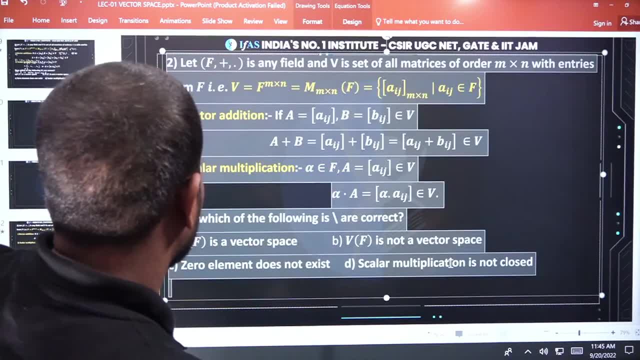 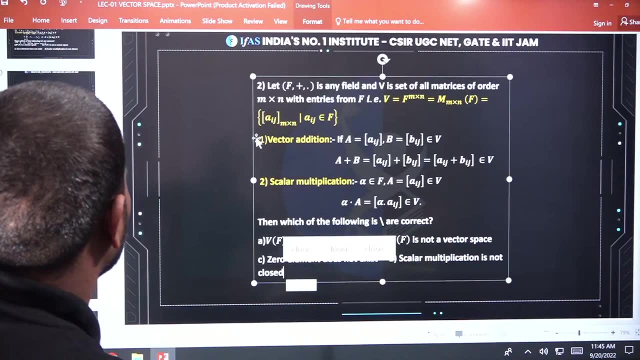 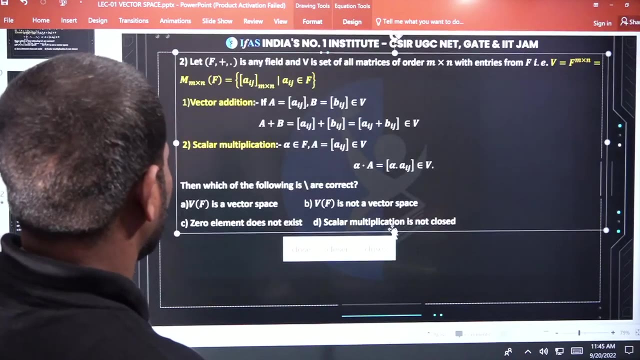 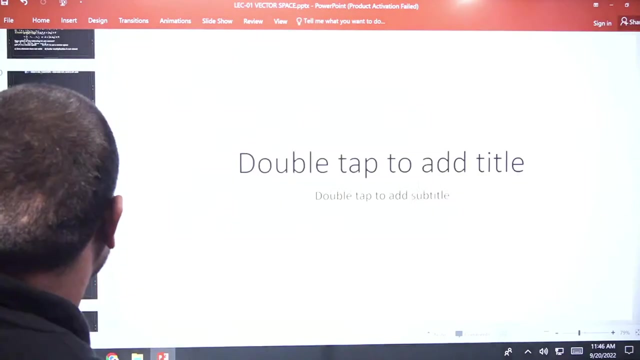 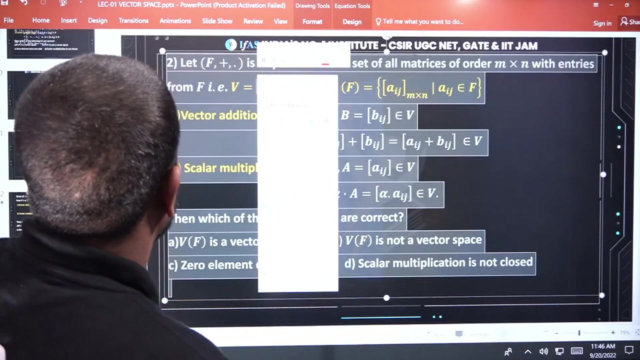 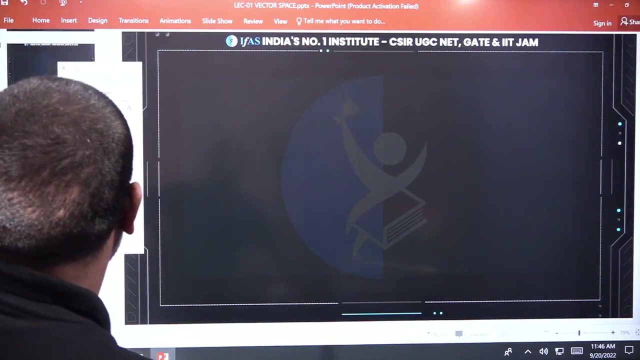 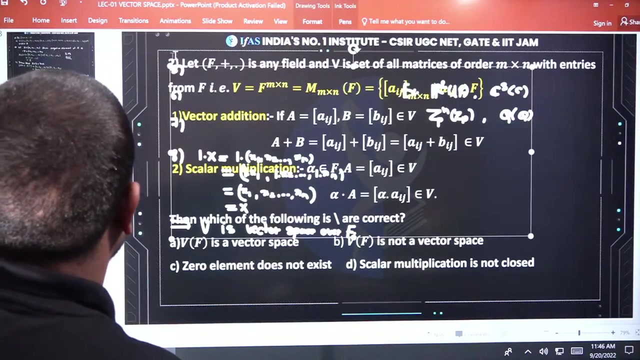 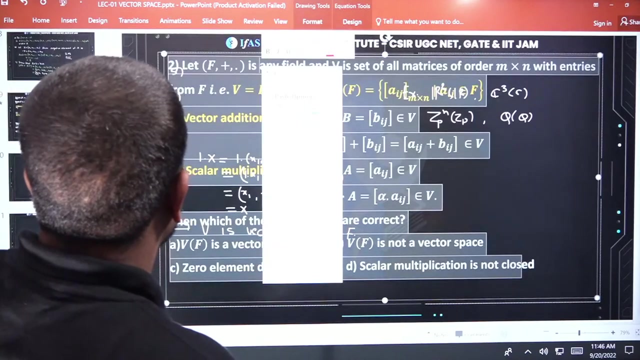 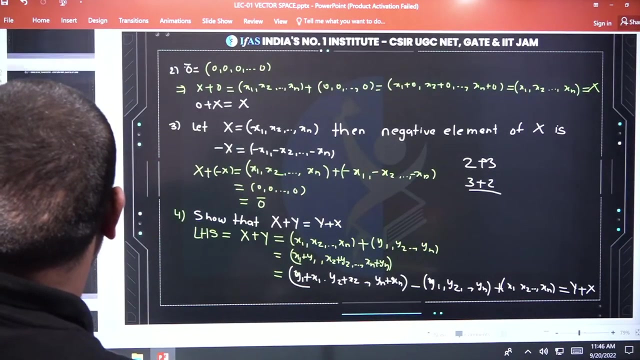 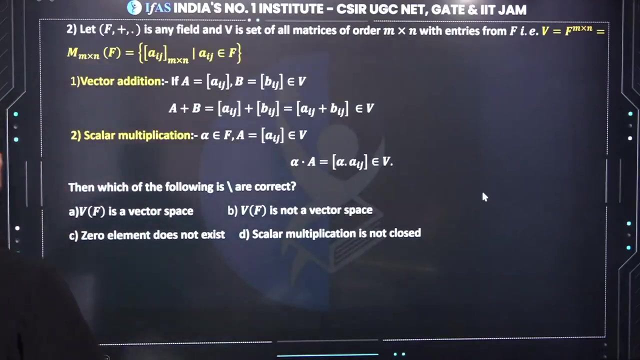 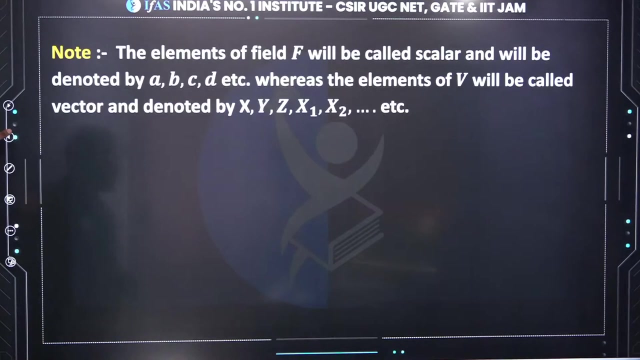 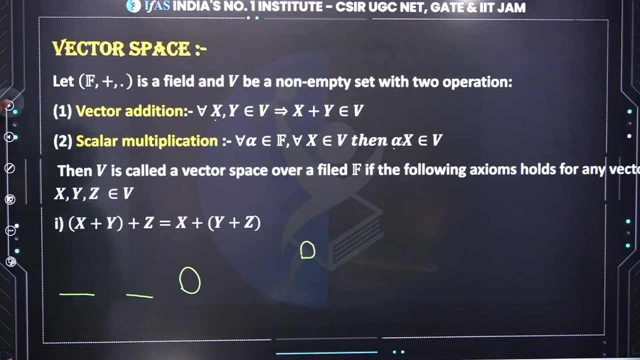 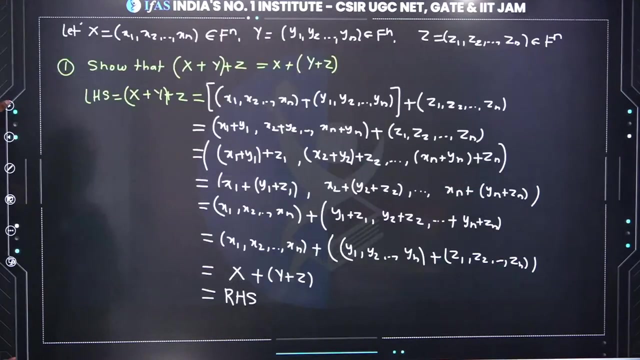 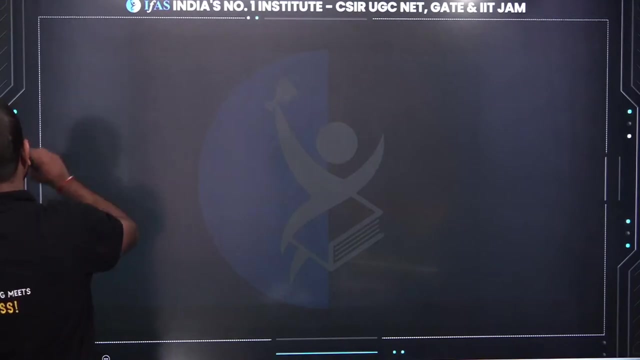 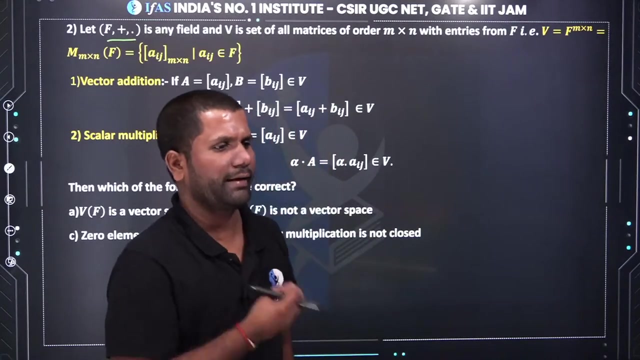 You guys, Go ahead, you. I hope you have been cleared up to here. then we will move on to the next slide. now, here we will see the example of a separate vector space. now, see here. let's move towards the next example. now, what is given to you next? see here what is given to you. there is a field, there is a field. see here. there is a field. and what did you take in V? you took all the matrices in V, set of all n cross n matrices. so what did we take here? V is a set of all n cross n matrices, which is also 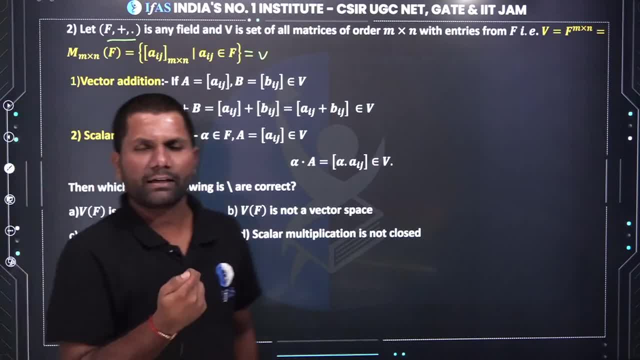 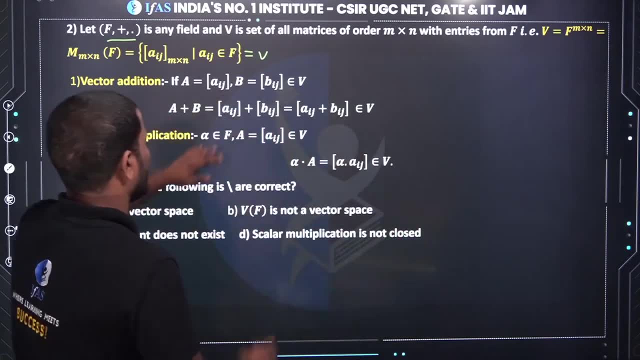 represented by your symbol. now see how to add the matrix. you know who you are. how are you going to add the matrix to the bench? add the same way. add the matrix as a component. what toca card? what you did from childhood? 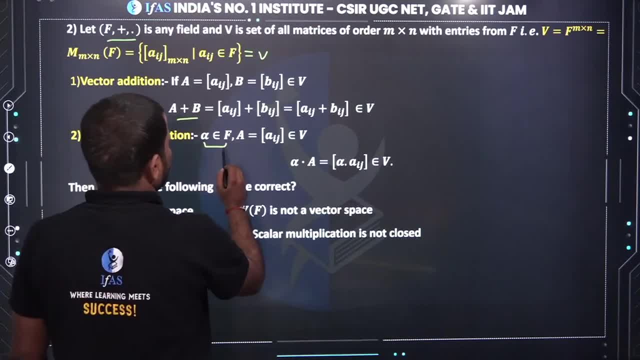 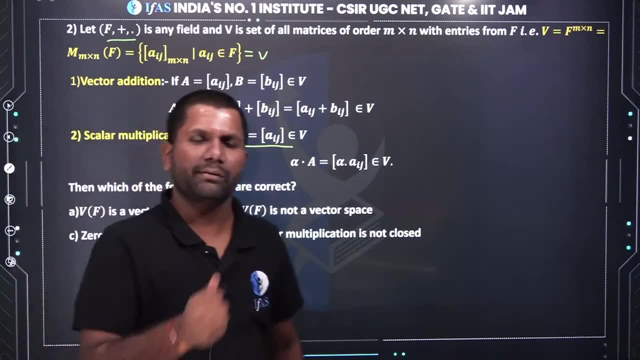 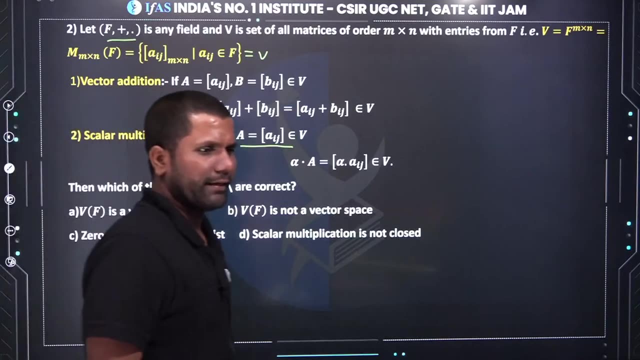 same addition and from childhood, this color multiplication is How to multiply by this color in the matrix. that same color multiplication is being given here. so you have to tell which will be correct among these. tell the matrix take care of this. tell there which. 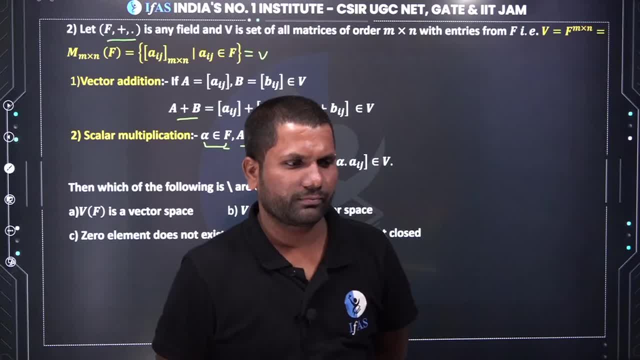 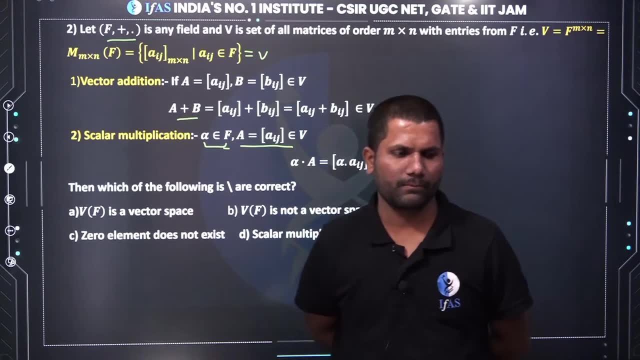 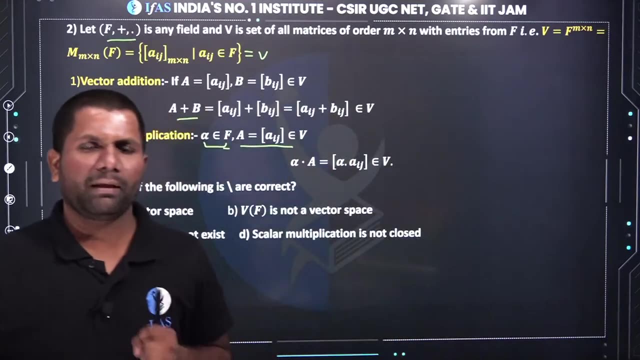 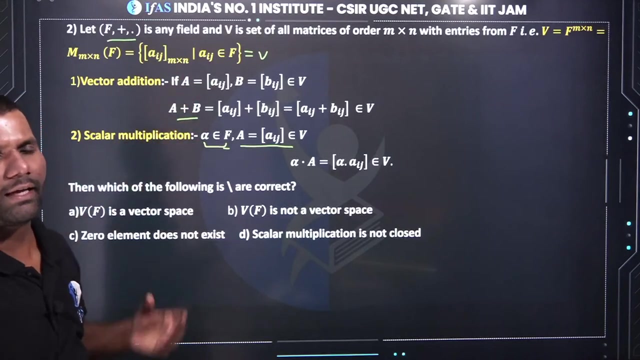 answer can be correct in this matter, guys, you see, is See all the students, See what we did in the first example: fn over f is a vector space. Now what we are taking in the second. First was n- tuples. Now what we took. here We are looking at the vector space of matrix. 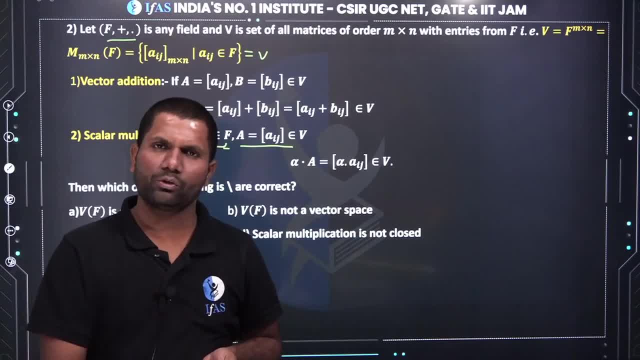 See the equations that come in the exam. Either they are of tuples Or they are of matrix. Either it will be function or polynomial. You remember these 4-5 types So that if there is a question of vector space in the exam Then you do not have to check 10-10 properties. 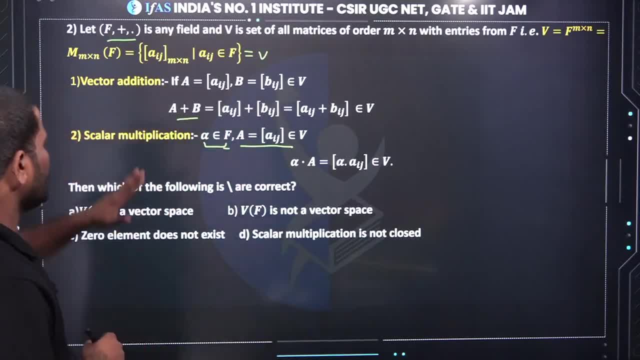 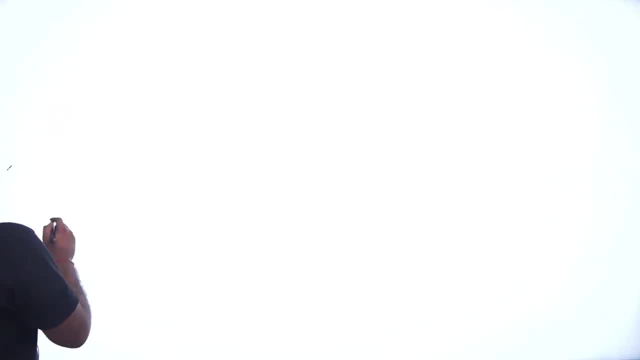 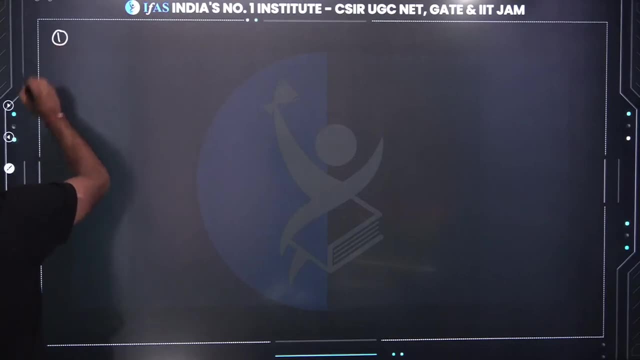 You can easily verify it Now. let's go Now tell me some special things here. First thing: Here addition will be associative. This is clear. See, here, Here the addition will be What will be your addition? First property, If you see, first, Vector addition is closed. What is vector addition closed? 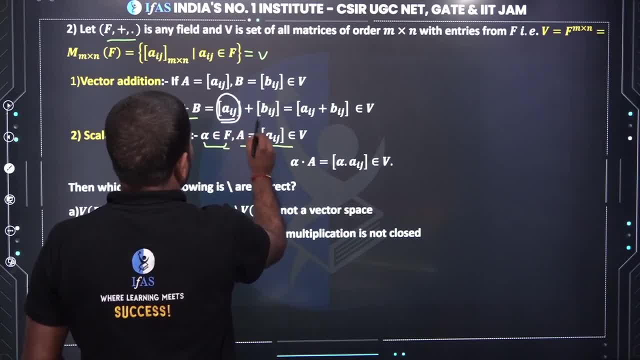 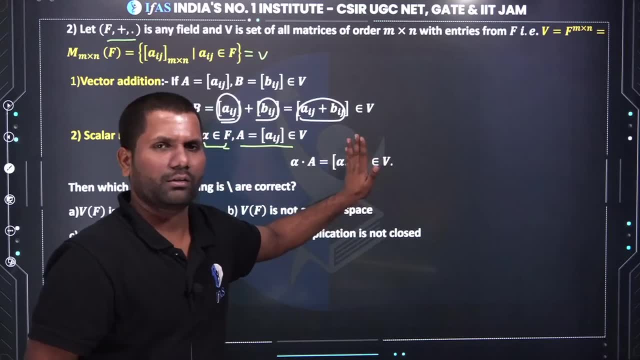 Like two numbers We took from any field- A is also from any field- After adding Will go in the same field. Vector addition and scalar multiplication Are clearly closed here. Ok, There is no problem in this. Now let's move forward. See What do you have to do in the first property. 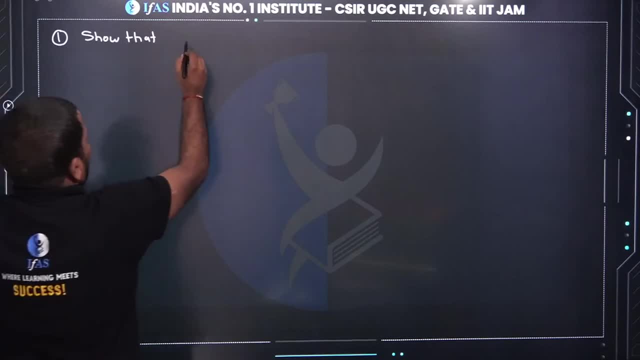 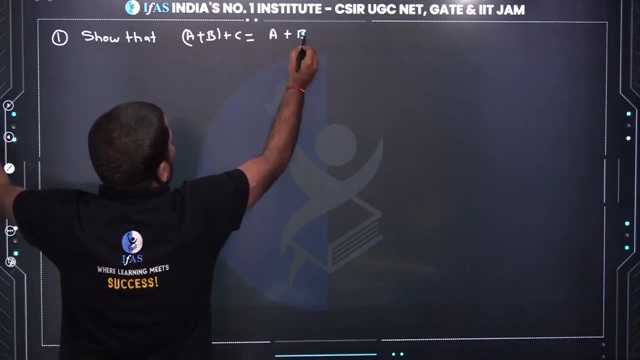 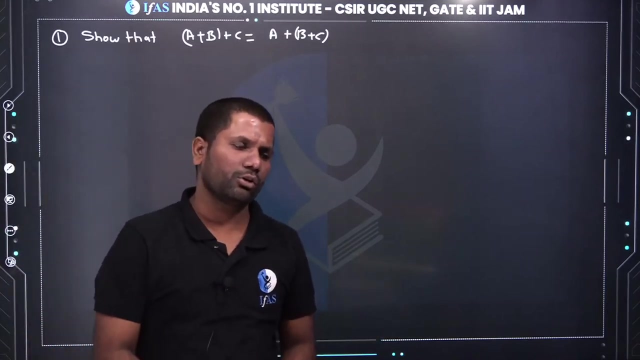 So that Take 3 matrix You have to tell a plus b plus c is same as a plus b plus c Means first add these two matrix, Then add with c. Or add the last two matrix, Then add with first. In both cases Tell you the result: Same. 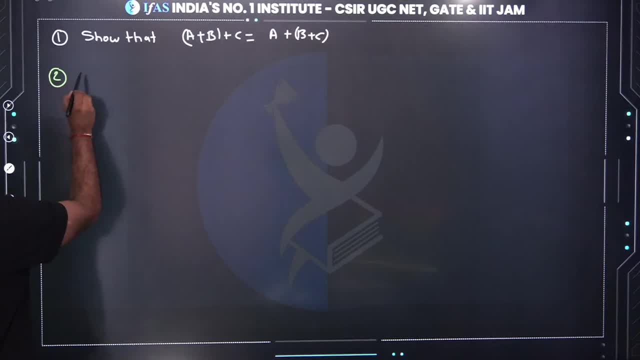 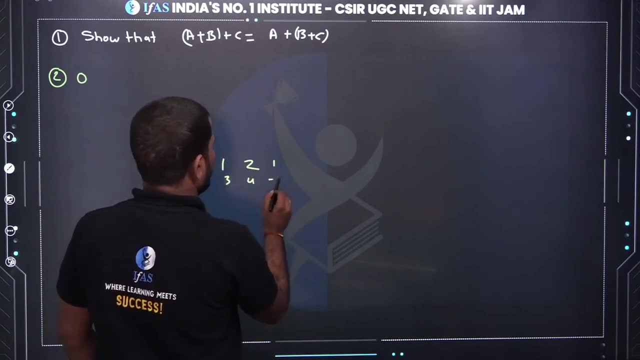 This is homework for you. Second property: See here Here: zero vector. Now I am giving some matrix. Suppose I have given a matrix Like one, two, three, four, One minus one. Now with whom should I add this So that I get this matrix? I add it with zero See. 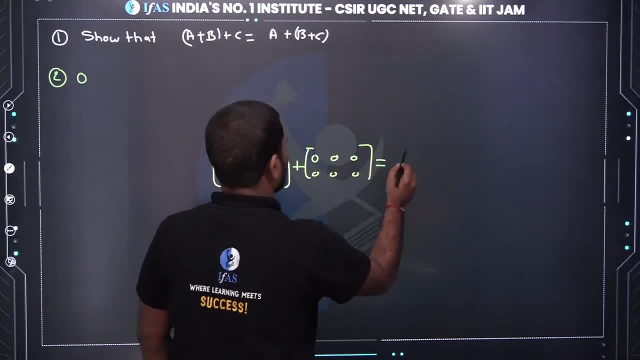 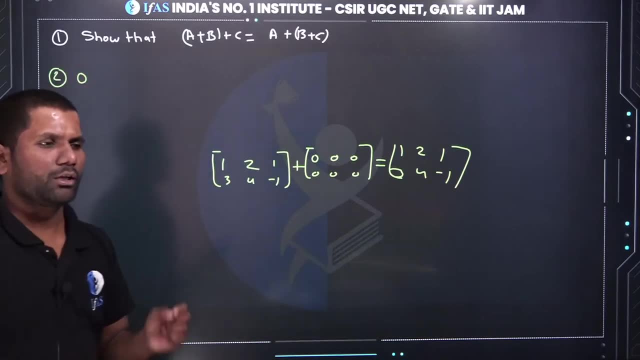 With this. With this I am adding. So what am I getting? This is the matrix One, two, one, three, four and minus one. So here you can see That in matrix. What do you get? zero vector In matrix. you will get zero vector, Zero matrix. Ok, So what can you tell here? 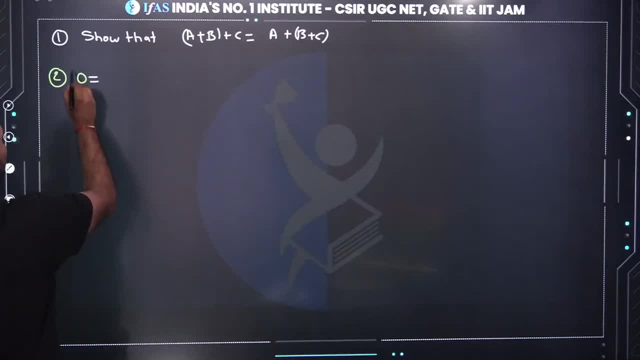 So what will be your zero vector, Zero matrix, So you can tell zero vector, Zero, zero, zero, zero, zero, zero, And so on. Remember, Its order will be the same. What will be the order of the matrix? Suppose its order. What have we taken? We have taken m cross n. 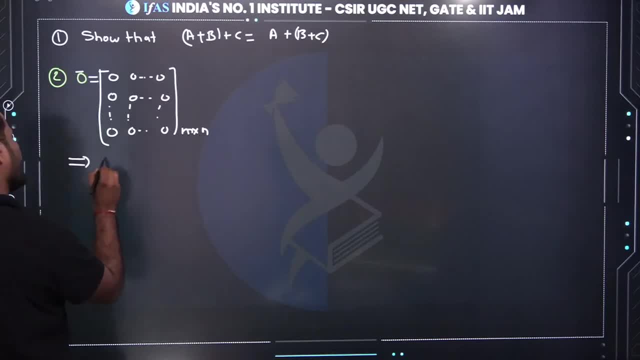 Ok. So in this case You can see A. Whether you add with zero vector, Add from left Or add from right, You will always get A. So in this case, What will be your zero vector? So here you can verify easily That your zero vector Will be zero matrix. 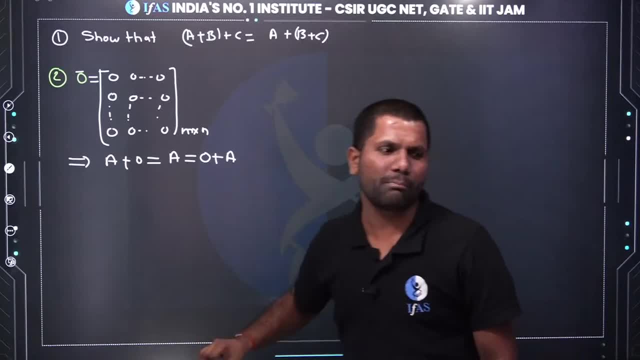 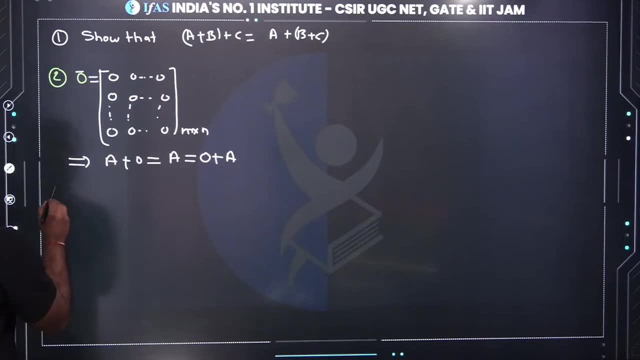 Ok, Yes, You can say null matrix Or zero matrix. Now we move ahead. Third property. So here you can see What will be your zero vector, Zero matrix, Third property. See in third property What you have to tell Negative element. Suppose We have taken A, Where does A belongs? 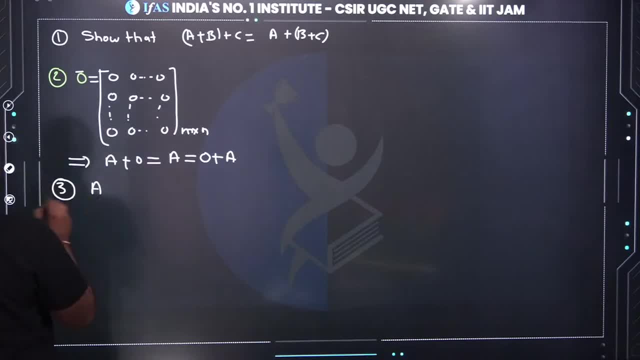 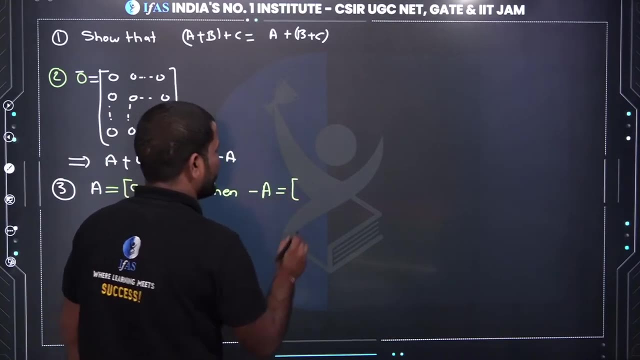 Suppose Let's write this: A is equal to What have we taken? A is equal to A, ij, A, ij And order is m cross n. So in that case Then Negative element, That is Minus A. What will you get? Minus A Is equal to Minus of A- ij. 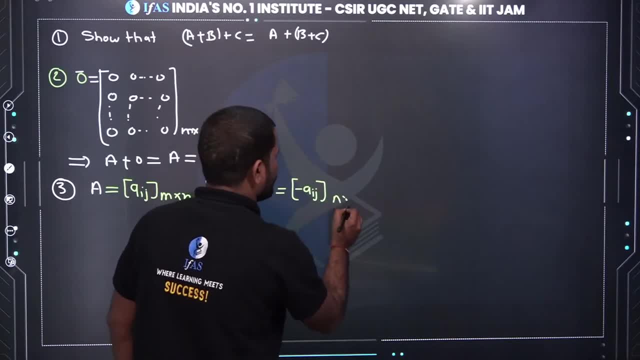 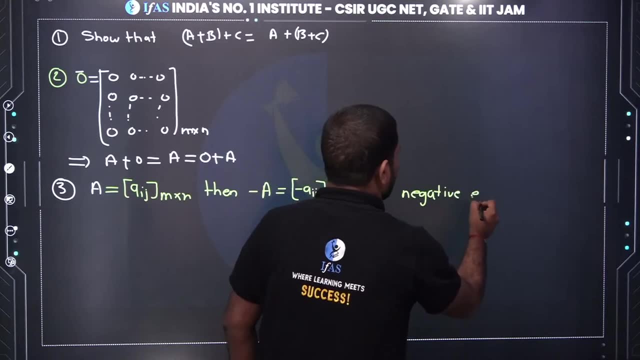 Minus of A, ij, n, cross, n Is Negative element- Ok. Negative element of A. What did you get? You will get its Negative element. Negative element of A: Ok, What will you get? You will get its Negative element. Negative element means, If you see this matrix, Matrix A. 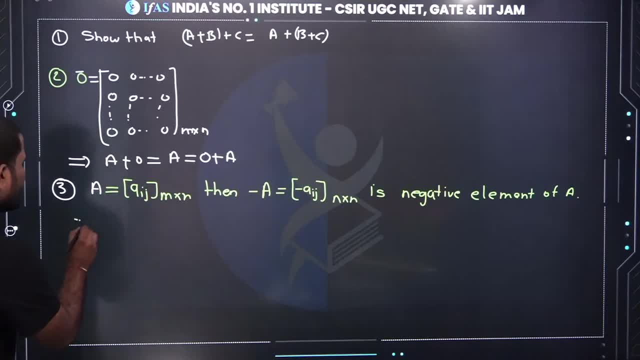 Plus, Minus of A, What will you get? Zero matrix, Which is equal to Minus of A. Plus A Is zero matrix. So from here, What have you got? Commute, There is also Zero vector. There is also Zero vector. There is also Negative element: There is also zero vector. 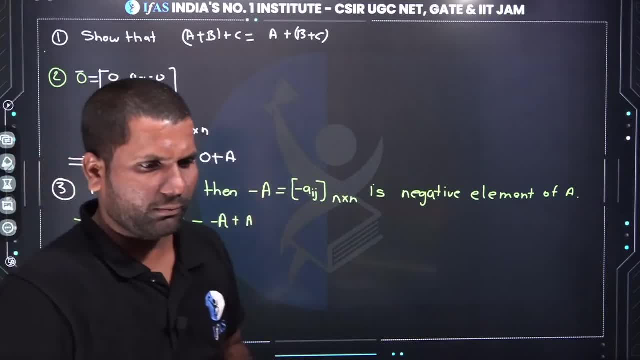 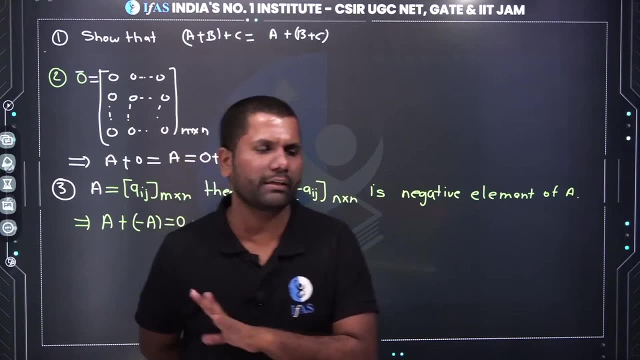 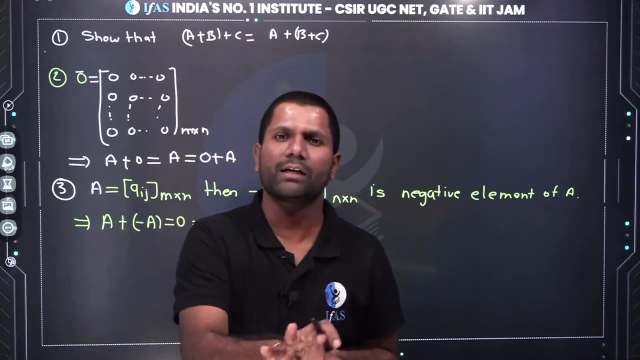 It also has identity. Ok, Yes, The order of the matrix. Anything can be. Yes, Matrix, Take a square Or take anything, No problem, Take any matrix. There is no condition On this order. When we read Subspace, Then We will put some conditions There. In the next session We will see. 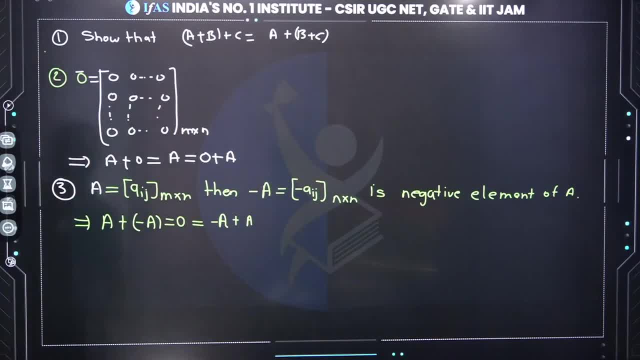 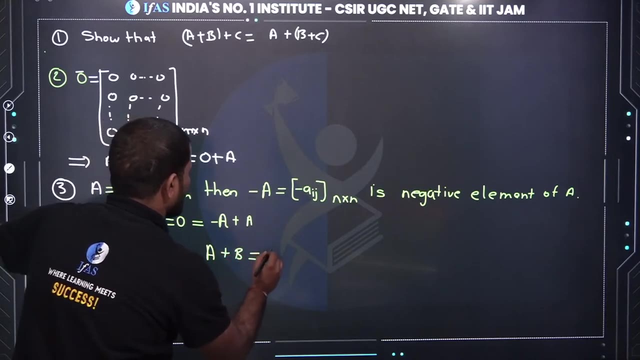 When we do Subspace. So here, See It gave you. Ok. In the same way, What can you do? You can check the fourth property. What is the fourth property? Fourth property: You have been given That A Plus B, If you see A plus B, B plus A. So here, 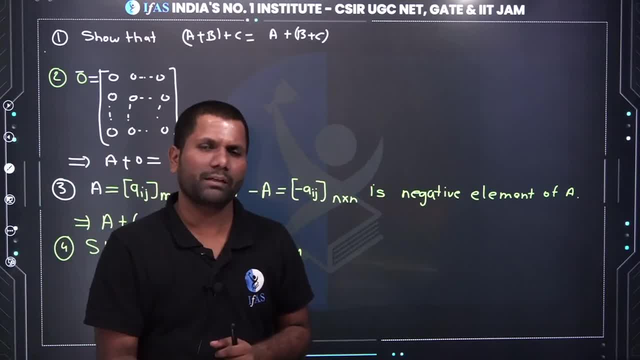 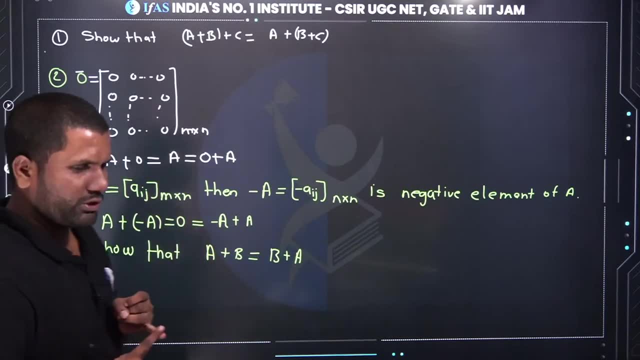 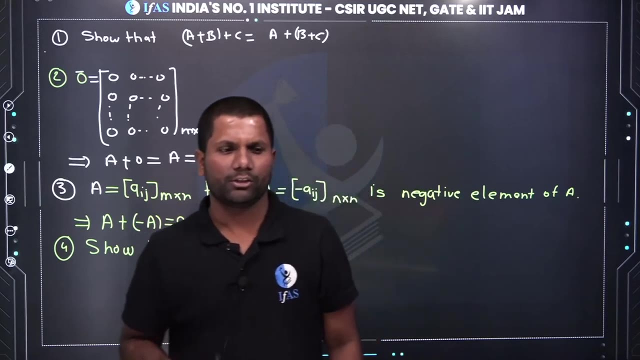 Fourth property: First you Two matrix, Whether first Do A plus B Or B plus A, Matrix addition Commutative. This property You can verify easily. Actually, Tell me here Some examples I am doing. Which is vector space? Just you Zero vectors. What are zero vectors? Negative elements: If N is given. 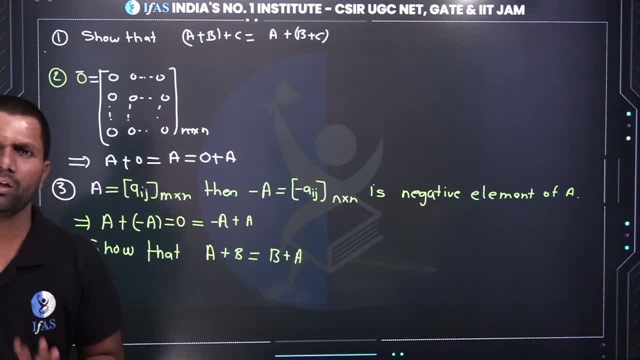 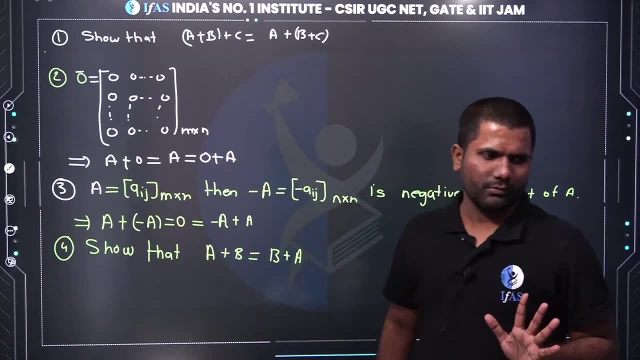 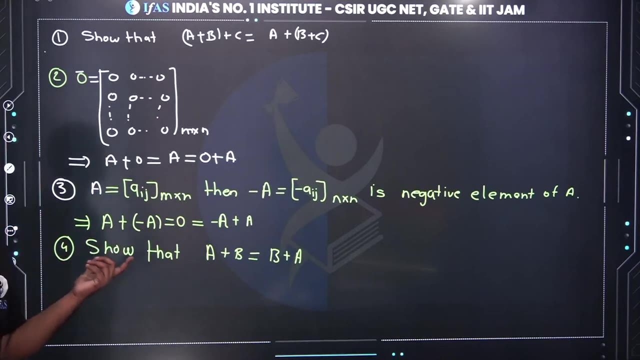 Then what is zero vector Zero, zero, zero, N times? If there is matrix, Then what will be zero vector Zero? matrix Will be: Ok, It is clear up to here, See everyone. Once all students See this. Clear up to here, I hope. Ok Now, similarly, Other properties You can easily verify. 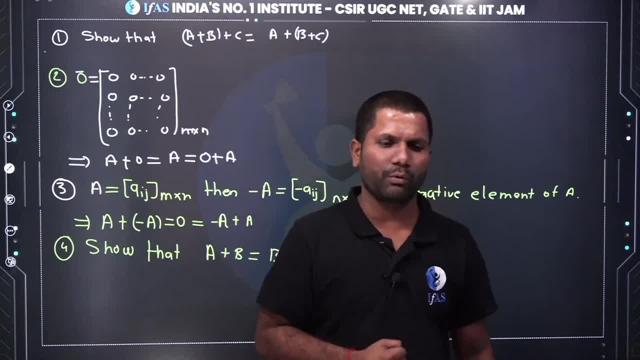 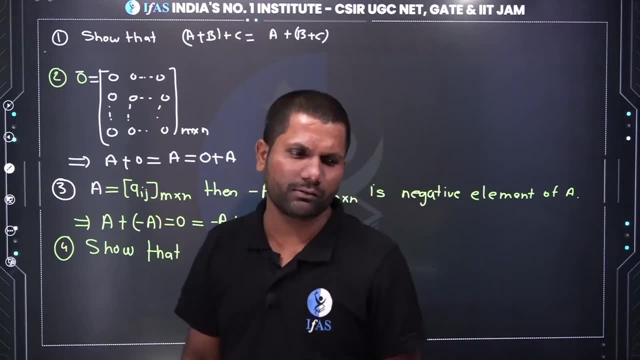 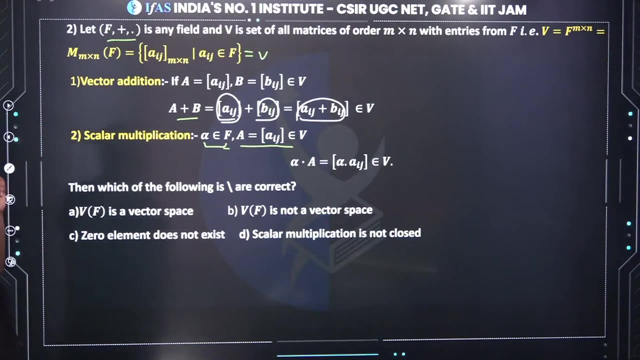 Other properties For you. Homework Here. What was more important? That you should know Negative elements, Identity. What I have told you here, Ok, See once, Clear up to here, So from here. If all properties Check once, So from here, What do you know? What will happen? This forms a vector space. 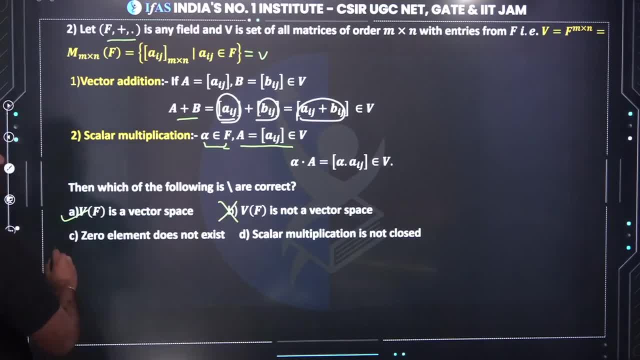 So this is a vector space. It is not a vector space. Zero element Does not exist, Zero vector It has. Will this multiplication fail? Will not. So from here You can say For this question What will be the first option. Will be correct. Clear up to here Everyone. If there is any doubt. 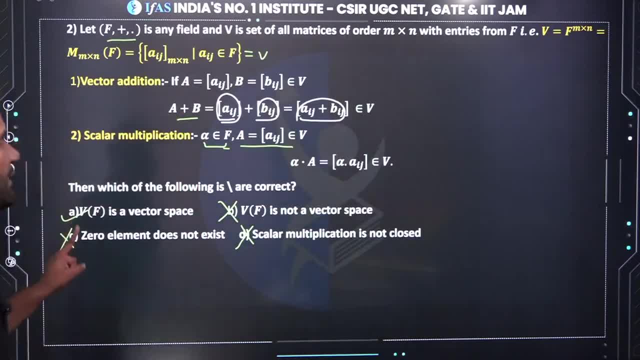 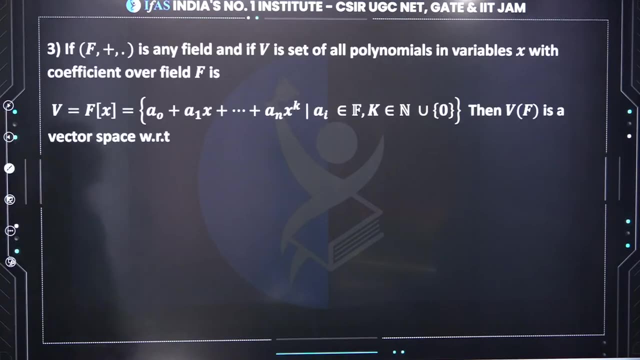 Then you can ask: Ok, So you have This. second example Came up Clear up to here. Similarly, We go ahead Now. third example: Here we have taken Polynomials. Third example: We see What are we taking. We are taking polynomials. So what is taken in polynomial? Suppose you first. 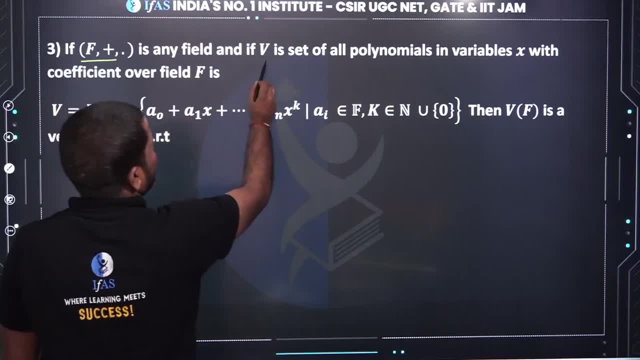 Take a field. What did you take? V is the set of all Polynomials. V is the set of all Polynomials In variable x. That coefficient is From field f. What comes in this Polynomials? How to see a0, a1x, n2, an x, raise to. 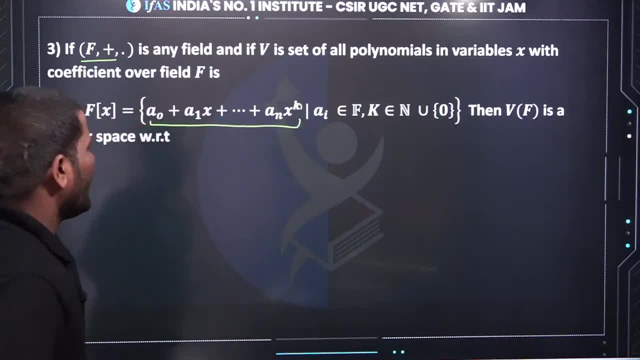 x raise to n. Do it here? x raise to n. Ok, Now what will this vector space Form Where you see, Two types of operations Are given. We need two operations for vector space. One is vector addition. Some threads have been given Vector addition. How to add two polynomials? 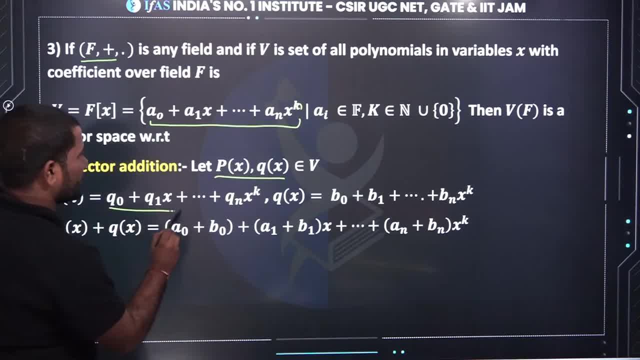 Suppose you took What, For example, a0, a1x, n, so on, up to a, n, x, raise to n. And what is this? b0, b1, n, so on, bn, x, raise to n, Took. So when you add it To add Means, Here the rule is given. 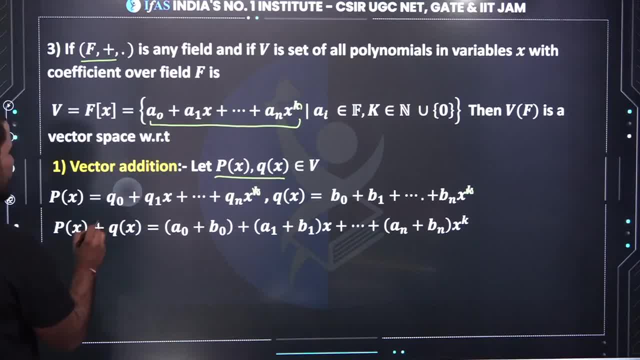 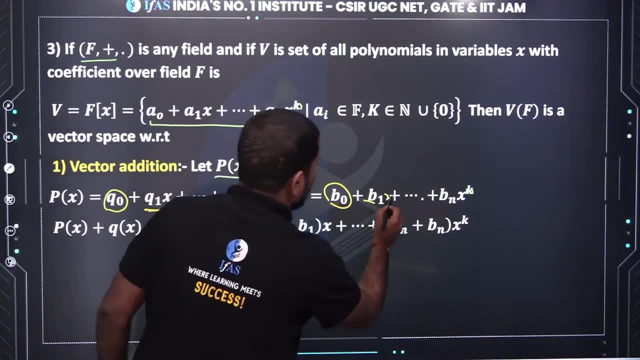 To add. To add: If you go to add, What do you have to do? Constant term of this And its constant term Together. Coefficient term of x: Together. Ok, Coefficient term of x: Together. Similarly, Coefficient term of x raise to n: Together. So here, In this way: 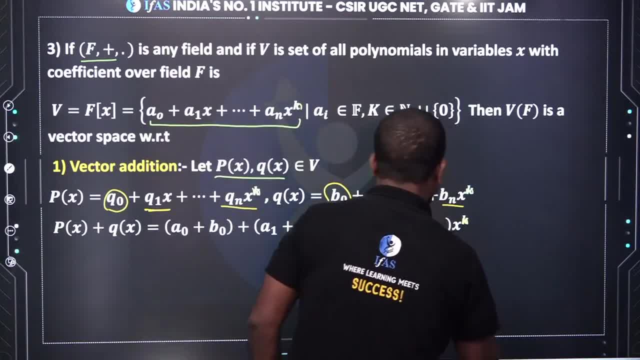 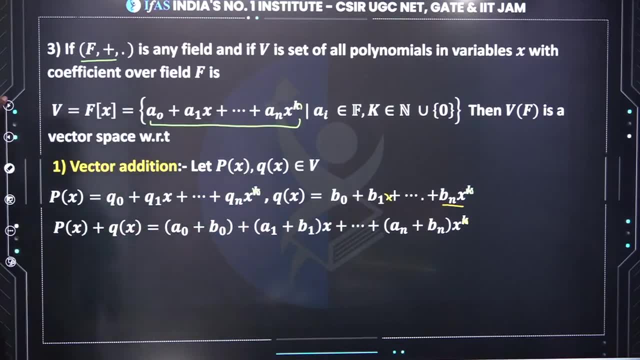 We have added here That you have got a, n, x, n. So in this way You have been given By defining vector addition. Ok, Vector addition. Second operation: You have been given Scalar multiplication. Yes, I will also give you Class PDF In the app I give You guys. Take it from there. 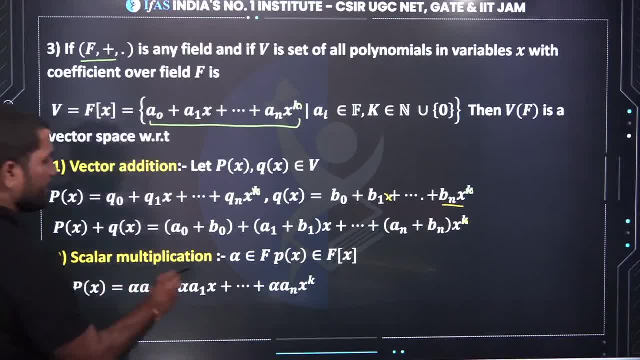 Ok, Now see What is the scalar multiplication, What has been given to you. Take any element From where Take, Take a polynomial. You took This alpha P of x, Which is Multiply with every term. In this way, You have been given Scalar multiplication. Here you have Vector addition And scalar multiplication. 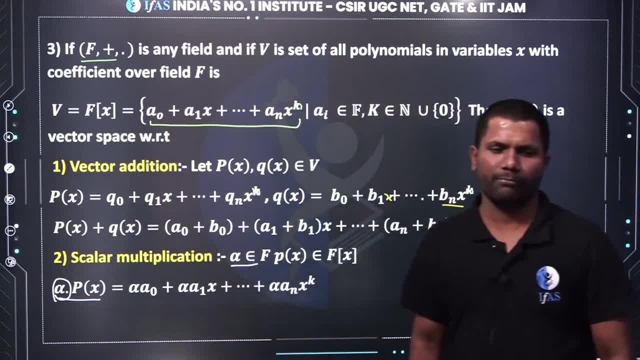 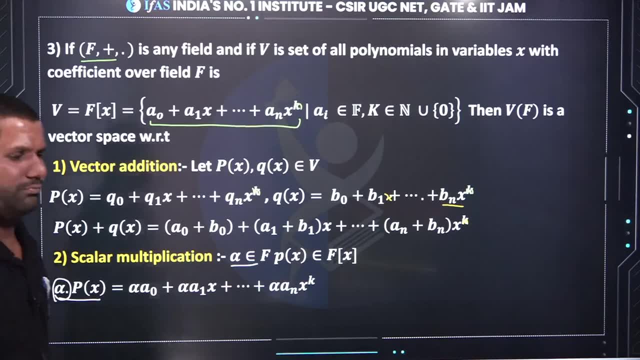 Now you have to tell: What will this vector space Form? What do you think You should form Vector space Or not? See once What will form Vector space Here? There are Four or five types. You have to remember it. If there are questions in the exam, Then it will be. 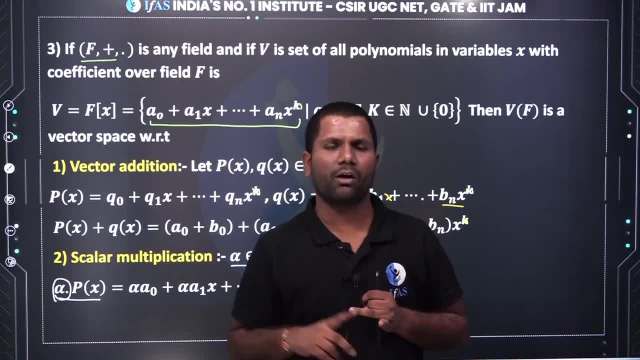 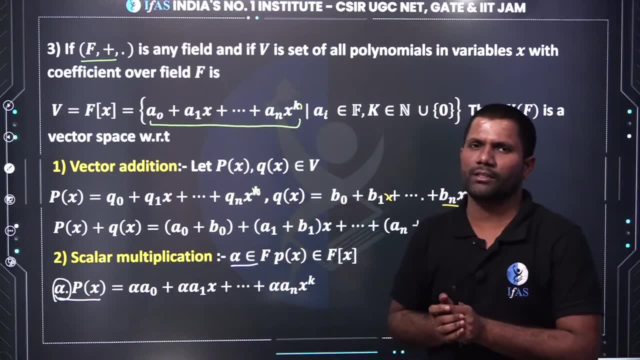 Of the same Four or five types, The operation Will be of the same type. The operation Will be your usual, Which we normally do In the same way. See When you have to add The polynomial. When no operation is given, Then you have to use For scalar multiplication. You have to use this: 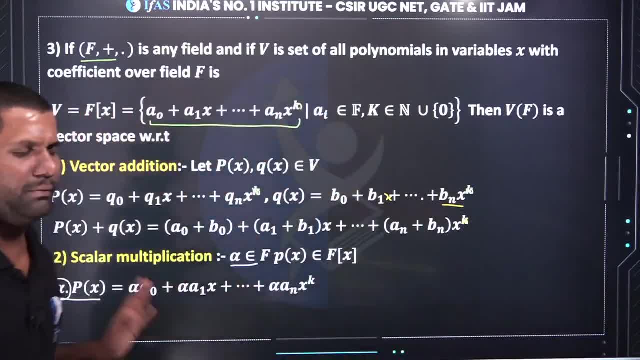 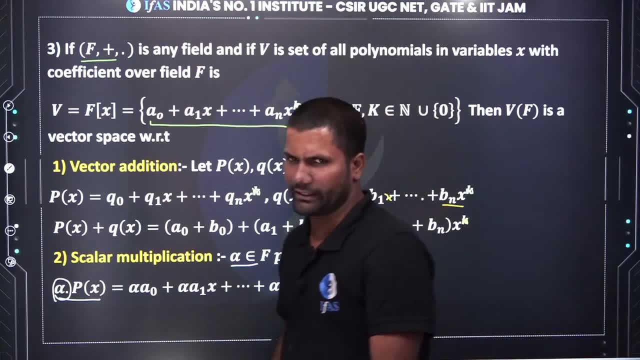 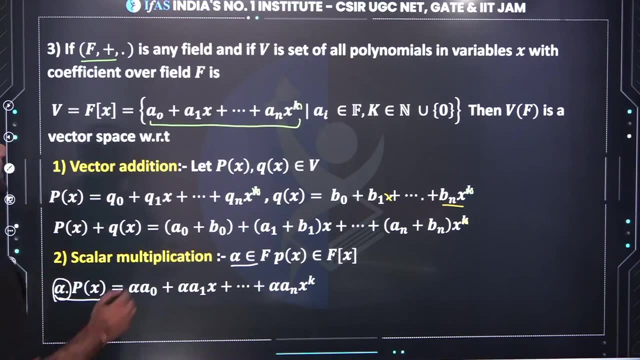 What will this vector space Form Tell? What will this vector space Form? Today We will see vector space. Tomorrow We will see all the space. So This vector space Will form. You have to keep in mind What will this always be? Vector space Means. This Means: Now You can keep the degree of the polynomial. 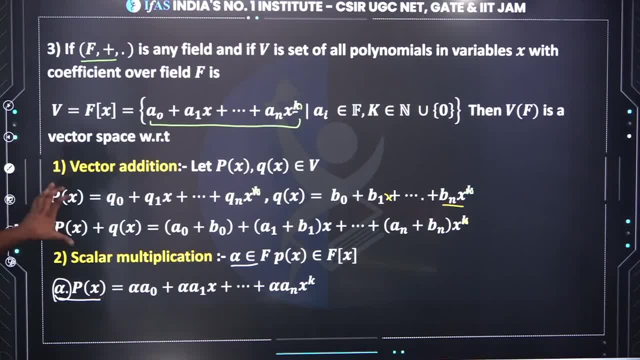 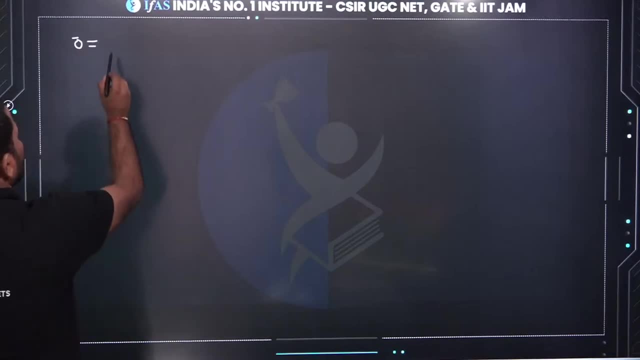 Anything, If you want, Keep anything. If this way Vector addition And scalar multiplication Is defined And given, So always That vector space Will form, Will do. Here You have to remember two things: This will always be vector space. What is? zero vector here? Zero vector Here, Zero polynomial, Which is 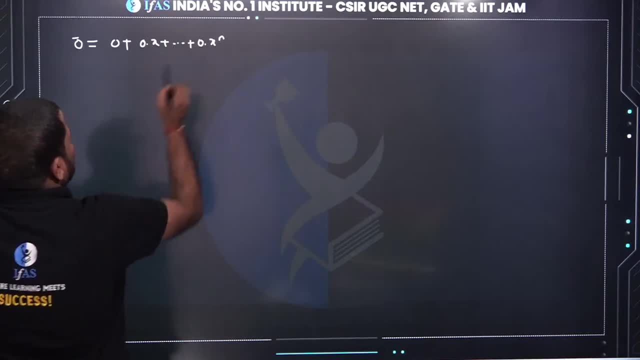 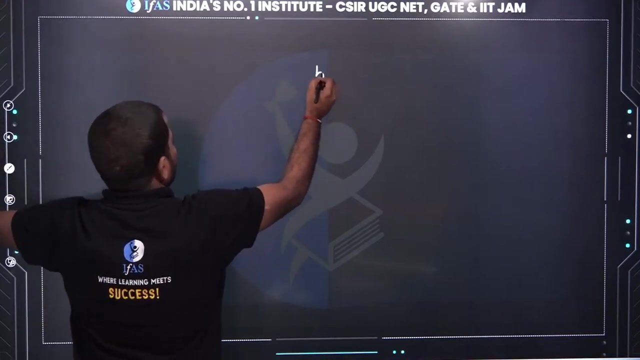 Zero, plus Zero into x, And so on. Plus zero into X, raise to n Zero. vector. What did you take? Let p of x? What did you take A naught? Plus A1, X And so on. Plus A n, X, raise to n Took. In that case, What will be its negative element? 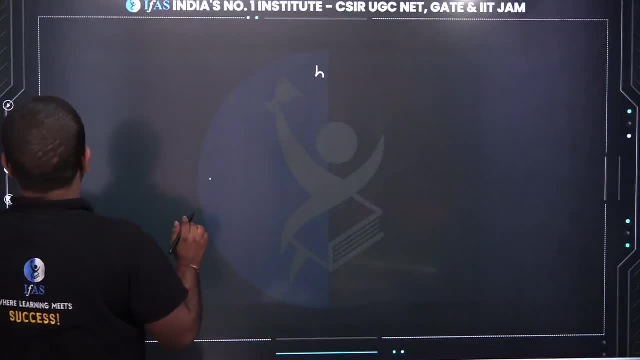 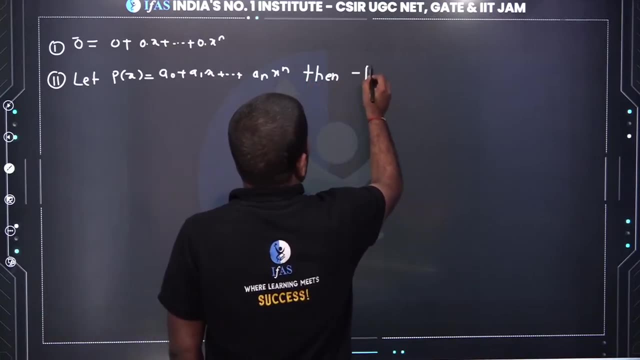 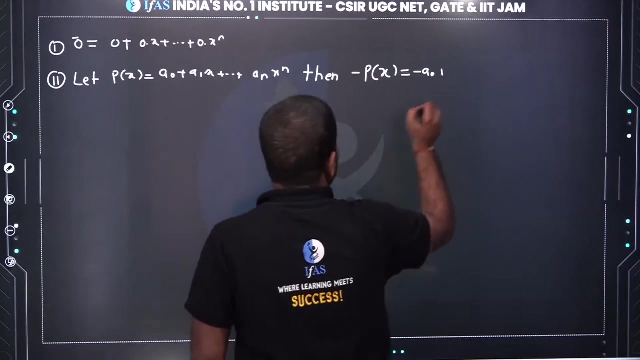 So In that case, If you see Negative element, What will you get here Then? Then What can you do here? Minus of Px, Minus of Px Means Minus a naught Plus, Minus, Minus, Minus, Minus, Minus, Minus A1 x. 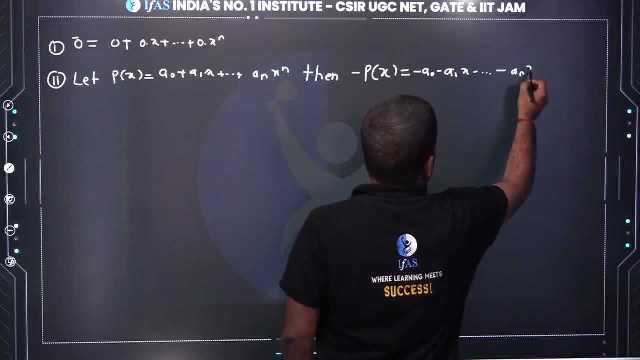 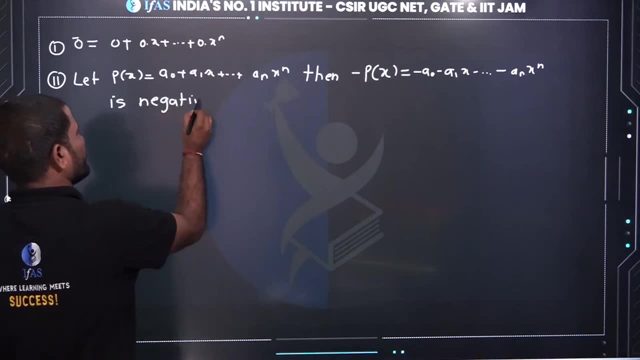 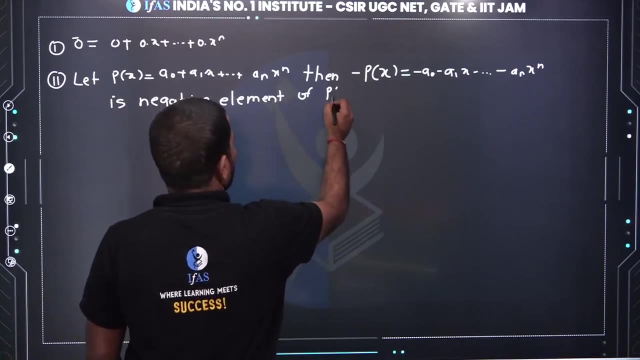 And so on. Minus A, n, X, raise to n. Is negative element. What did you get? Is negative element. Is negative, Is negative. Is negative element Of. Is negative element Of Is negative element Of, Its negative element Will be. So this is negative element Of p of x. 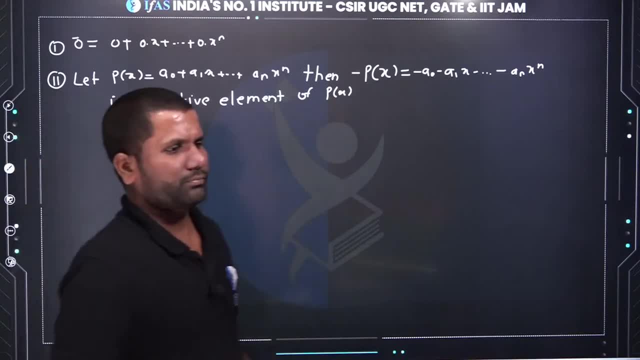 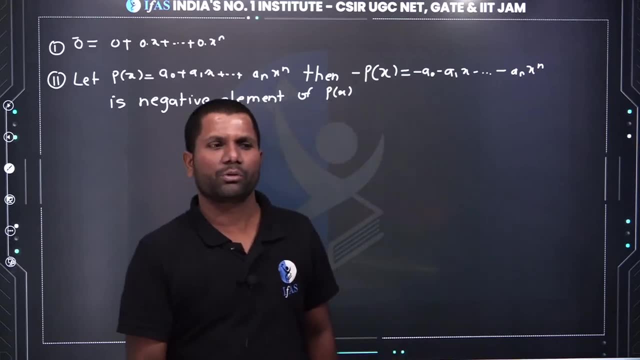 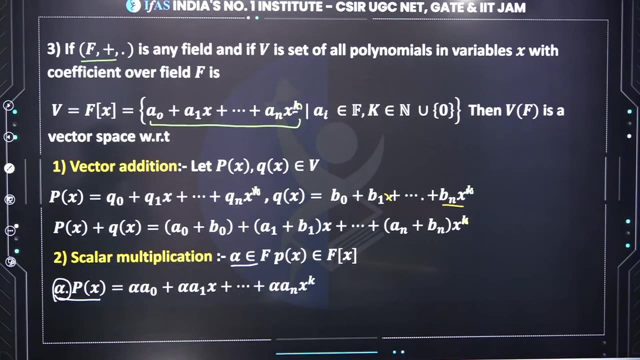 So here You have to keep in mind What will be its negative element And And this Identity And Identity, No, The Identity, And What will be the hotel, The Identity E What will happen, Which Will become Zero, And What will be the negative. What Will become Then? This Was. 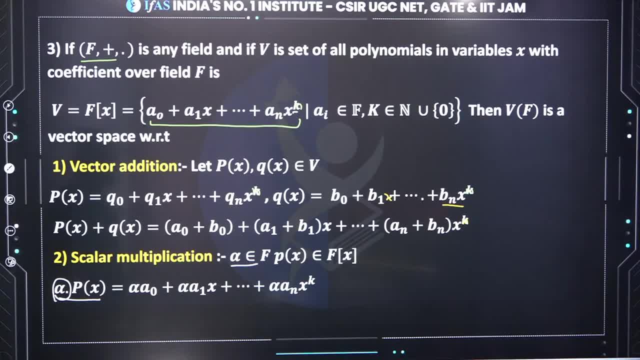 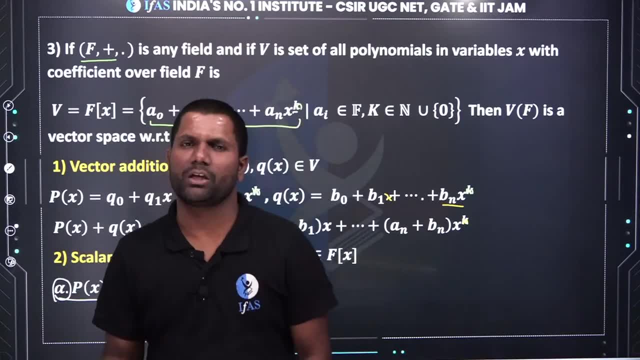 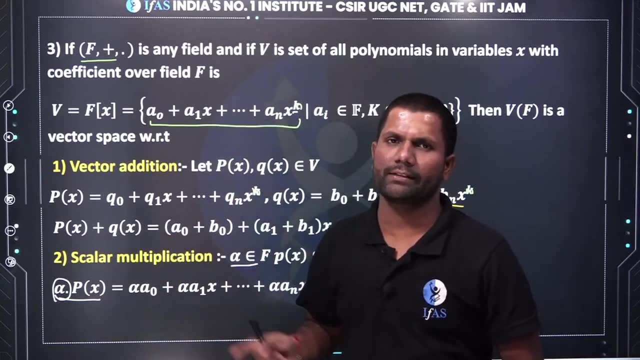 Hy right For Minus. So let's do this much in today's session. The three types of vector space we have done. you have to remember that We will do the remaining vector space and subspace in tomorrow's session. Just keep in mind that if this type of vector space is given, 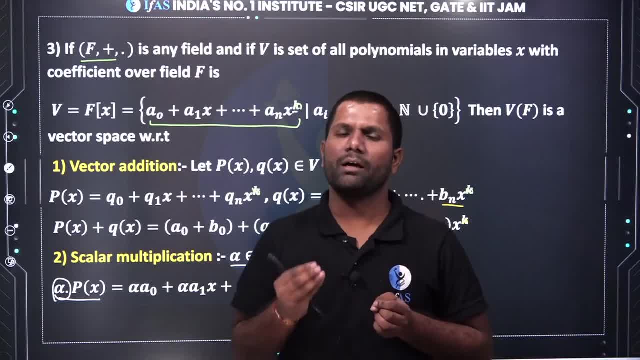 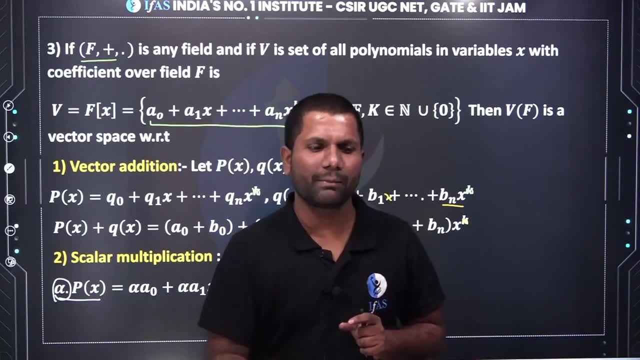 Then, whatever it is, whatever the value of n is, If vector addition and scalar multiplication is given, Then there will always be vector space. you have to remember So that if there is a question in the exam then you do not take time Look at it and tell me: hey, this polynomial addition is less than this one that we had read. 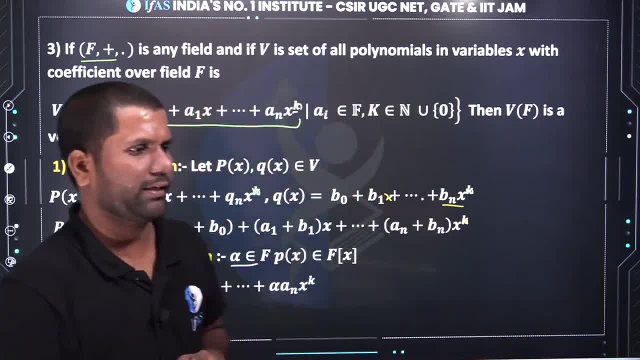 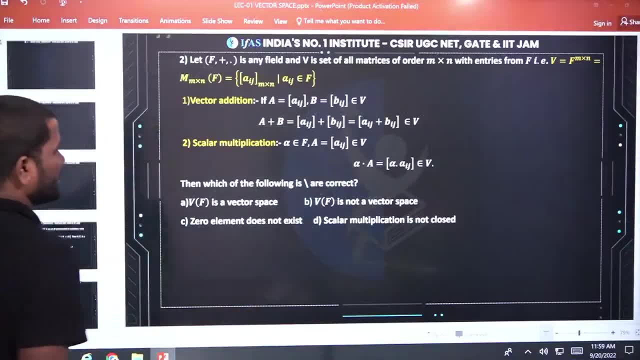 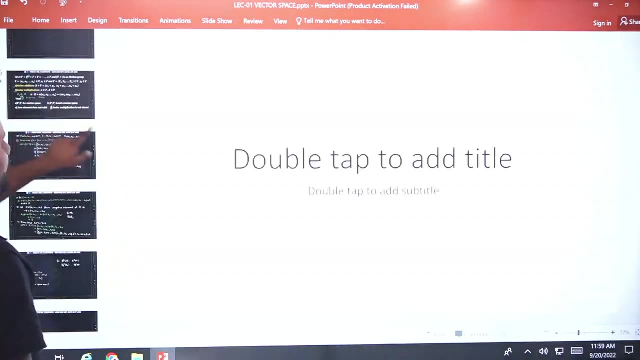 This will definitely happen. tell me easily, Remember all the zero vectors. What are the zero vectors of the first one, n tuples. If you talk about the zero vectors of n tuples, then see n tuples. what will be its zero vector? Its zero vector is 0, 0, 0,. you will get this. 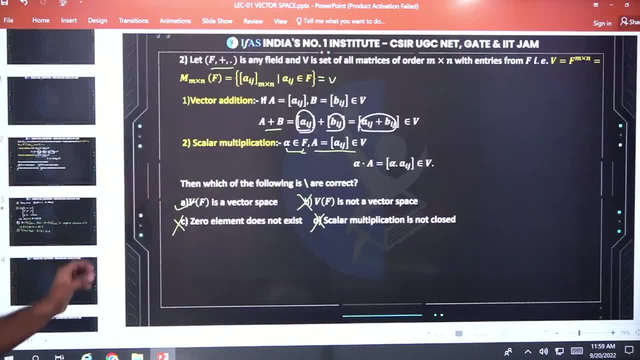 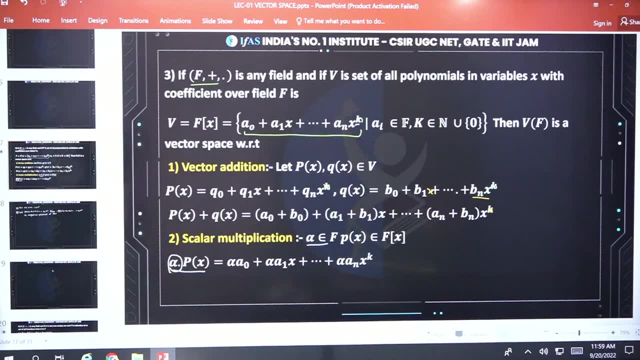 If you come to the matrix, what is the zero vector of the matrix? You will get the zero matrix of the zero vector of the matrix. Similarly, if you are asked what will you get the zero matrix of the polynomial Zero polynomial 0 plus 0 into x, 0 into x square, and so on, 0 into x raised to n. 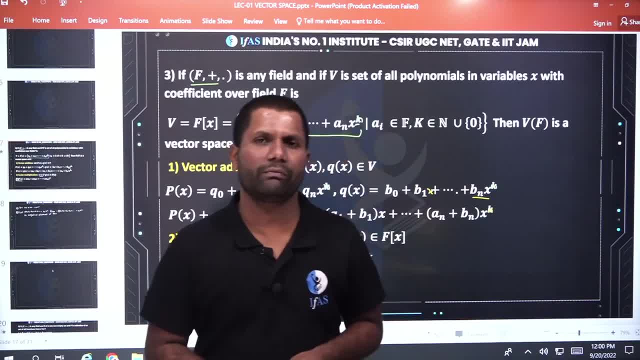 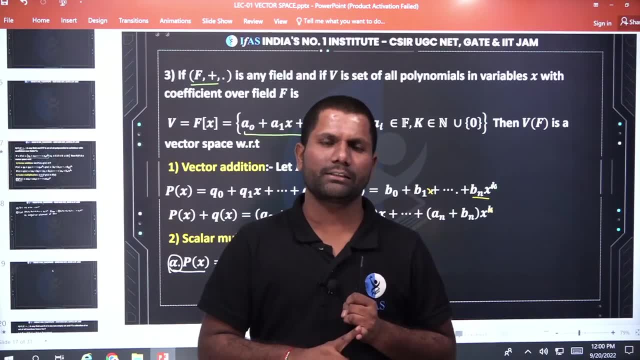 I will give you the PDF of this if you have registered yourself in the IFES app. If not, then register yourself. Where to register? go to the Mathematics CSI NET section and do it There. you will get this PDF. I will get it for you. 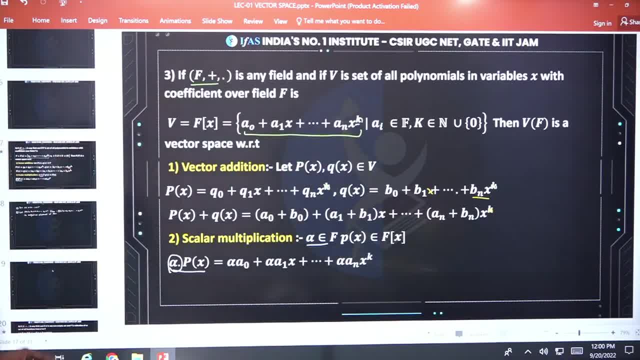 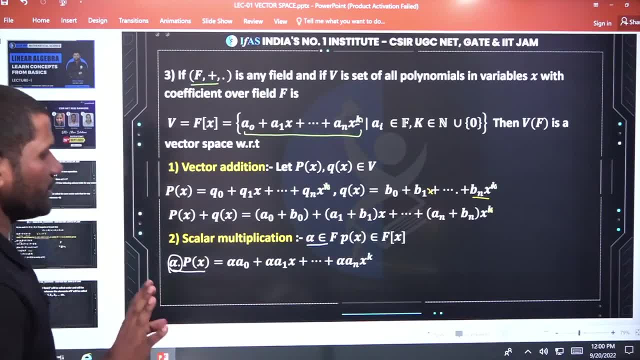 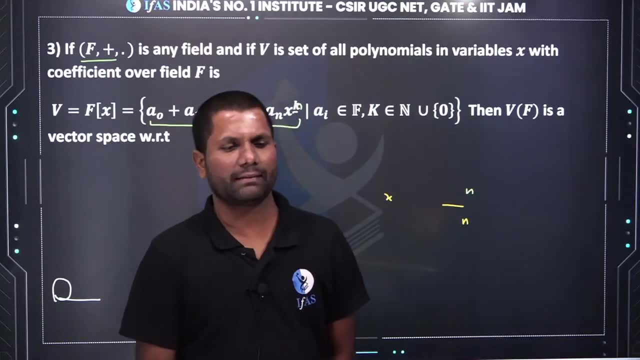 So that's all for today. There are some remaining examples of vector space and subspace. We will do it in tomorrow's session. There are five types of vector space. Just keep that in mind. So let's stop here for today. All of you stay with us. Thank you so much. 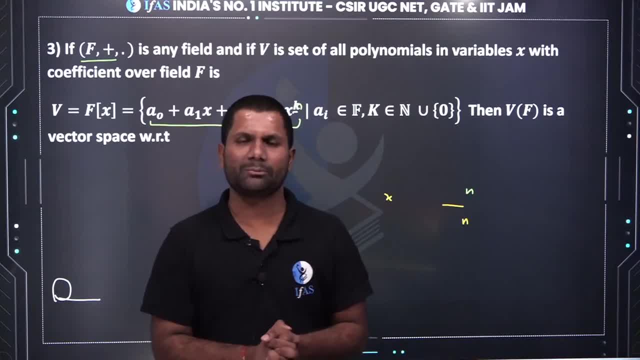 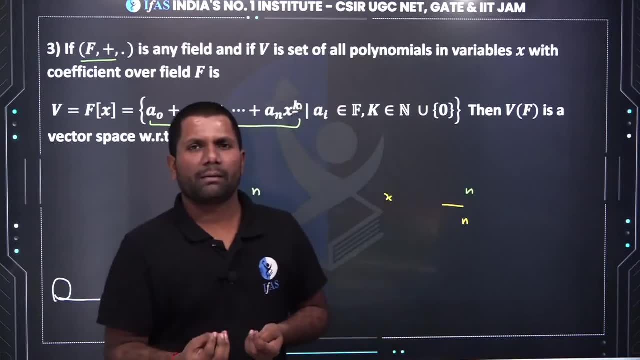 See you in tomorrow's session at 11 am, Where tomorrow we will read some more important things of vector space and subspace Means. our way of reading is this: If there is any question in the exam, If there is a question of vector space and subspace, 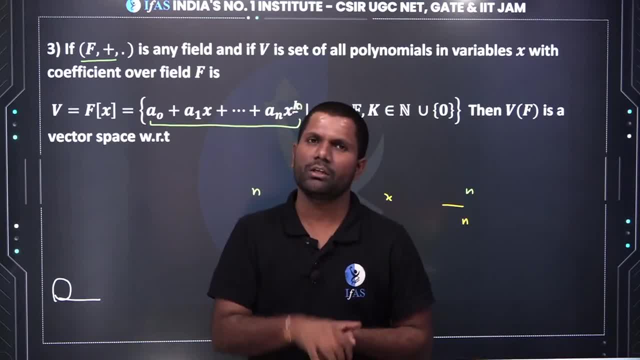 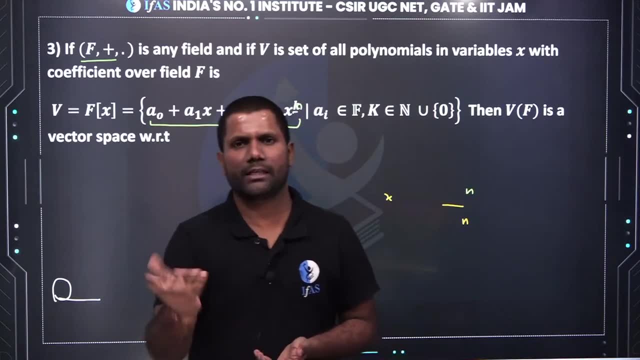 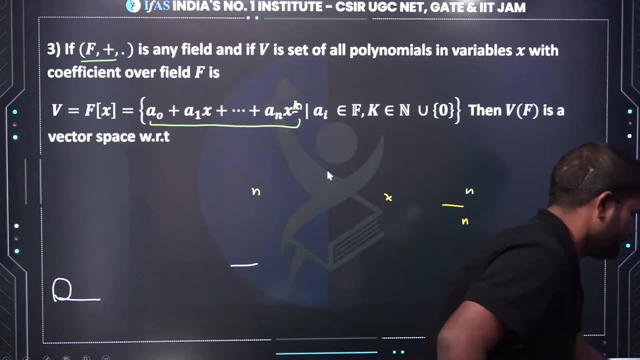 90% questions. Only you can see and tell Whether this is a vector space or not, Or whether it is a subspace or not, Means there is a 10% chance that you check it. Okay, So let's stop here for today. Thank you, see you tomorrow.